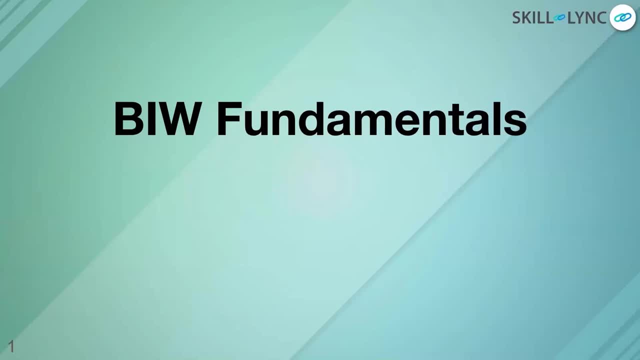 I just want to know, like, what kind of crowd we have it here is like all are from college or all are working for professional, or if somebody can help me out, Yeah, so, so, let's do this, Folks, if you can, in the chat box. 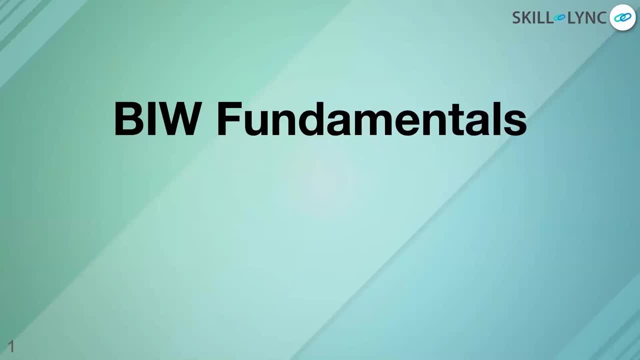 Let us know if you are either currently in your third, fourth year degree, first, second, third or fourth year in mechanical or automotive engineering, say, first year mechanical, second year mechanical. third year mechanical, fourth year mechanical. If not, if you are currently, 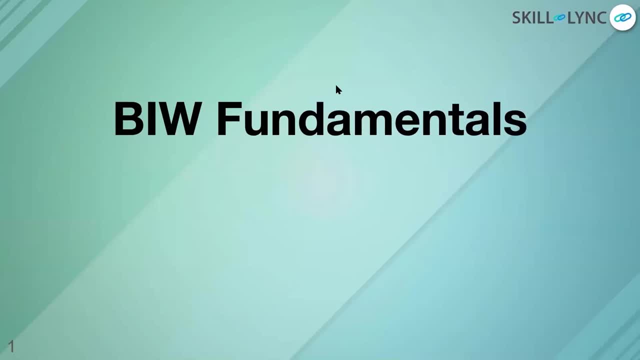 working in the industry, say two years experience design, three years experience automotive, Yeah. And if you're searching for a job, just say graduated, Great. So I have seen, I got my answer. It's like most of them are. 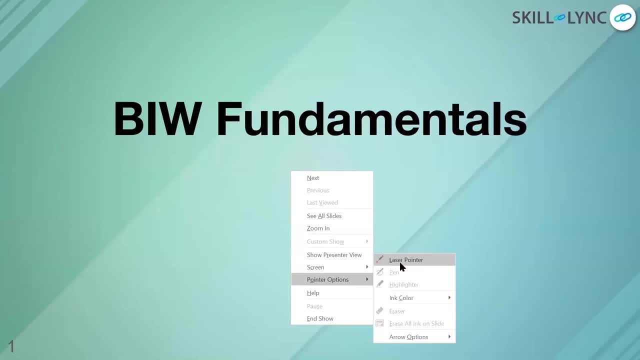 From college. Okay, So great, So perfect. What is your understanding, Like guys, is what's your understanding in BIW, when we call BIW, What is your understanding till date? I have to check chat every time. right Body in white: Yes, But what does that mean? Designing a? 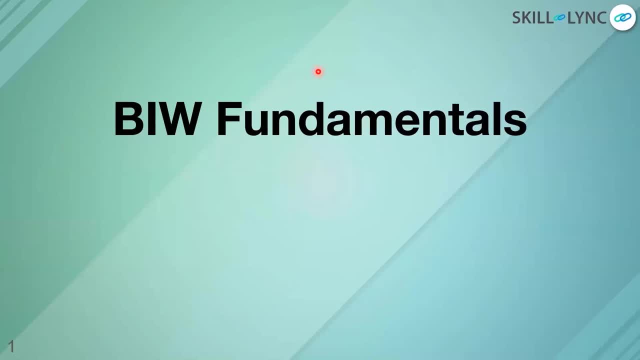 car. Okay, So I think we can't unmute people's right. Surya, Yes, Yes, Sumit, So there are so many people, Okay, It will kind of create a noise. Okay, Perfect, So okay, I believe the understanding of you is like all you, all of you, was having. 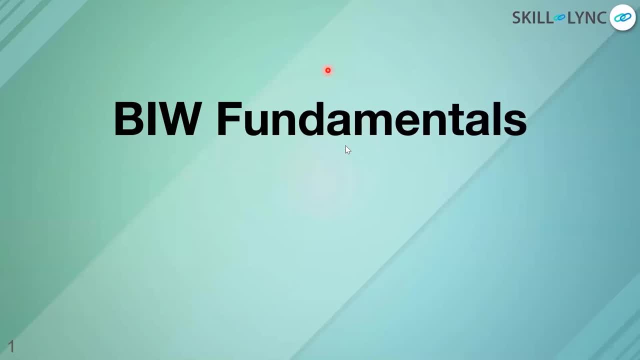 a similar kind of saying: skeleton of a vehicle for some body frame. So one person had given a good answer is Wazir Farooq. His body in white is the stage in automotive manufacturing in which a car body frame has been joined together. That is before painting and before 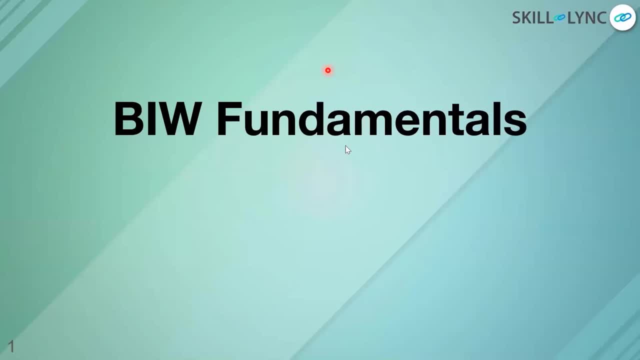 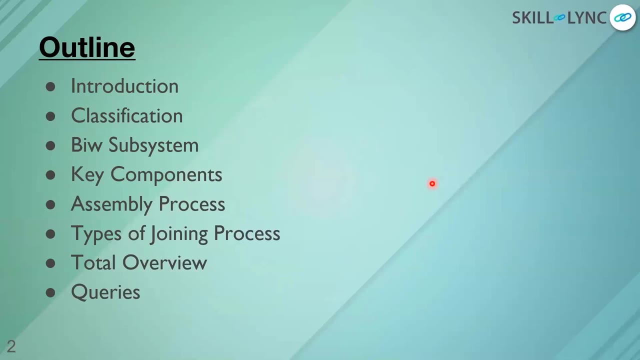 the motors. It's a very good answer Like this is the answer, what I'm expecting. So, guys, BIW is nothing, but it's a skeleton of a. not skeleton, It's a sheet metal: components of vehicle, Okay, Which has been assembled, joined together. So before that, this is the 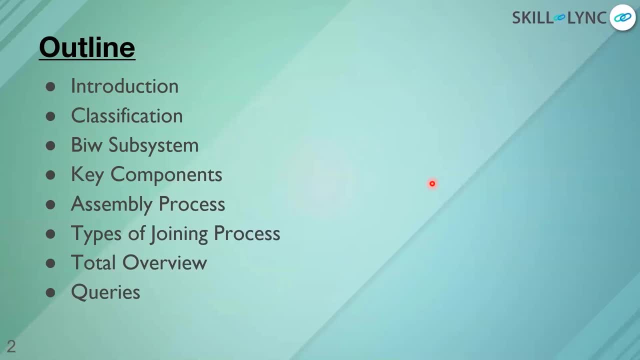 outline of today's session is like we will be having first going with in production, then classification, then BIW, subsystems, key components, assembly process, type of joining process, total overview and credits. So this is the sequence in which we are going. 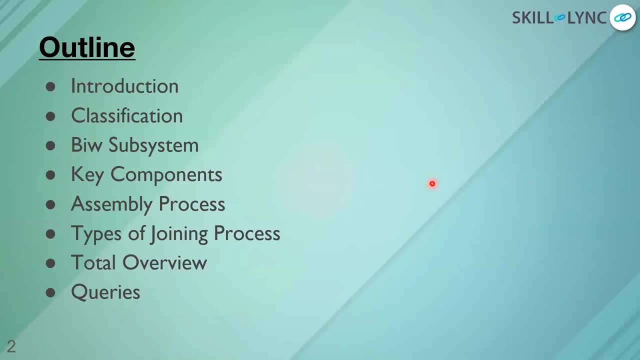 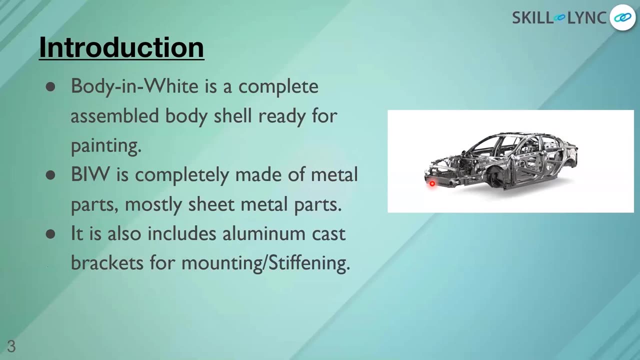 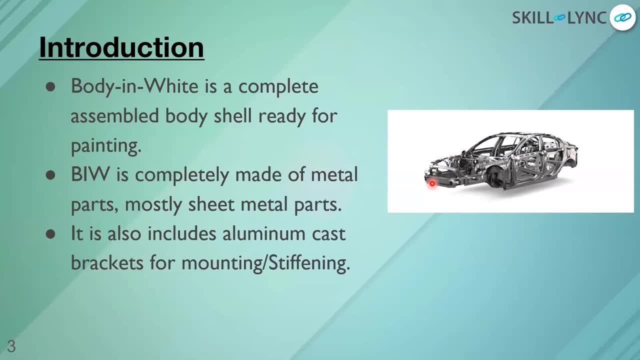 Okay. So what is CD? It's a catheter electronic deposition process, Okay So, in which we depower entire skeleton or entire sheet metal part of the body. we call it a monocoque structure because after this we assemble all the engines and the other components. 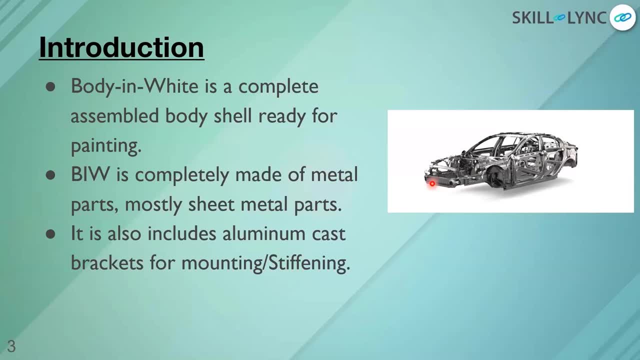 Okay, So in engine also we have seat metal, but we can't, we are not calling them as a BIW component. Why? Because when we dip this, these components all together with the skin panel. I have just deleted the skin panel over here with the skin panel all together. 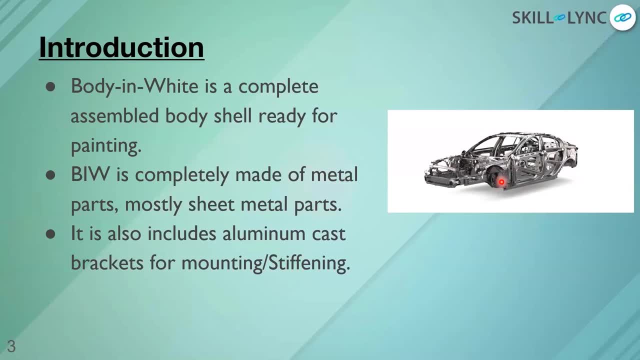 we call it BIW. So BIW is a complete, assembled body shell ready for painting. Okay, The blue is made of metal parts, mostly steel sheet metal parts, And in the very expensive car we have aluminum cast brackets and the other things also. Okay, 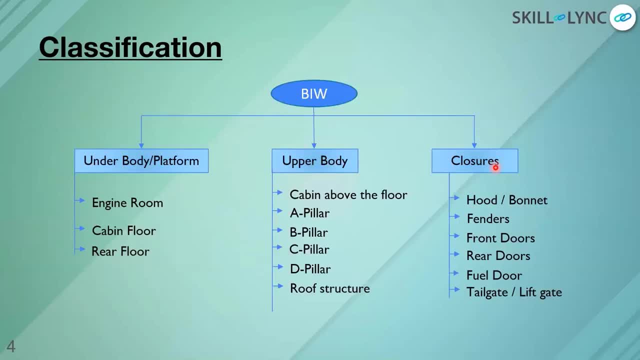 Hope you guys are clear with the BIW introduction. So when we call about BIW, we have divided it into three main segments. What are those? That is, underbody platform, where our chassis, engine, everything is getting mounted, Even the seats of the car, the fuel tank, everything. 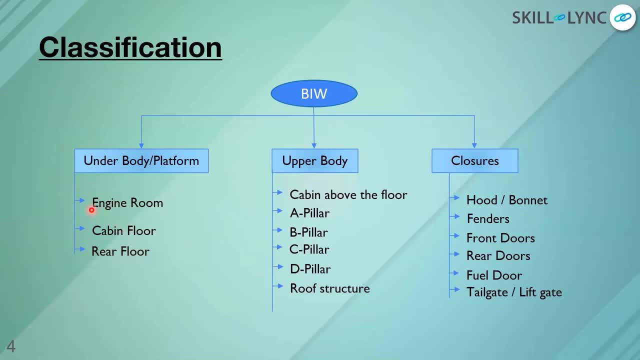 has been mounted. That is also been divided into three subunits: Engine room, cabin floor, where the seats are there, and the rear floor where the second seat and the third seats are being closed. That is the underbody, Okay, And we call it. 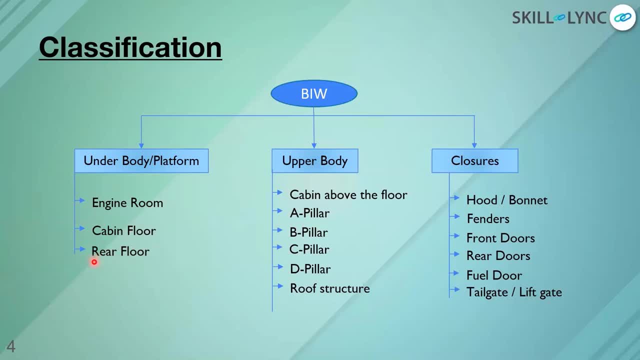 engine room and in cabin room and the rear floor zone we have our fuel tank, which I will explain you in the later slides how it has been placed and how it has been there. Okay, Then we have upper body, where we have cabin above the floor or whatever we have. 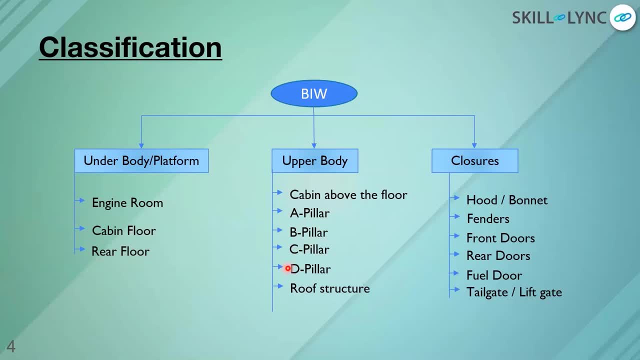 we have in there. We have B pillar, we have C pillar, we have D pillar, we have roof structure. Everything is coming into upper body category. Then we have closer. Why we call it closer? Anything which gets closed is closer. Okay, So we have hood. it is opening and closing. Yes, it's. 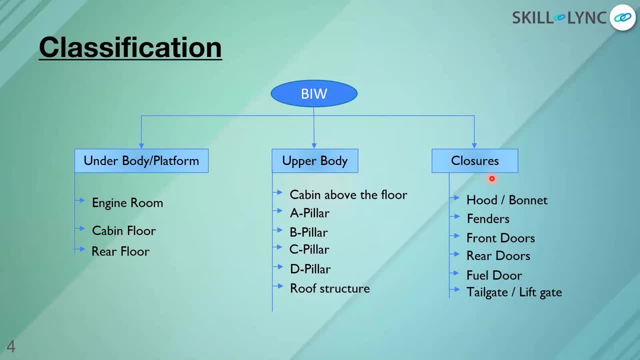 a closer. We have doors which is opening and closing, Yes, we do call it closer. We have even fuel trunk which opens, Okay, And closes Closer. So all the things which opens and close, we call it closer. In that there is 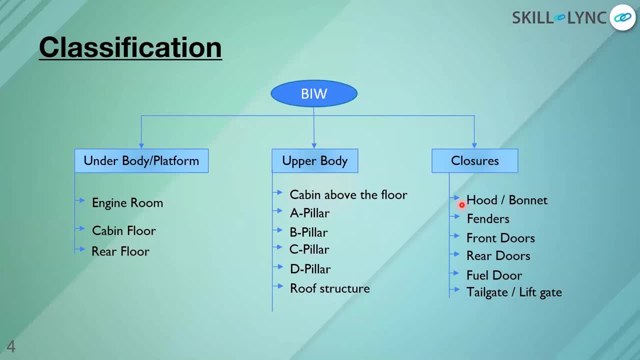 one component, which is fender. Okay, It doesn't close, but the thing with fender is doesn't weld also with the components. Okay, It's always getting bolted and it's. it doesn't have any uh safety regulations in the car. Okay, It's just a style uh feature and it. 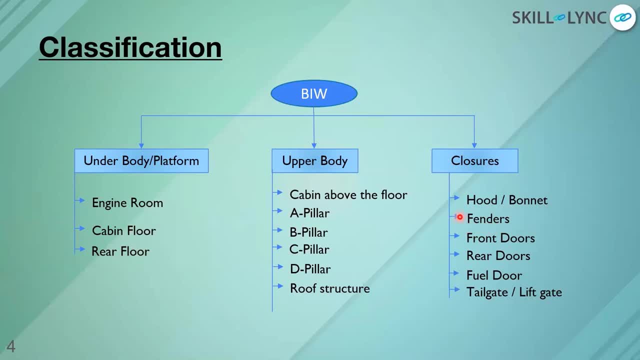 has some requirements, uh, based on the functionality, but it comes into closer department. Okay, So any doubt. Till here you guys have, as if you have any questions in this slide or in the previous slide that the that summit spoke about, please ask in the chat box. Okay, I think there are. 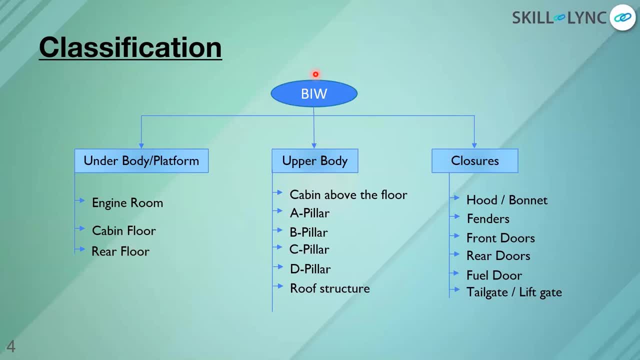 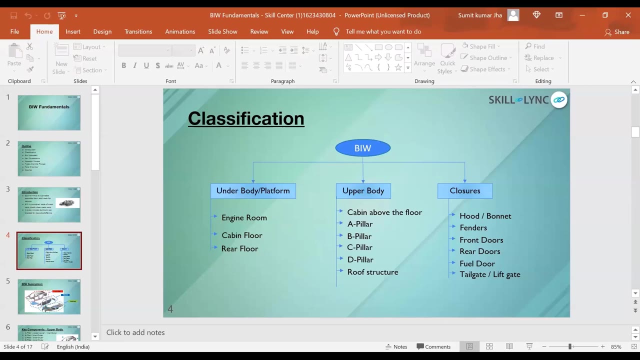 no questions, Artia. we asked what tailgate or lift gators. Yeah, I will explain you those things till Okay, Great So hood, ABC pillars: all those things will be explained in the upcoming upcoming slides. Yes, there is some issue with my presenting okay. okay, so what is upper body, what is closers and what is? 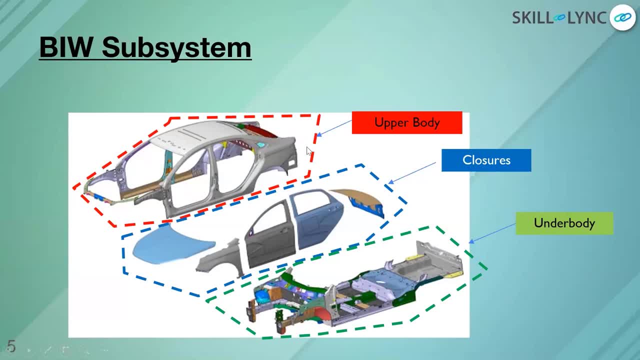 under. so this is the area which has been divided into uh the viw. as i showed, told you in the previous slide, it has been divided into these three areas. so what is upper body? this shell of the body which have body side outer, a pillar inside. this is the b pillar. we have c, pillar i. 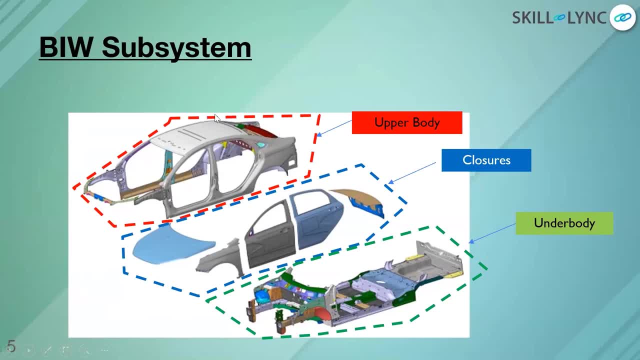 will show you what is c player, what is d pillar, everything this is the roof of the vehicle, okay. similarly, closers, hood, this component in closer, okay, this component in the closer, call as fender: okay. front door, rear door, hood: okay. front door, rear door, tailgate: okay. we have fuel trunk also. 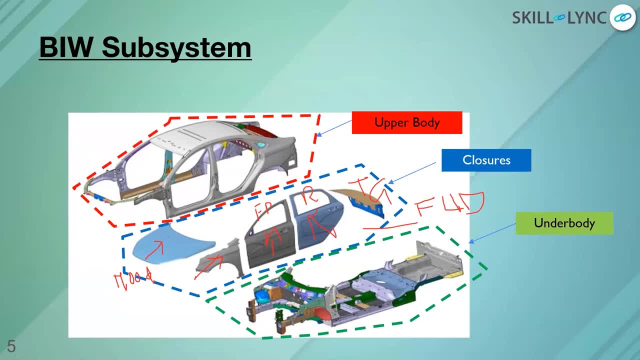 okay, fuel lid okay. so these things are closer in upper body. what we have, we have hood, sorry, roof- body side outer. it is the main styling component and this is the biggest component in automotive vehicle. okay, whenever somebody will ask you what is the biggest component, the body side outer. but in this also there is lot of engineering, like: 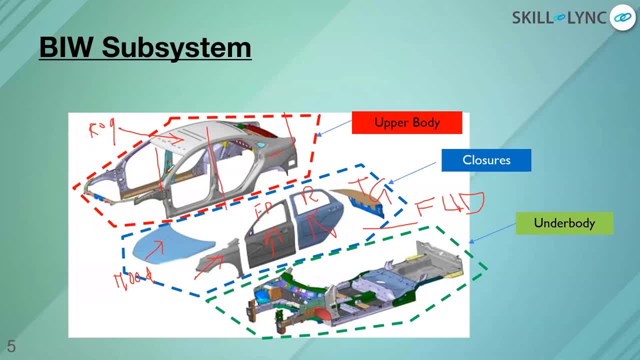 uh, this segment of the car is coming into frontal crash, okay. this segment of the car is coming into side crash and this is coming into no crash, okay. so sometimes what we do in vehicle is to have a two component joining together to make a bso. why? because in some area we need 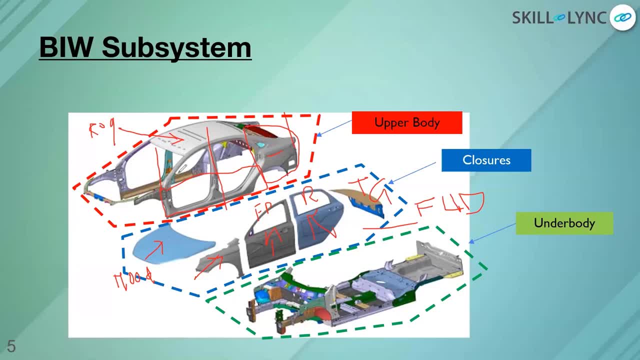 uh, more strength, and in some area we don't need more strength. so in that perspective, we just break this components. also, sometimes in honda, in duster, if you will see, it has been divided into two. in honda it is divided into three segments. okay, so this is a kind of design, uh strategy. what company? 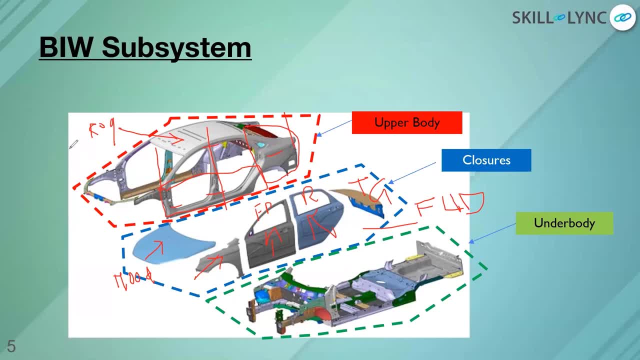 used to make to understand, because in automotive we have a number of regulations that is uh and we follow end cap new car assessment program in that we have country-wise regulation. we have 10 country uh regulations over there, which has usa, japan, canada uh, india, okay, uh, china, uh, australia, new zealand together, then korean uh, and then european. 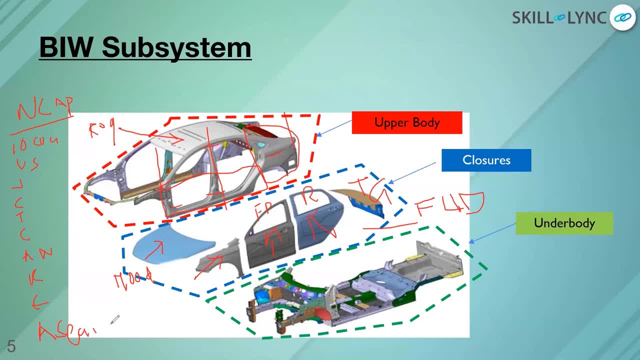 and then asean consist of all this. so this is again a different topic, but consisting considering all this country regulations we used to design all our this components. so in crash, the most important aspect is underbody. so our underbody is fully designed for the crash. okay, because it have all the features it have: front seat here, rear seat here, 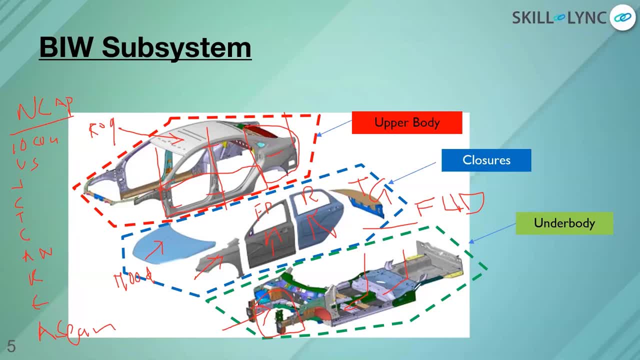 okay, it have engine compartment in this zone. okay, it have fuel tank under this uh small zone, under this zone. spare wheels coming inside this. if we have a third wheel, uh, third seat, it will be coming here. so, spare wheel: if there is a third seat, the spare will not come in this area, it will come bottom of the car. 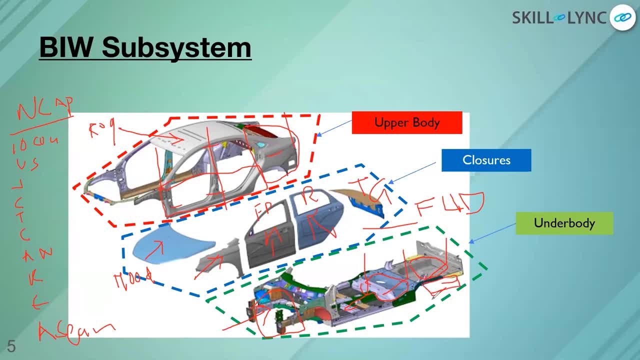 we have the axle mounted in the bottom side of this area, we have exhaust going through from the center of the tunnel, which i will explain you in the later slides. okay, and then this area. we have axle, we have engine, we have transmission, ac unit, everything, whatever you see in the car. 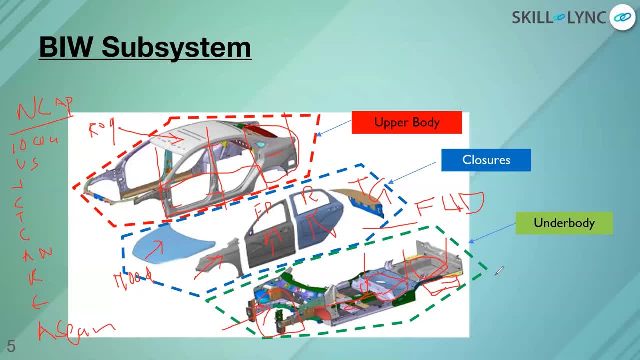 uh, in the, in these blocks are being mounted in underbody, so this is the biggest robust zone of the vehicle. what is upper body? it's the second robust zone of the vehicle and the area which is not very much strong it's other, closer. okay, so all together, when we weights all the thing it is, it comes. 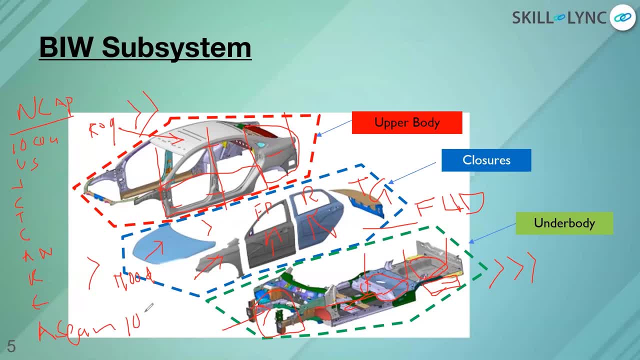 around thousand, uh, like, uh, this, uh, the entire weight of the vehicle is something 1300 kgs. okay, say, a normal suv car where this all combined together gives you around 400 to 500 kgs. okay, and then rest of the components are different. okay, clear, okay. so till now, guys, you are clear. 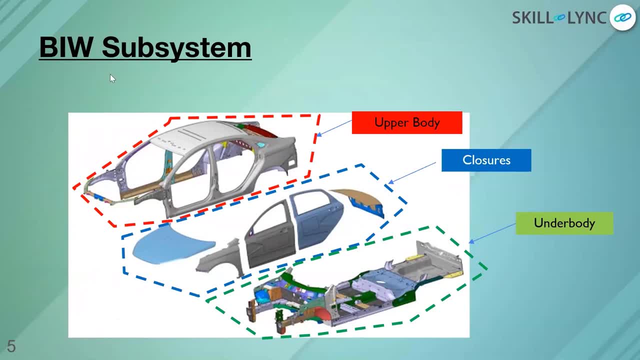 with the thing or you have any doubt. if you have any questions, please let us know in the chat box. uh, with respect to upper body closures or underbody: okay, it looks like they are clear. okay, great, great, so this is how we do our uh. uh, this is our biw subsystem. then, talking about the 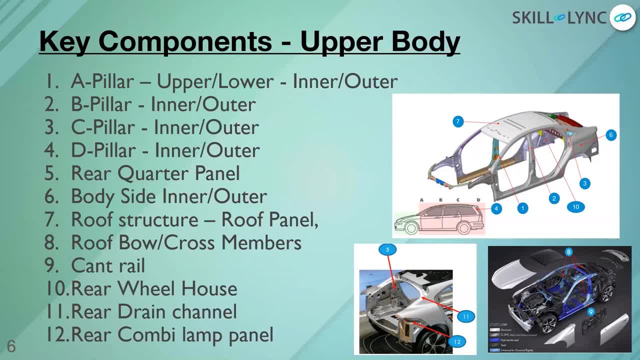 key components in upper body. so when we are talking, like somebody have asked me what is a pillar, what is b player, what is c player, t player, so here, if you can see a complete, uh, bigger picture of a in a bigger mpv vehicle, okay, so a pillar is the pillar which we have it here. okay, we have. 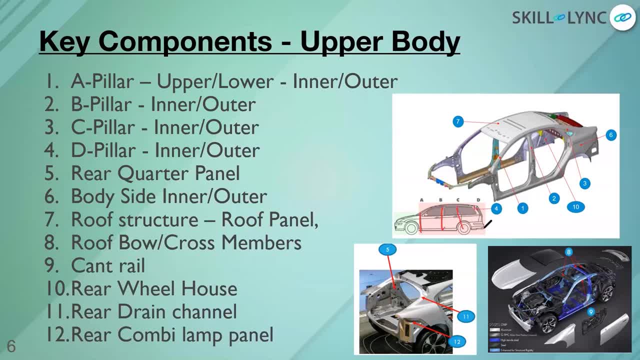 b pillar here, you have c player here and we have d player here. so all together we call it a vehicle will having a uh around, uh d uh. four pillars in the vehicles. can anyone say me why we need pillars in vehicle? type it in the chat box: uh, the question is: why we? why do we need pillars in vehicles? stability. 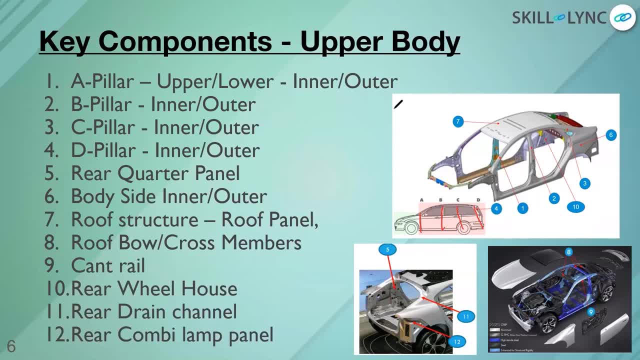 somebody said, yeah, support, yes, what else to sustain load? okay, very good. so, uh, uh, yes, actually, uh, this pillars uh very much required for the strength and stability. at the same time, we use it for having a very good stiffness throughout the vehicle. okay, as we know, for uh, for these zones, we need, uh, we have a door, okay, so this all other very uh. 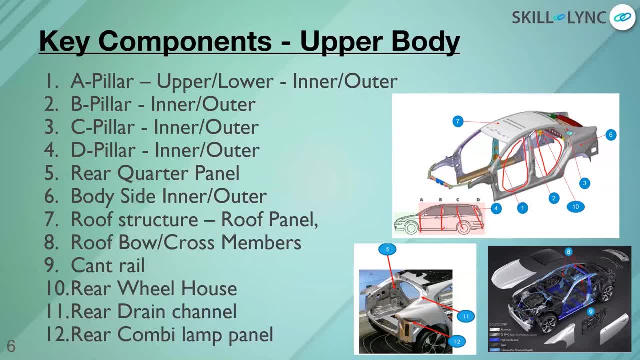 it's a vacant areas, okay when the loads are like: uh, if we consider the torsional stiffness of the vehicle, how that? can somebody? someone tell me what is torsional stiffness? and carry load parts? okay for carrying upper aluminum, carbon steel? no, we are not using those kind of till now, so 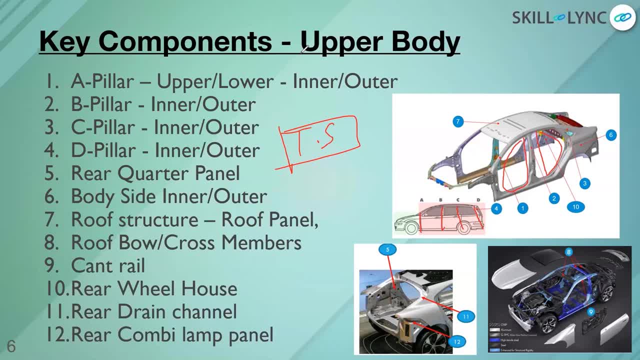 the question is: what is torsional stiffness? right? uh, yes, yeah. so punit kumar says strength to resist shear force. okay, resist torsion, okay, so, okay. so i, i believe, like all you have your own understanding on on this and i'm not saying anything is wrong in here, it's correct. 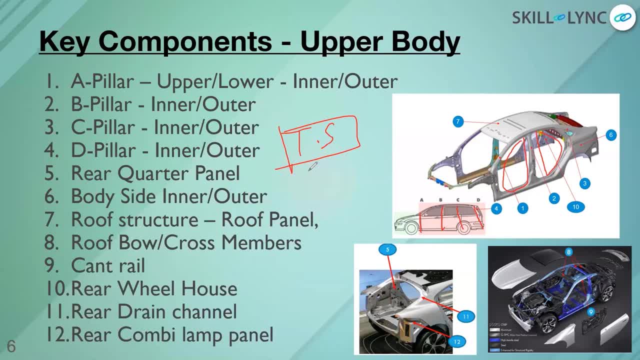 but uh, you have to i. i will just show you an example. okay, just, we will consider a piece of piece of paper. if we are going to rotate it with this axis, it is all uh easily rotatable, right, okay. so, but if we make it a frame outside the, uh suppose, just take a consider of a frame picture. 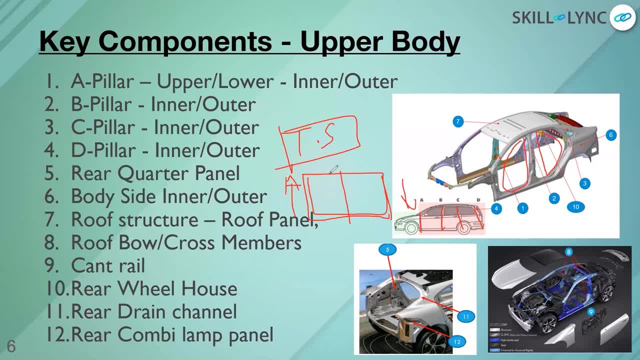 frame. if we only twist the paper inside the picture frame, it can easily rotatable, but if we take the frame and we will try to twist it, it won't because we had provided a stiffness throughout the boundaries. okay, so what is stiffness? and okay, you will say why, how it is important in uh car, because when we have a car, okay, 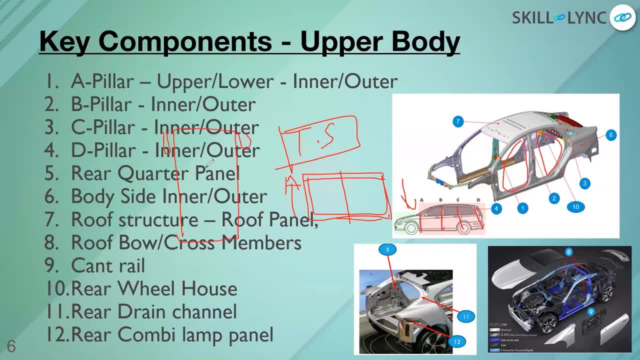 suppose this is a car with four wheels. okay, when we are driving in a twisting area like it's- uh, it's in a? u, it's kind of curving. so what will happen? we have two forces acting on it in one in here, one in here. so if we won't provide this kind of pillar, what will happen? 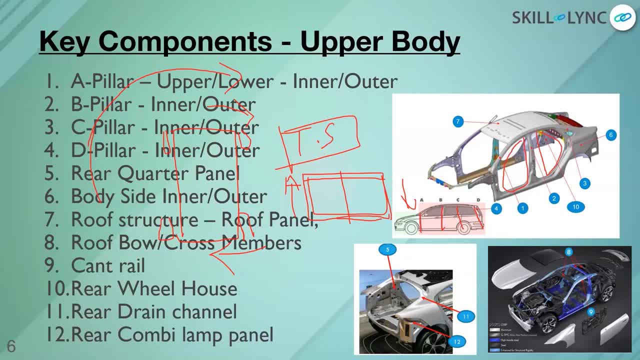 stronger pillars. what will happen? this areas will become slightly deformed, okay, and the vehicle will become unstable, as because we, we don't have a good torsional stiffness in the vehicle. so to provide strength, uh, in the vehicle and to provide a very good stiffness, uh, torsional stiffness, which 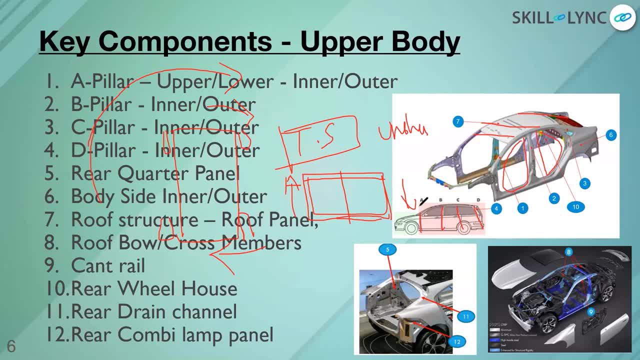 enhances the vehicle dynamics and the vehicle dynamics and the vehicle dynamics and the vehicle performance. we have to use this kind of uh stiffness, uh pillars in the vehicle. okay, for mpv we need four because we have a bigger zone from c to d, which is unavoidable, which we can't avoid, but when? 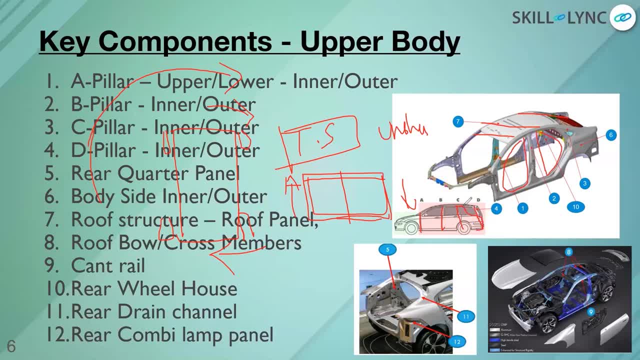 we have sedan from here. it goes down like this: in this we don't need it because the height over here is not much. okay, so we only use c pillar up to c pillar when we have hatchback. we sometimes don't have a c pillar. also, we just manages with a and b pillar, okay, so this is how the pillar uh designs. 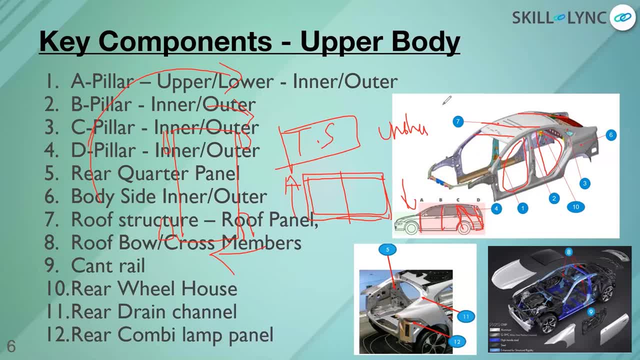 takes place in the vehicle, all clear? or anyone have any doubt in pillars? these are all the components uh in vehicle. so this is the a pillar, this is the b pillar, component two. this is the c pillar, component three and d pillar. we don't have it here. i can show it in here, okay. rear quatra panel is. 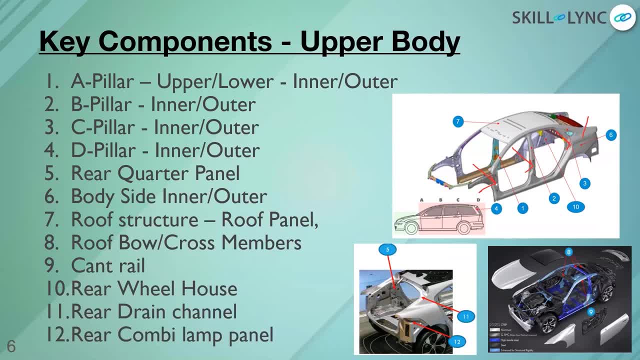 okay, uh, we have it in here and here. inside quarter panel will be there inside this panel. and this is the bso body side, inner outer, okay, and this is the part which reinforce it from the inside. it have rear quarter panel, okay. seven is the roof structure. this one, then roof boss: uh is here, we have it here. 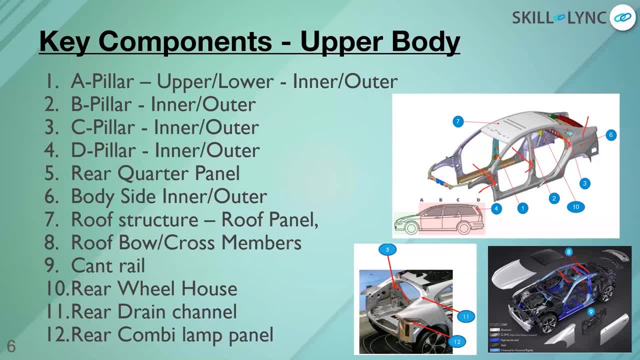 here, front, middle rear, and this also depends on the length of the car. if the length of the car is huge, okay. if the roof is huge, then we have to divide it more. okay, again, the factor is same, uh, torsional stiffness and the bow. the roof is not welded with the vehicle, it is sometimes welded, laser welded. and in this area, 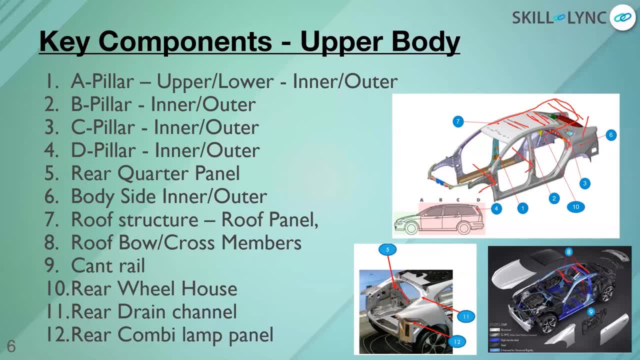 it has to be mastic with the reinforcements. what we have it in here. okay, so we need more uh roof reinforcers in this part of the vehicle. uh, then we have can trail. okay, this is the can trail. okay, you can see it in here. okay, we have rear wheelhouse. okay, that is uh somewhere here inside because uh here wheel. 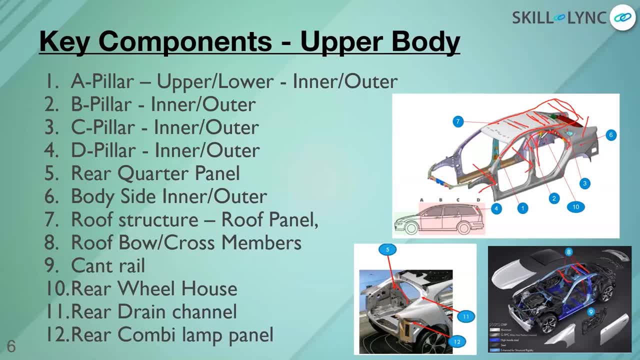 housing. we call it because inside this, only the wheel movement will be there and the suspension also will be mounted in here. okay, then we have rear drain channel, which is used to uh drop the passenger into passenger compartment for the passenger. so this vehicle runs this rain uh. 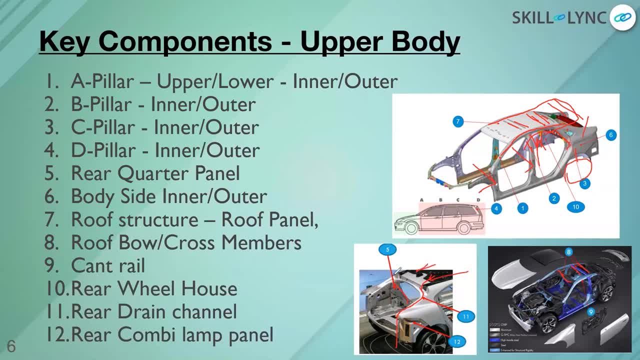 because if it is moving, the vehicle traverses the vehicle on the road and but the vehicle is moving, it does not enter the passenger compartment here, so the runner will be right here and all the water is coming down here whenever it's coming, where it's raining, suppose, and all the waters. 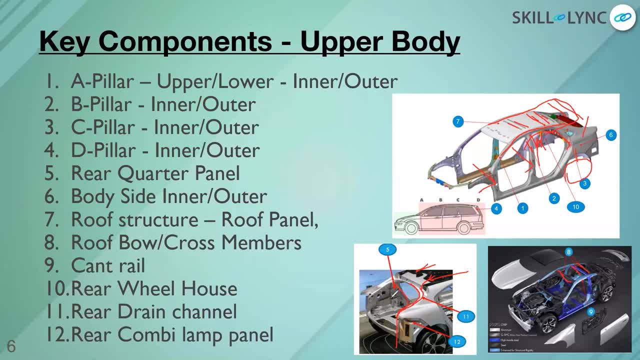 are coming down here, all because the vehicle is moving, all due to the aerodynamic, all the water will be coming and it should not enter into passenger compartment. so we have this rain, uh drip. so in this lamp panel, other than this, we have a big cutout, which we call it a body exhaust, a car. 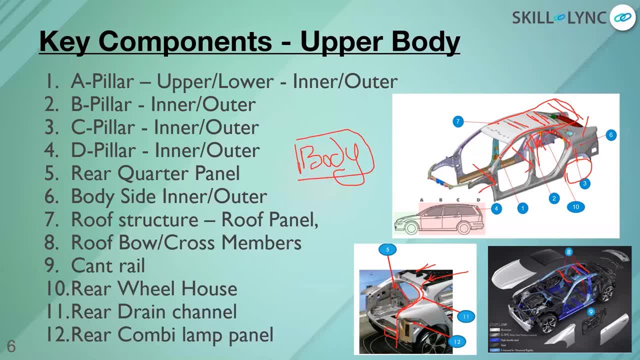 body exhaust. okay, we have two kind of exhaust. one is the exhaust which is coming from the engine, one is inside volume volume, inside the volume of cabin passenger. we have one more exhaust. okay, can anyone say, like, why we need this exhaust? sorry, uh, i think they are answering that in the 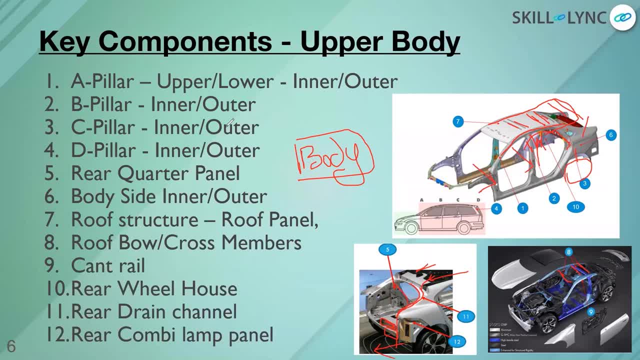 chat box. somebody have told dampening somebody have to remove the co2. i i'm not saying it from the exhaust, i'm saying it's from the body. uh, volume okay. ventilation like a ventilation, very good. which type of coating used for cars to withstand environmental condition okay? 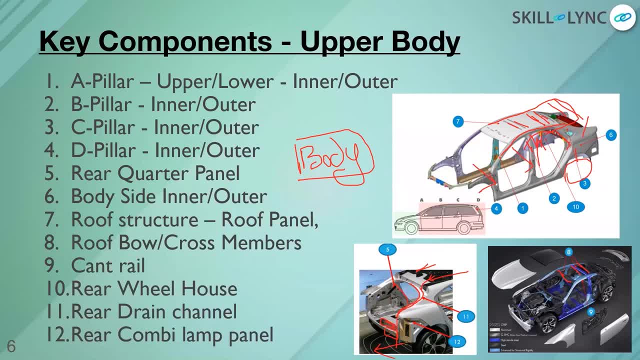 i will answer you this question after the session, when we are answering all the questions. because of ventilation, to remove heat, to release the pressure? yes, then akash showed the answer. uh, yes, this is the answer. what i'm expecting? uh, to release the pressure inside, okay, suppose we have a closed structure? uh, closed packed uh chamber, okay, and 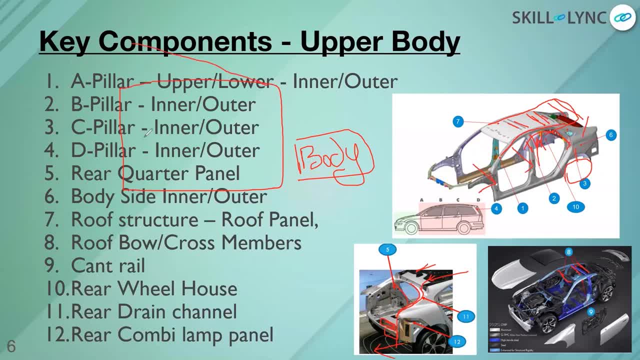 if we have a very good ceilings and all the air will not come out and suppose, when air conditioning is going on, everything is going on. so whenever we close the door, okay, as the air come inside, this is so much huge it won't allow us, uh, the door to get closed. okay, because it it will reflect. but 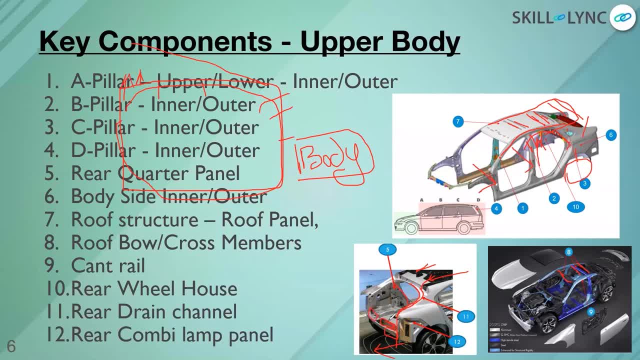 due to that, we have this kind of small, small exhaust inside the vehicle which releases this airs okay and doesn't create this huge pressure for the doors to get locked, okay. so this is the reason and again, second reason is we have to recirculate the air inside the car. one is with 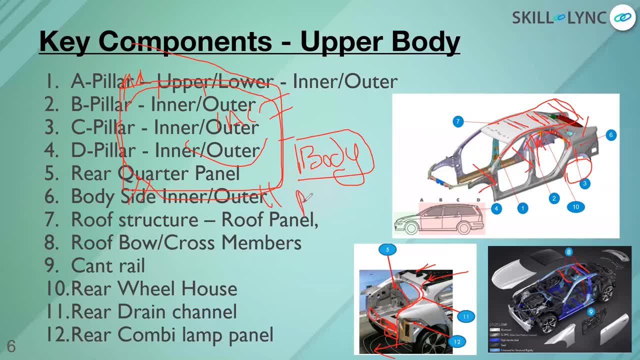 another is with this kind of exhaust, so that the pm particulate matter inside the car should not be huge. okay, so this is the reason why we use it. so, akshay, you are right. okay, so this is uh, uh about upper body. if anyone have any doubt related to upper body, they can ask, and then we will switch. 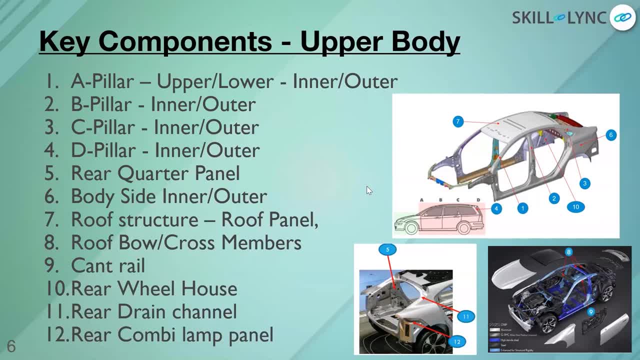 to closers. clear material of upper body- okay, torsional stiffness and material of what is can train- okay, can't get what you said about second exhaust, okay, okay, so we will answer one by one. surya, can you help me with the portions sequence? okay, so first, sorry, sorry to involve you. no, no, no, okay, so uh. 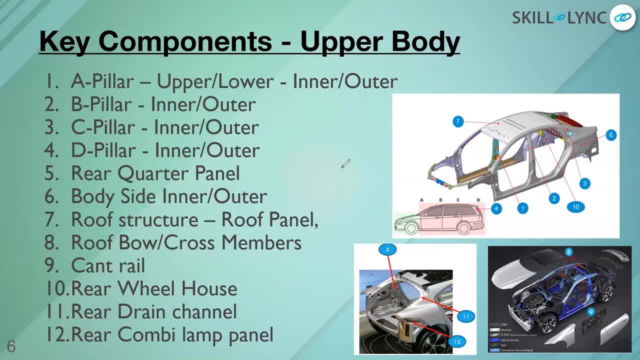 material of upper body is a very important uh aspect. okay, so what we have to understand is: like what kind of uh uh purpose this upper body solves? okay, so we uh in vehicle. mostly we use steel. okay, so in steel we have lot of grades with. we call it lesser yield grade and higher yield grade. 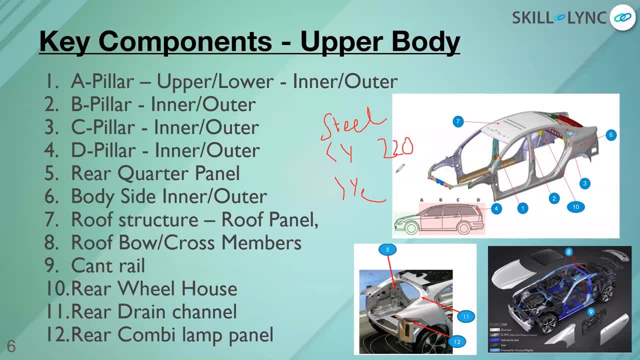 okay, so lesser is something around 200 to 220 mpa and higher is around 880 mpa. okay, we use this kind of steels in the car. but now what is important is like if roof- if suppose we consider roof, roof- is not coming in any crash? 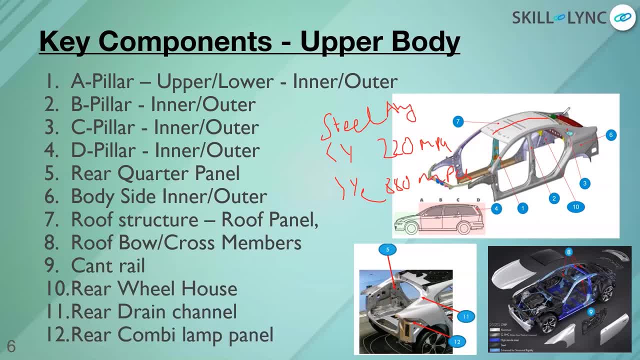 requirement: okay. no, crash requirement comes under roof. there is something coming for 2022 for that we are considering, but that is again for the pillars, not for the roof. okay. so for roof, we always go for the lower yield. uh, steel, okay, but if you will see a pillar, b pillar, okay. so these 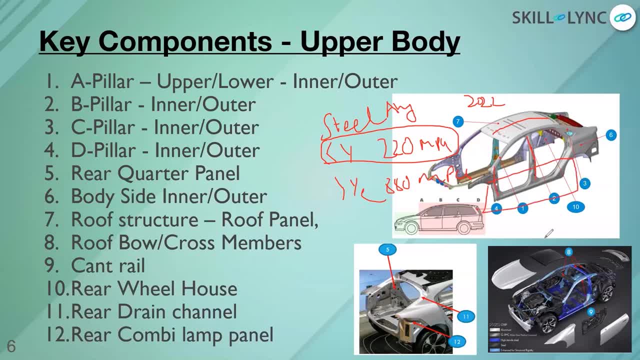 components are okay, so these components are okay. so these components are directly coming under go under side impact. directly coming under. go under side impact. directly coming under go under side impact test test test. okay so in side impact test and the pole. okay so in side impact test and the pole. 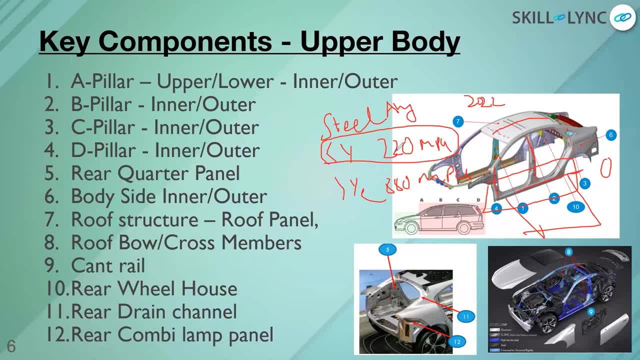 okay, so in side impact test and the pole impact test, this component are directly impact test, this component are directly impact test, this component are directly coming into play. so we can't use 220 to coming into play. so we can't use 220 to coming into play. so we can't use 220 to 220 because the yield, the crash, uh pulse. 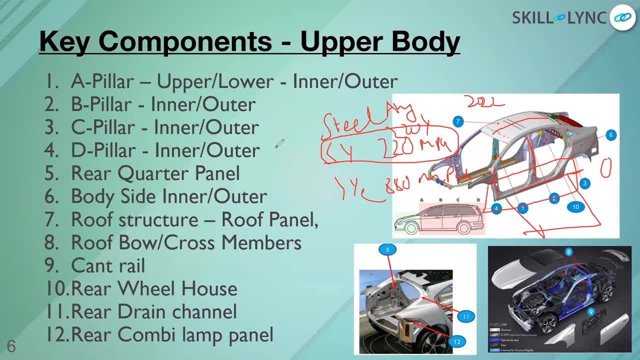 220 because the yield the crash uh pulse. 220 because the yield, the crash uh pulse what is getting generated. it's more than what is getting generated. it's more than what is getting generated. it's more than 220, it's around 350 to 400. 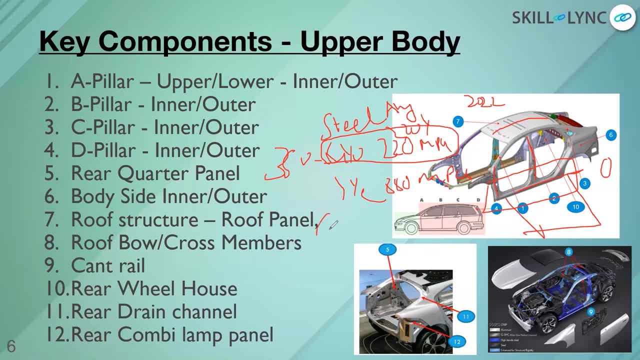 220, it's around 350 to 400. 220- it's around 350 to 400. so what we do in this area, we try to use something around 600 mps. okay, and that also there is a catch, okay, uh, the crash occurs only. 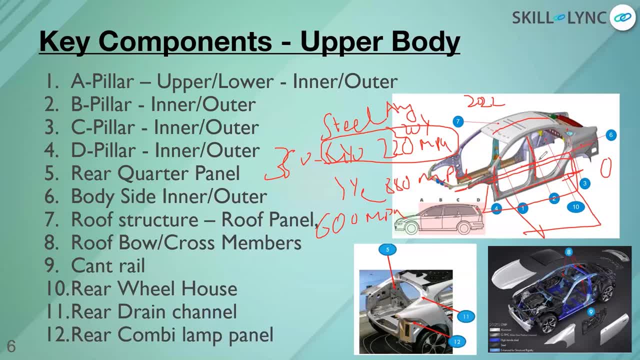 in this part of the vehicle. okay, up to this zone of the vehicle. okay, so what we do we? we make a laser, uh, welding for d pillar, okay, so what we will do. suppose this is a b pillar of the car? okay, so what we do? till here we will use 600 mpa, okay, or higher thickness, higher thickness. 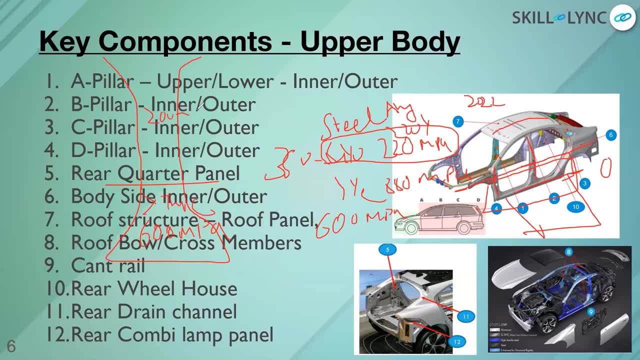 and above this, we will use again 200 to 300 m. okay, why we use this? because this is a very expensive steel. okay, so we, if we use it throughout the component, it will make it a expensive part. okay, so what we do? we just do it, uh like, we just trim the part into. 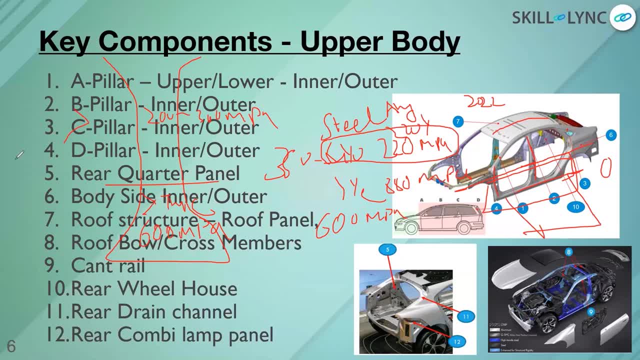 two components again for 600 mpa. uh forming is a challenge, okay, forming is kind of a manufacturing process to give a sheet to this form. okay, so this is again a different uh subject altogether. for this, what we used to do, we do hot stamping, okay, hot stamping is something in which we take the 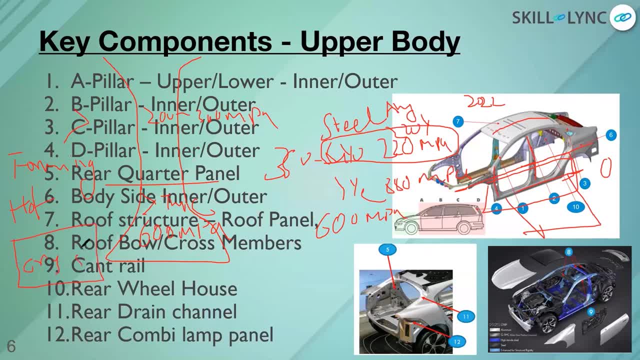 steel into crystallization temperature, something around 800 degree centigrade. we heat it and then we form it. so again, if we do it for a bigger component, the call the part getting colder is more timer. it will take more time, okay, and for this small component it will take lesser time. 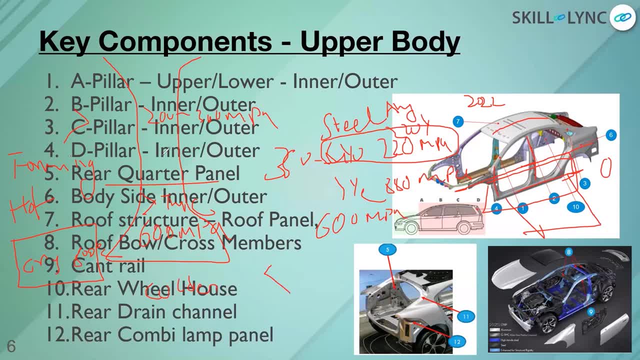 so that is also one of the reason we go with two kind of stiffness in this area. all clear. so that is again how we select the steel here. bso is a part which doesn't uh help in the crash. okay, so we use again the lesser yield. but cantrell is a component inside. okay, uh, cantrell is a component which is. 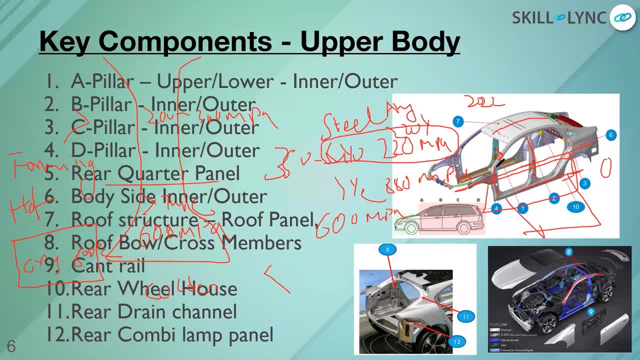 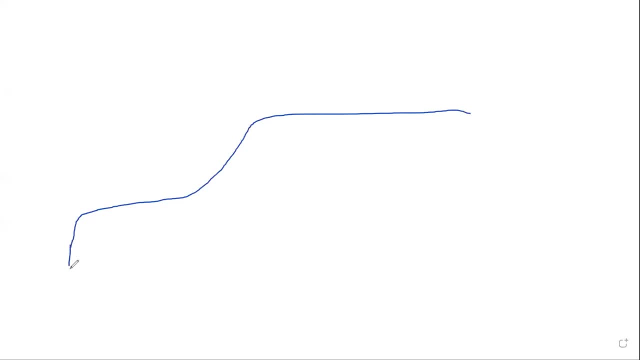 inside this area, which, which is with the aerodynamic of the car, we use it. i think this is also one of the questions somebody's asked: what is cantrell and why you use it? so if i share a whiteboard, yeah, can you see my can like whiteboard. yes, yes, okay, okay. so suppose this is the car, okay. 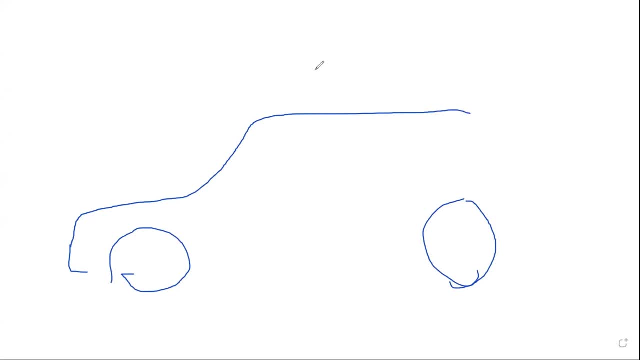 somebody asked me what is canceled. okay, so for that sorry sketch. okay, so suppose this is the car. okay, okay, so we know our driver is sitting here. right, this is the position of the driver sitting in here in the seat. okay, suppose this is the pitch. suppose any crash is happening. 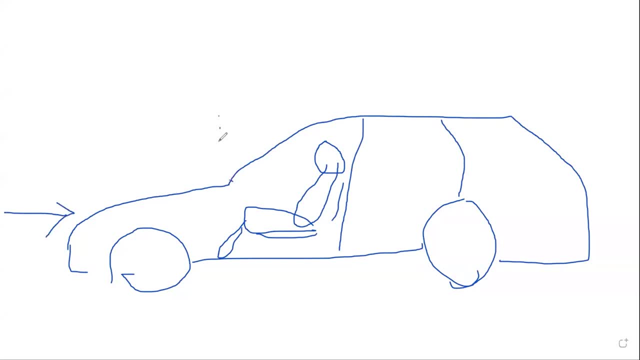 from the front. so this can't will. before it was something like this in the previous- uh see, old car. these are not much aerodynamic. so nowadays the car become more aerodynamic. okay, just to take the load air in a very well manner so that the downward force will be good. 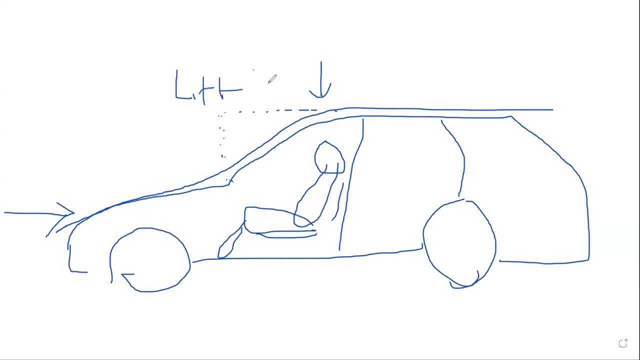 uh, the lift force will be, uh, good, there won't be any drag force, uh, lesser drag force, so that the efficiency will enhance. okay, so then. but what is the challenge in this kind of thing? if you see this, this structure, whenever the crash will happen, the driver head is well safe from the top, from the 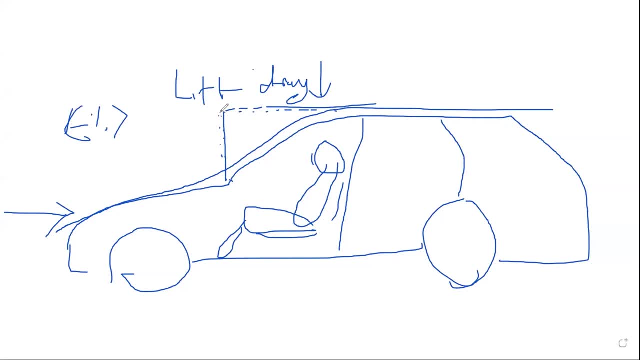 here and from here. okay, it's none nowhere near to the these kind of pillars. but now what happened when we had this aerodynamical consideration? what we did? we bought this pillar near to the driver's head zone, okay, so now this player, have to be very much strength there, because if the crash, 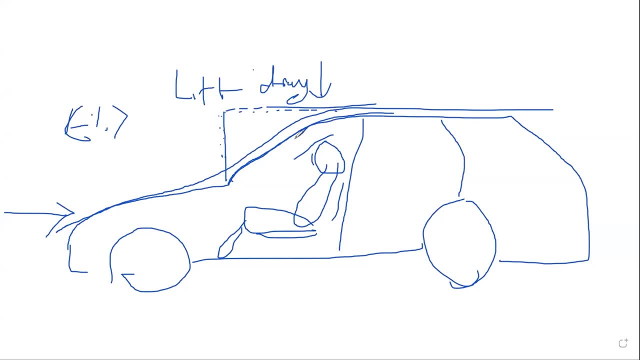 it happened, it should not come in here. so what we do in this area? we make a program deformation. suppose a deformation is happening whenever the crash is occurring and the deformation is coming in here, we make our crash in such a way the deformation will always happen in. 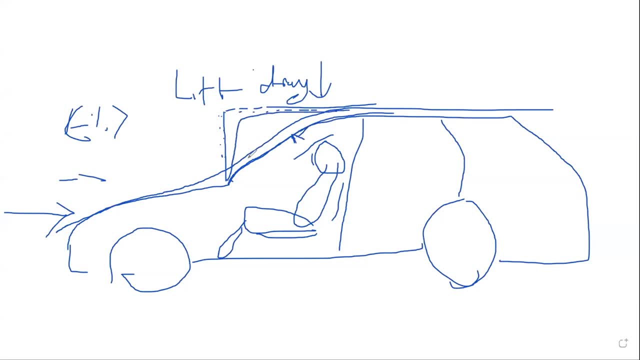 this direction means, this will break in this manner, not in this manner. okay, that's why we call it here a program deformation. so we give a crack and whatever load will come, the crack will only come in the in this direction. so this will break in this direction. so we have this deformation. 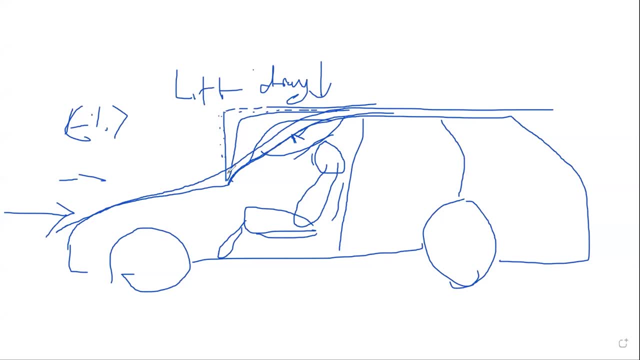 always come in this area. okay, so cantrel- why we use cantrel to this- is a one ribbon which takes vehicle from front to the end. and why is it in this shape? now? because to consider, as we are considering, aerodynamic structure, so this have to be here. okay, in here, and the glasses will be also. 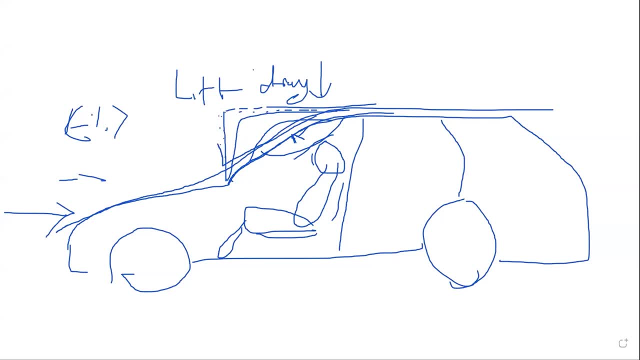 coming and resting on the cantrel. I hope your doubt for cantrel is done. so there is one more question someone have asked me. that is regarding: okay, a build up a body with 3d printer, will it have more strength? but what material you are using? again, it's a very expensive and time-taking. 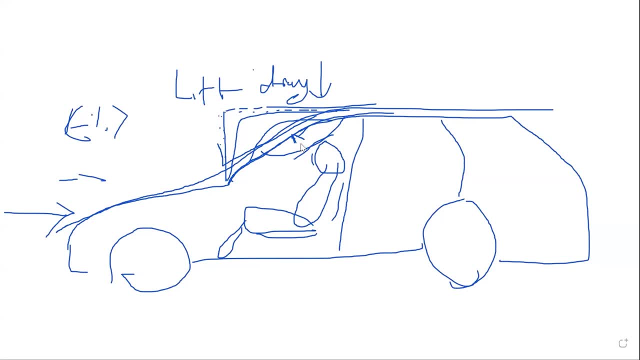 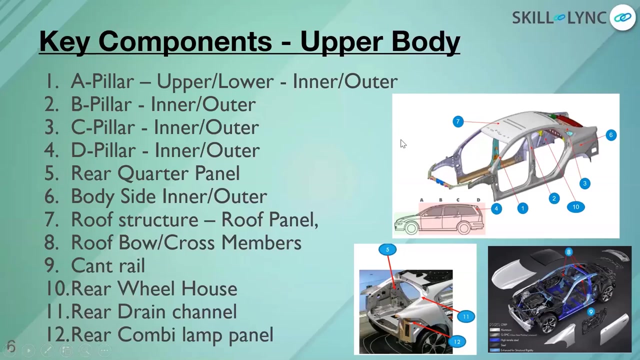 process. one thought process is, since there will be questions parallel to the topic that you also teach, what we can do is, for those kind of questions, we can keep it at the end so that your flow kind of goes: fine, okay, sure, I want them to get cleared in every area, like, yeah, absolutely, absolutely so for the, for the questions. 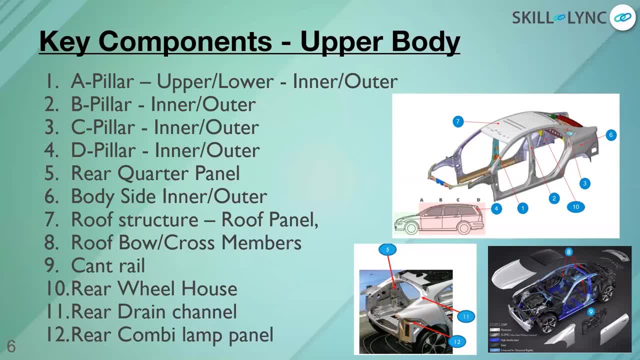 that they have about these topics that you teach. yeah, that I am answering. if we they are questioning something apart from the topic, guys, please make it sure, like we will be doing in the end of the session, so that I can answer you in a very well manner. okay, so right now, if I'm asking you some question, try. 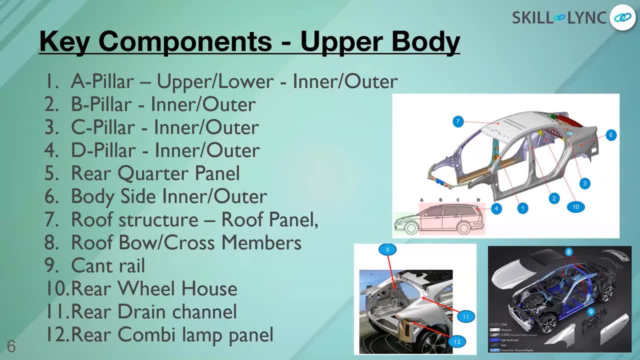 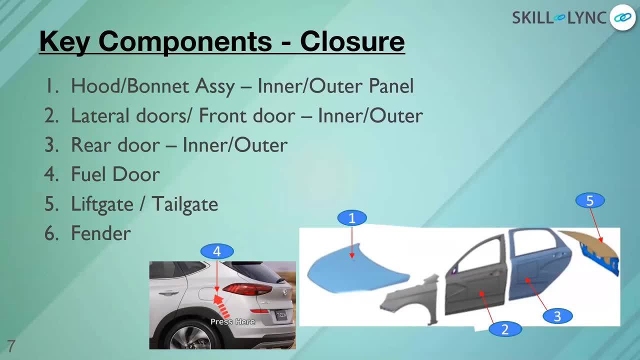 to answer in that way, in that zone only. okay, upper body question thing is clear with you. then we have under body, sorry, closers. as I have told you, the components which are getting closed are closer, but we have a separate part which is fender. why fender is not inside upper body and under body? because it is a part which is not been welded. 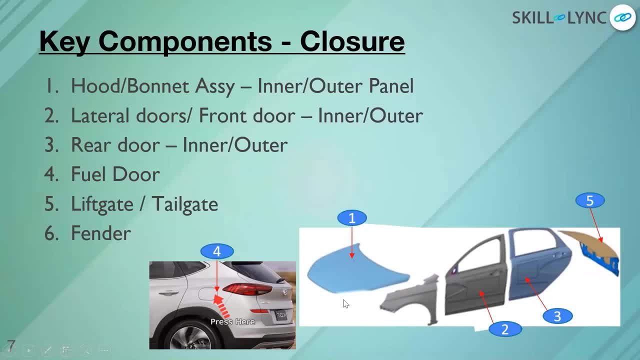 into the car. it has always been bolted into the car. okay. so under body zone all together it comes as a weld component. upper body comes as a weld component. then they will fit all this component inside the car. that's why we call all these closers okay. same applies for fender, but it doesn't open. 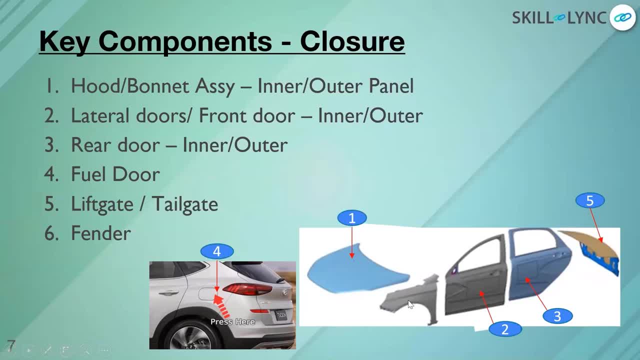 and closes. it always gets closed. it never get opens. if we want to open, then that is a different criteria. so this is the component: hood, bonnet assembly. we call this hood. second is lateral door and front door. that is the this one, the frontal door, this is the rear door. fourth one is the trunk fuel door or 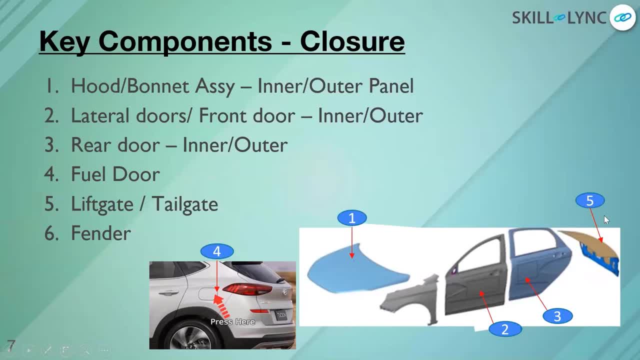 trunk lead, we call it, okay, sorry, fuel lead, we call it trunk. we call for doors, tailgate- okay. and then fender is the fifth one. the balloon got missed, okay, so this is. this is about fender. somebody have asked me- I have just seen in the questionnaire somebody is asking: what is fmvss for hood? okay, so. 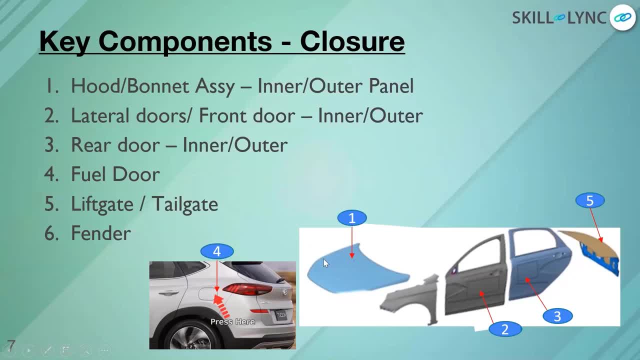 have to understand what is fmvss. it's a united states law for the crash, okay, for hood. yes, we have pedestrian head impact, but it have different consideration. us is the only country which don't have a head impact initially, but now they have to integrate it okay. so that is something different. 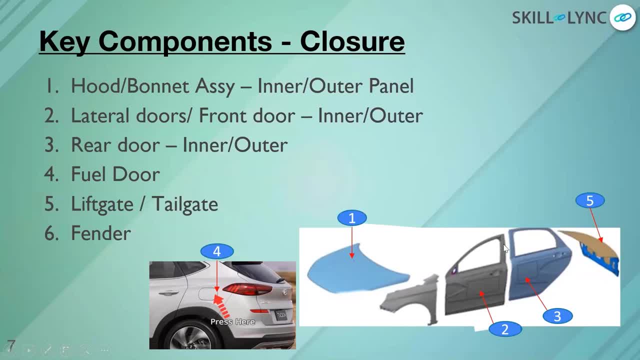 okay, so these are the components. whenever we design our doors, we have to take a lot of thing into consideration. okay, so the first thing is open and closes the door. okay, so we, whenever we design and when we test, so we closes the door like a lakh times one. lakh eight thousand is the cycle. 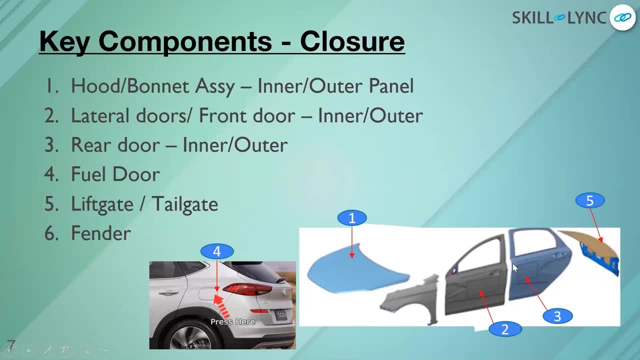 time for a door to open and close, okay. similarly, it is for the rear door. this is not for one lakh, it is for some 64 000 and 48 000 times. this is how the testing for the doors have been done. so in this testing what we see, the doors should not get, uh, bended. 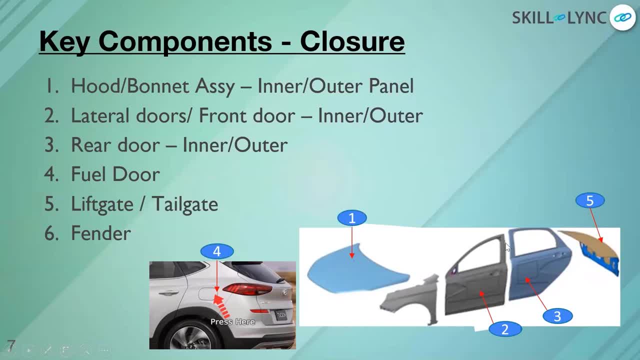 it not that deteriorated, it should not bend, it should not deteriorate and it should not break anywhere. okay, with this one lakh eight thousand cycles. so this is what kind of test we do for the doors, the similar kind of test we do for hood, but the numbers are not huge. uh, like one lakh it is. 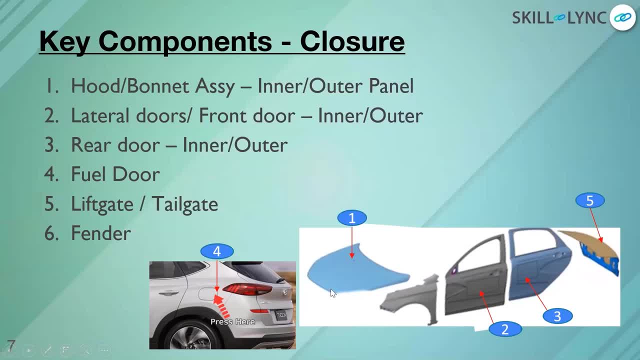 around thirty thousand or forty thousand for some of the regulations. okay, because we open doors more frequently than the hood. okay, in this also, we have primary lock, secondary lock. okay, so, uh, anyone know what is secondary lock and why we use it? no, uh, this is not related to child lock. suppose you are driving if we we have a secondary lock, if 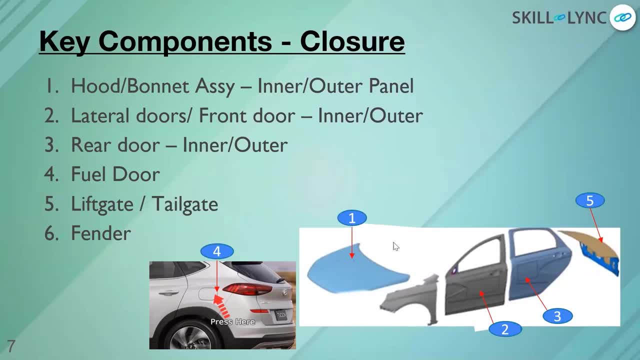 whoever driving a car they might be knowing, like when we open a bonnet it won't open full, okay, it will, just the primary lock will be unengaged and the secondary rock is always a manual lock. it's. it should not be uh, automatic or uh, it's a motor. 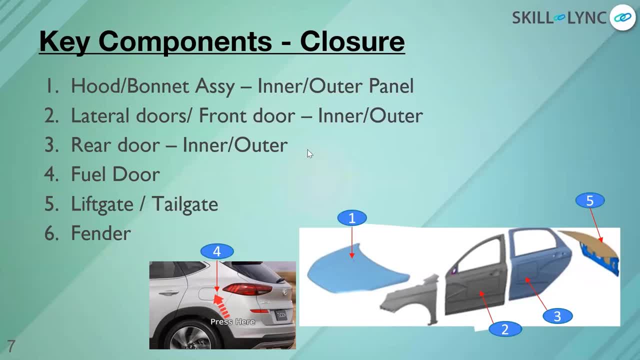 uh one, why? because suppose you are driving in a speed of 120 kmph. okay, suppose you are driving your car in a high speed, okay, and all the aerodynamic effect is happening in here, and suddenly, by mistake, you triggered your hand on this. uh, latch area for the hood. so this will all. 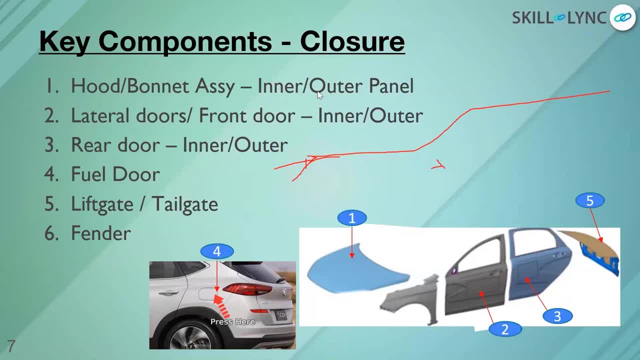 due to the air effect, it will open like this: okay, so it will open. so what will happen? you will have a uh, this uh like your uh visionary will be getting affected and you may crash in the uh your vehicle somewhere. so, all due to this reason, we always have a secondary lock in here, which is only accessible. 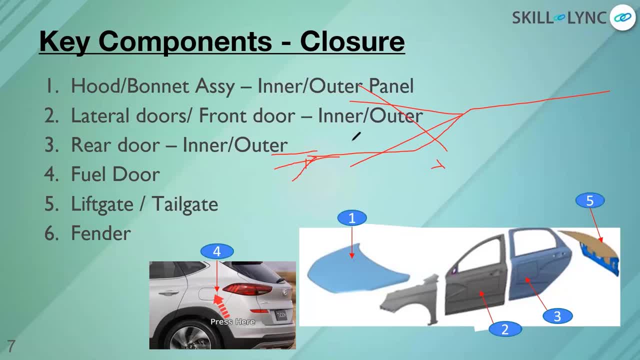 by the hands. okay, so suppose you are driving in a high speed and your, by accident, your hood, uh, the primary lock, get disengaged. this will not open, it will still be intact, okay, but you will feel some which will alarm you, that okay, this area is. nowadays we have a digital cluster. it shows 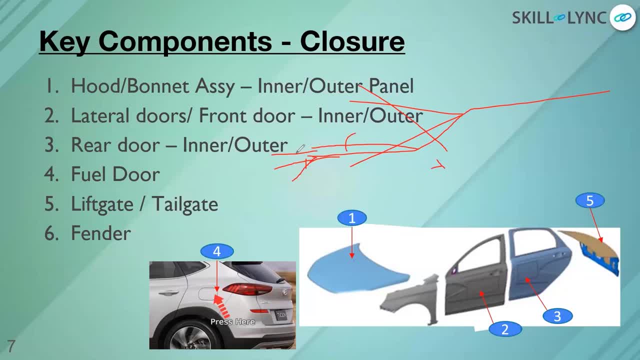 okay, your bonnet primary lock is open. okay, so that you can open. okay, that is the only reason why we have still a manual locking in this area, not a uh electronic locking for any kind of car. okay, that is what why we use uh hood, uh like, uh in that purpose. uh. second is like all the closer. 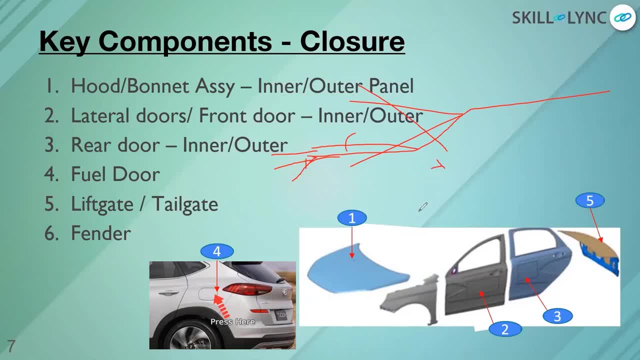 components: uh, the components are not a very uh like. they are not into lot of uh crash regulations. okay, we have some regulation related to pedestrian impact but not related to high crash, like uh kind of uh. uh, we call like uh the load absorbing and all. but that is for hood tender also doesn't. 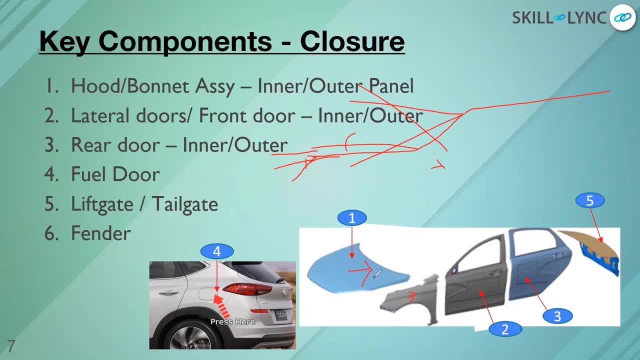 absorb any load. hood also doesn't absorb any load. but with hood what we have, we again, as i explained you about the can trail, okay, how the deformation happens in hood. also what we do, we give a program deformation so that whenever the impact will happen, the program deformation will be. 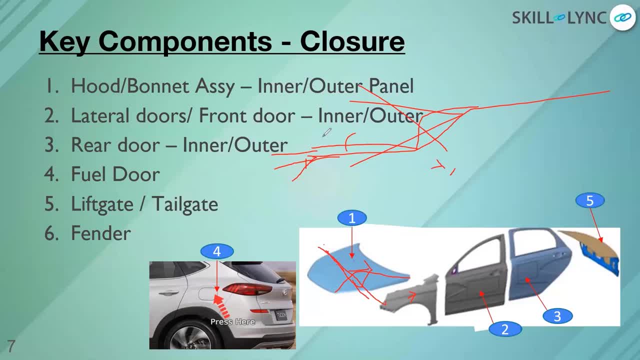 like this: okay, so that, uh, this complete hood assembly should not bend and go into this passenger zone. okay, suppose this is uh. okay, suppose this is my car. okay, this is my car and this is my hood. okay, so, if suppose the crash will happen, and, and with any pulse, if this goes back in here, 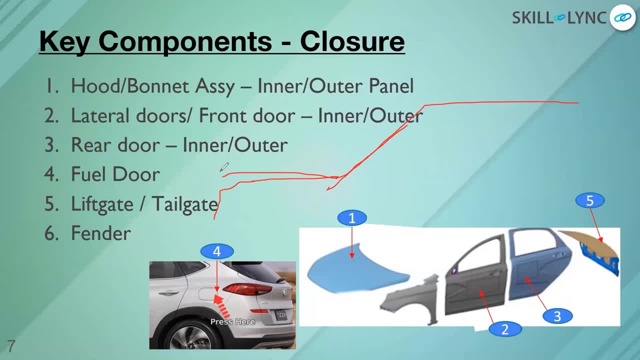 and we hit the windshield and all or go inside. but what we do as a designer, we give a compel zone in here so that whenever the crash happen and this engage, it will not break everything on the vehicle of the hood. okay, these areas and all. so what it will do, it will break in this area as we plan. 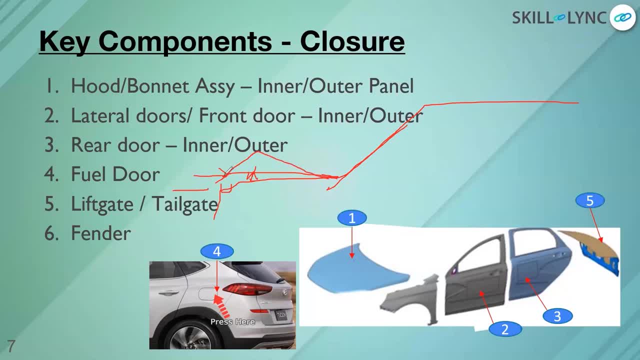 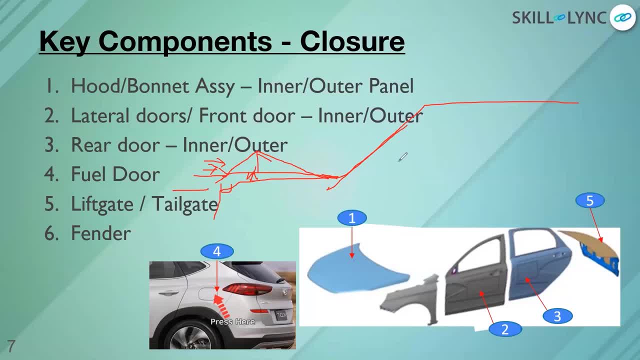 of the uh hood, okay, so that it won't go back and uh hit anywhere of the zone and it won't absorb the load. then all the load will be absorbed by the underbody, okay. so that is the second area where program deformation in the vehicle. okay, what, who in doors we have for frontal crash? because, as we 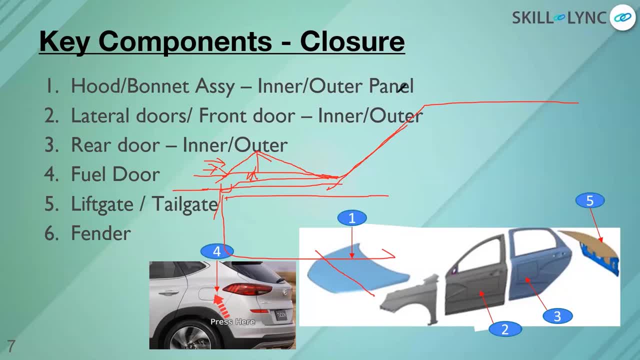 know the load is traveling from here front. okay, i will color it from with different color. okay, yellow. suppose the load is coming like this and from here it has to transfer in all part of the vehicle. okay, we have b pillar here. okay, we have a pillar here. we have cantilever here and we have the. 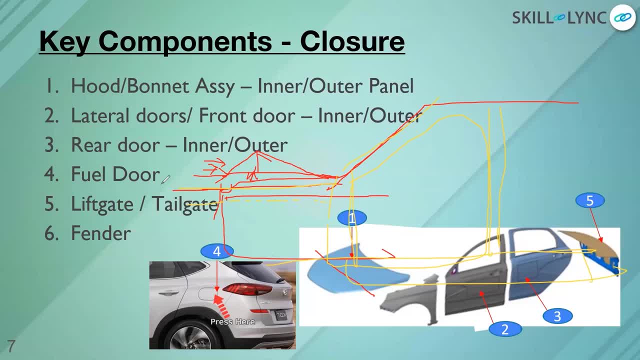 bottom seal here. okay, so when the load is coming, the first point of contact is from this area, the side member, and this side member. from the center it takes it till the rear of the car, but from here, from the side end of the car, it transfer it from here top, from here it goes down. 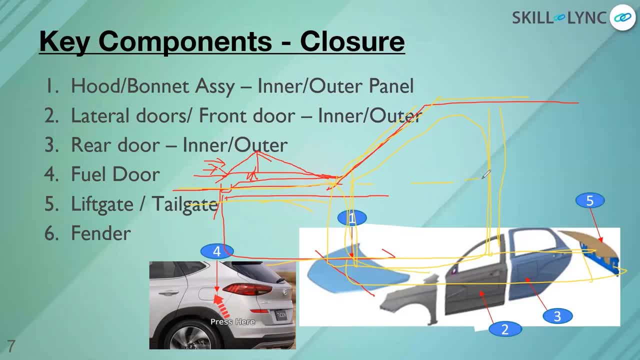 and from a pillar to b pillar. we have one skirt. we call it skirt or stiffener rod in the door. okay, inside somewhere here. okay what it do, do it like it takes all the energy and transfer it to b pillar and from b pillar. we have the same kind of rod in here which transfer it from b pillar to 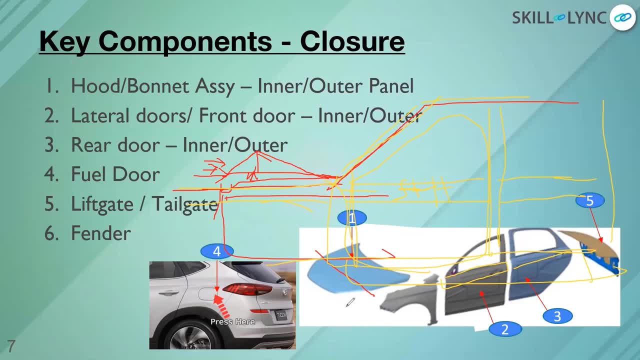 c pillar. so that is how the load is being transferred from front to the end of the car with the help of this kind of designs. okay, similarly, we will be having one more rod. we call this uh g bar or anti-intrusion beam. so it is also like this in here, so that whenever the impact is coming from, 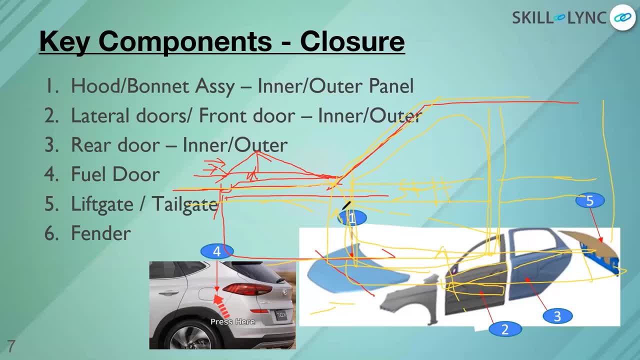 the front. all the load will be going in front c a pillar and the b pillar of the car. okay, not inside the passenger passenger area. so that is how this door panels comes into play. rear gate tailgate is important. uh, now we have lot of crash regulations coming for rear, also china and usa, and 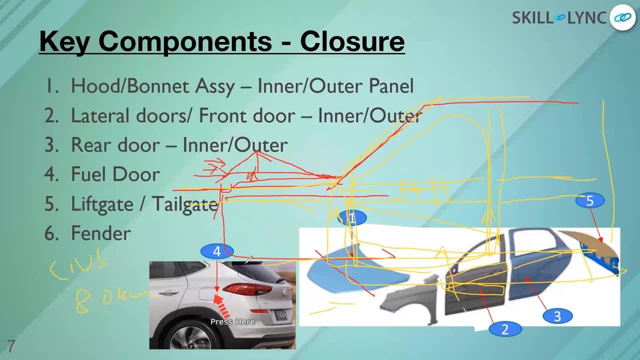 have a rear crash with atk mph speed. okay, so in that area also, the criterias are: this: should not break and grow inside. okay, so that the designs are very much robust in this areas. okay, so this is all about the closers assembly. if anyone have any doubt related to closer can ask me. 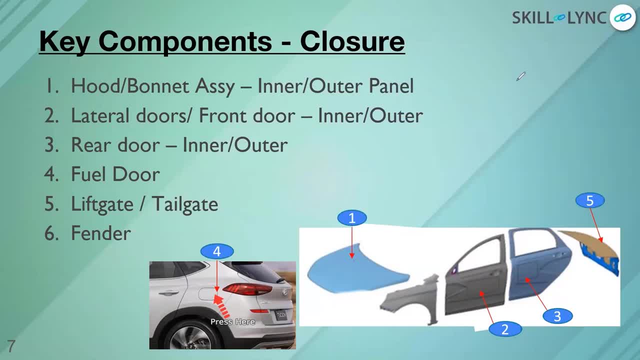 now only related to closer. somebody is asking which type of sensors used for uh, to know if you close and open of the door. it's a touch sensor and the impact sensor. we have it okay, and that is on and off sensor. it's not a huge sensor and it's a very less. 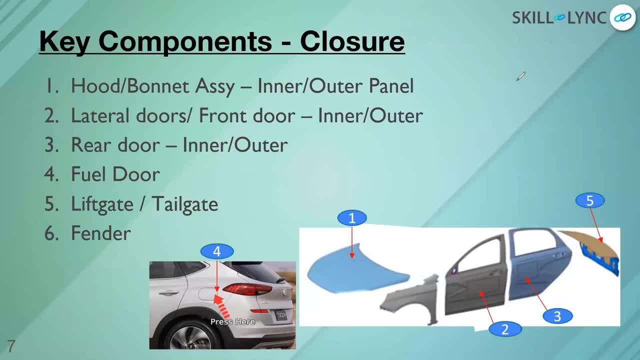 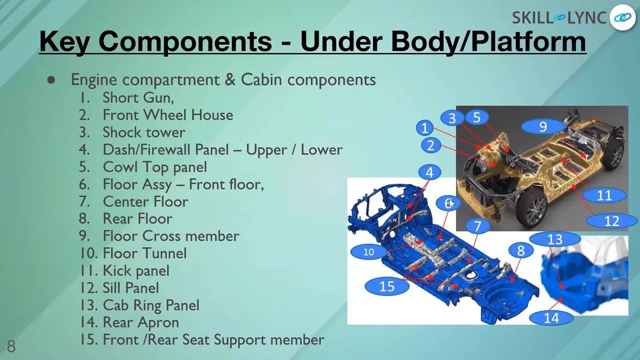 cost sensors. okay, no doubt, what is fender? I have already explained you what is fender. this component, we call it fender. so you want to know more about fender? okay, so the fender. okay, see why the fender is bolted: because in underbody. okay, if you can see. okay, so this. 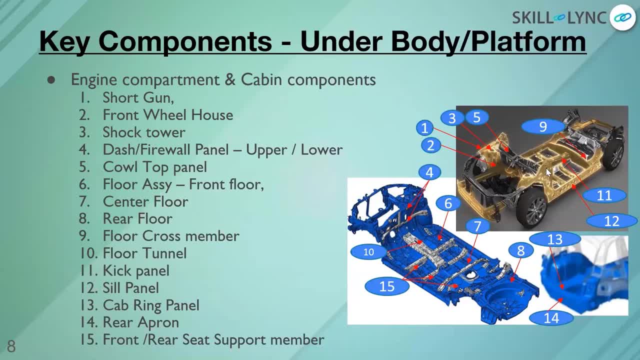 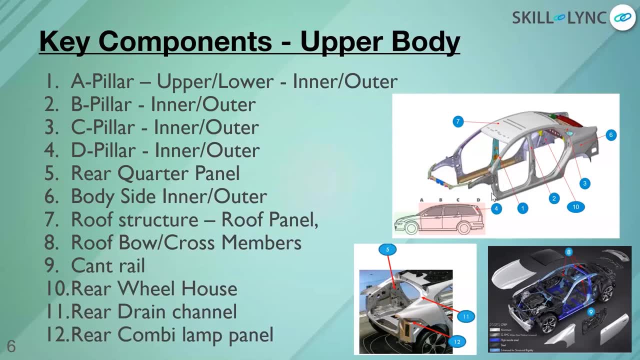 is the skeleton of the bottom, skeleton of the body. okay, this will come, and then upper body will come. and then fender is been mounted half in here and half in underbody. it is bolted in here as well and in upper body as well, so we can't bring that fender with any of. 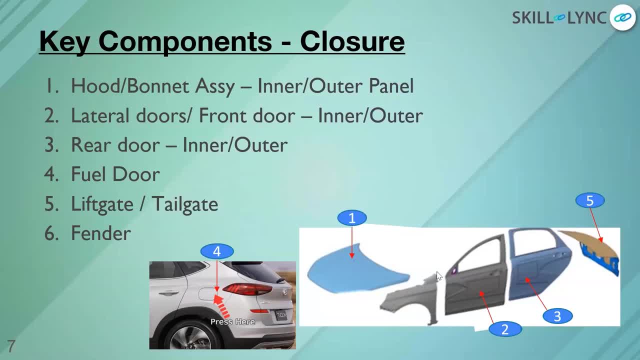 this component. Okay, so that's the reason we can't weld it with some area, so that we have to weld it in again different area. so we put this fender always as a bolted object. and the second thing is, whenever the crash happens, folder this fender gets deformed very easily, if it will. 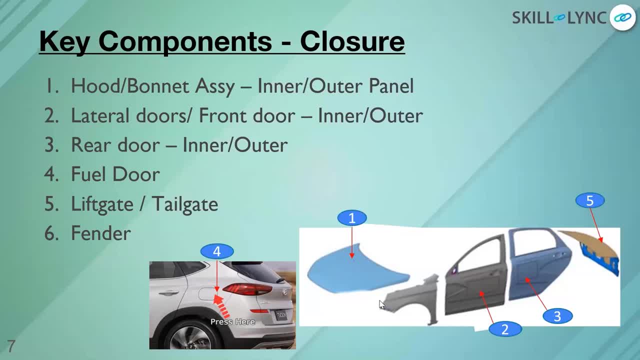 be welded. it is very expensive, it's an expensive process to like repair it. but if it is bolted you can easily unbolt it And you can repair it okay. and third thing is it is not a load carrying object, okay. only purpose of this fender is for styling and for the wheel aperture. like wheel should come. 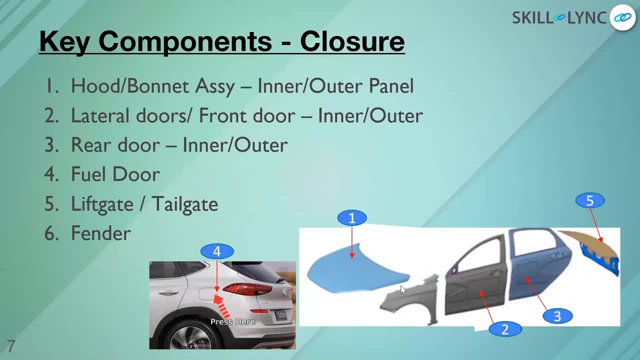 in and come out. that is the only thing. we need it for fender, okay, so we. we don't need it to be very constrained, lot of constraint manner, we don't need it. so we don't need any welding and all in here, it's just a one component. 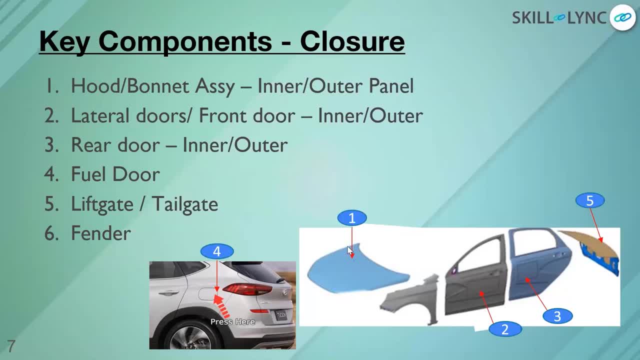 We even don't have fender. Okay, For hood we have a hood reinforcer inside. for door also we have a door reinforcement inside. tailgate also we have an enforcer. but for fender we don't have an import. even for trunks also we need, we have an all because this. we don't need any statical stiffness. 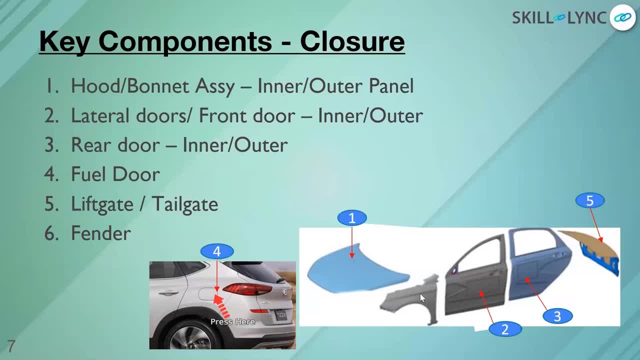 of this component. we don't need any internal stiffener or internal components in this area. okay, So I guess it is clear what could be the generic design tolerance limit for these parts. So tolerance of these parts. again, for the surface tolerance, we always use monon more. 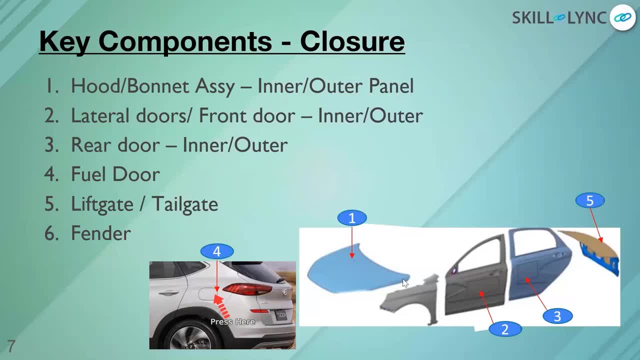 than 0.5 mm. okay, for the edge tolerance. it should not be more than 0.1 mm. okay, for the holes and all it is. we have a general tolerance for all the kind of hole standards. okay, only for surface and the lines. I have already told you what is the tolerance level we maintain. okay, which previous picture. 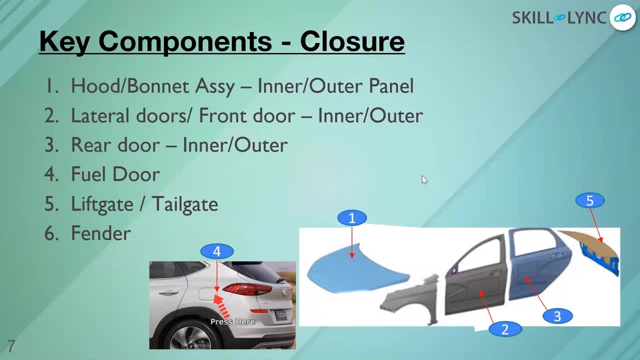 we don't have rear side fender in car, okay, So fuel door, it's a component, like we have this fuel door with a inner reinforcement and the hinge assembly. We always have a positive locking in here which locks and unlocks with the sensor. So the fuel, the gap and flush at the fuel lead is not there. 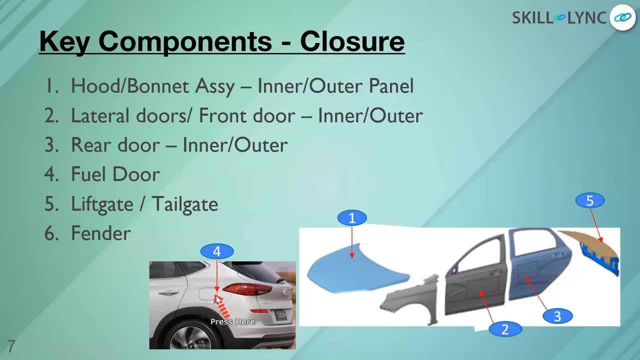 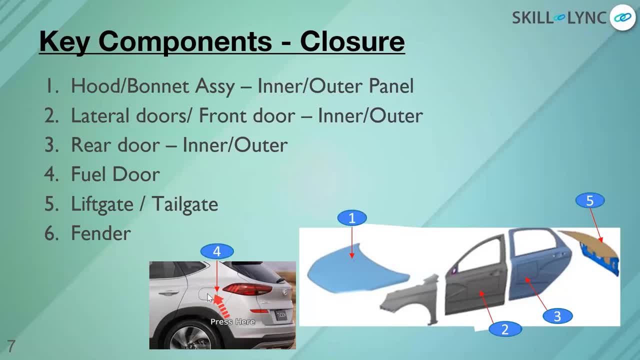 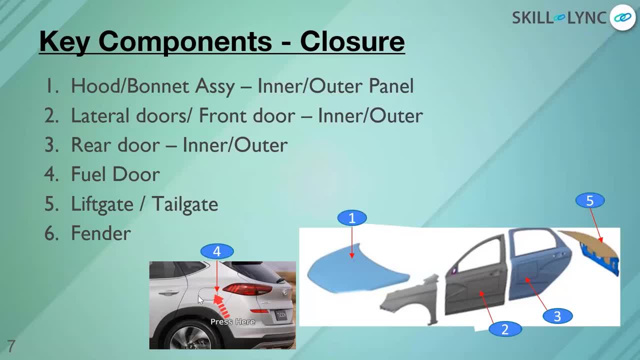 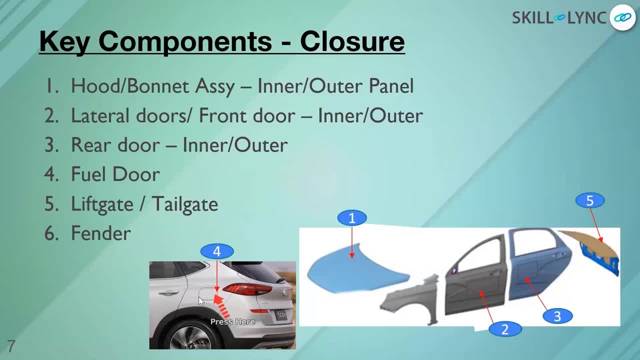 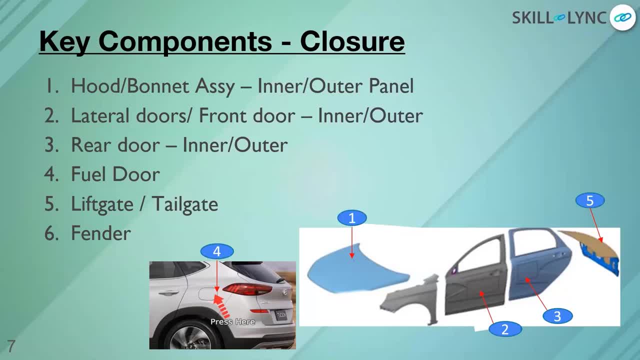 So the gap and flush at the fuel lead is not there. different sizing or different flushing in this area, so this area is very much critical. second important aspect in fuel door is like it should always flush with the outer panel so that the aerodynamical drag should not affect this zone. okay, so that is the reason this is a very important. 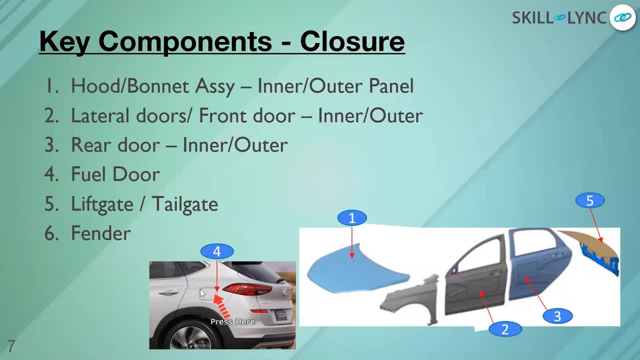 aspect of the car. okay, uh, the water should not get stick here because we have unprotected zone inside which get rusted if it is, uh, not well designed. okay, so this is how. so what is gap and flush? i can explain you. those area, okay, suppose, uh, this is door, okay, it's a bso and this is a fuel trunk, okay, 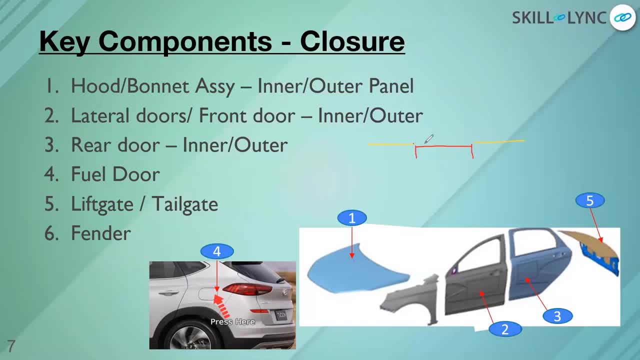 so we always maintain a negative flow flush. what is negative flush of 0.5 mm means this body side outer component will be in higher side in the and this one is always in the negative side, so that whenever the water comes from here, it it should not enter in here. from here it goes and here it comes out, so it is sometime also. 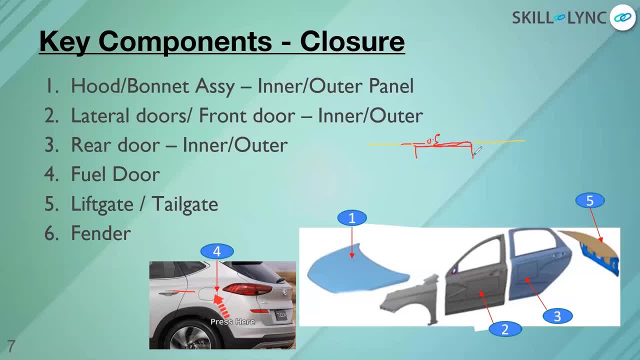 tilted in this manner: this one. okay. so how? it has been? from here minus 0.5 and here it is plus 0.5. okay, sorry, 0.5, so that whatever the water comes from here comes here and goes here. okay, so this is sometime. we always maintain zero, zero type of plus, but that is not possible, so we always 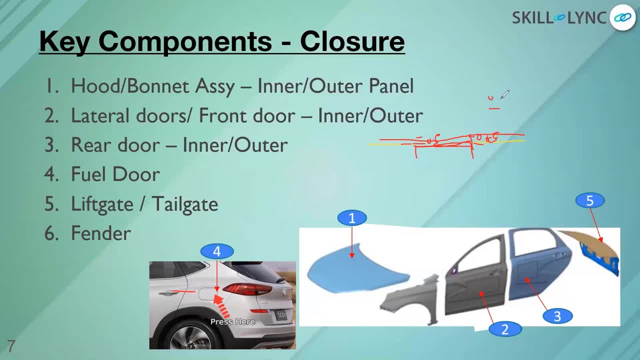 keep a tolerance of- uh mine, zero two minus uh point five, zero point five. okay, not more than that. that is the tolerance limit we maintain in this kind of zones. so, uh, this is all about closers, so we will move to our next area, that is underbody. okay, uh, anyone, if anyone have any? 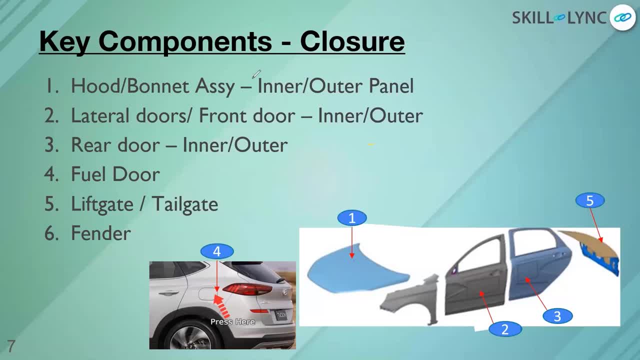 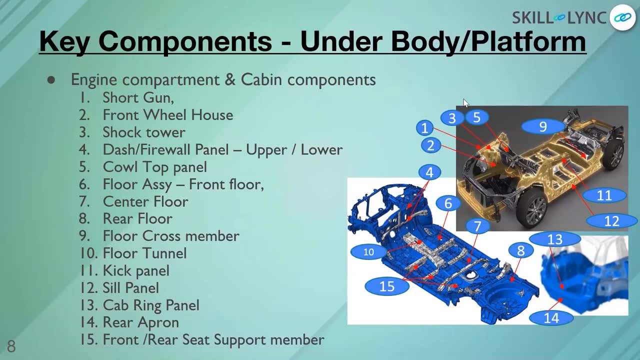 doubt. they can ask me, or we'll move to the next area. we have any question, mr clear. thank you, i will answer these kinds of questions later or after the training has been done. okay, uh, forces act on closers. okay, what is the aerodynamical forces? acts uh on the closer while moving? uh. 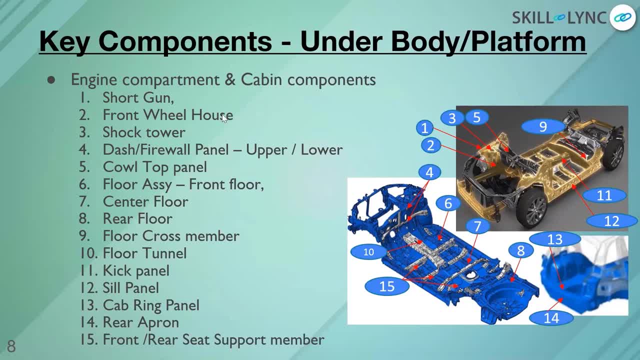 when the component is moving, when we have a uh, when we are closing the component, we have a force, the like closing force and opening for uh closing efforts. okay, when we drop our uh, uh like food from, uh, when we unlock it and drop, those are the forces acting on closers, uh, those kind and the 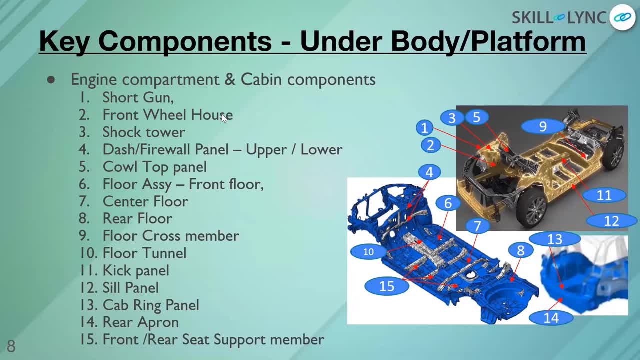 in static condition, these are the forces. and when in dynamic condition, aerodynamic is the only you uh thing, and sometimes, if it rains- and those are the forces, which is acting on closers defining fender. you showed one diagram, okay. okay, we have been talking about underbody, so this is the main. 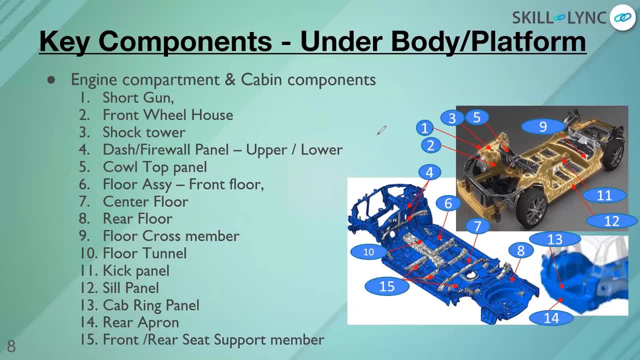 area of uh vehicle which is not related to the styling of the vehicle, which is related to the performance of the week, okay, why? because all the crash loads have to be absorbed from in underbody, okay, and all the things like the vehicle. uh, the seat mounting also is in the underbody, okay. so 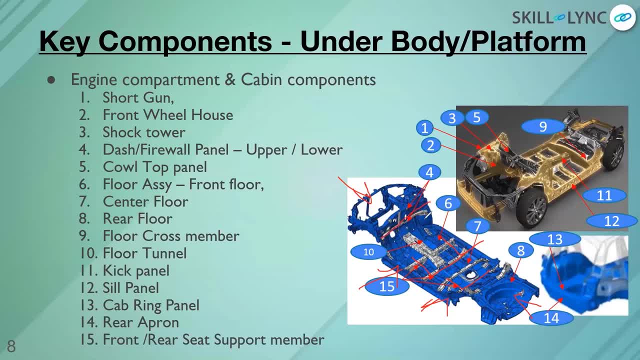 related to any safety. all the, even the steering wheels, everything has been mounted in underbody part of the car and it is the only component. it is the only area which have more number of component than any of the other areas. okay, it have something somewhere around 120 to 140 components. 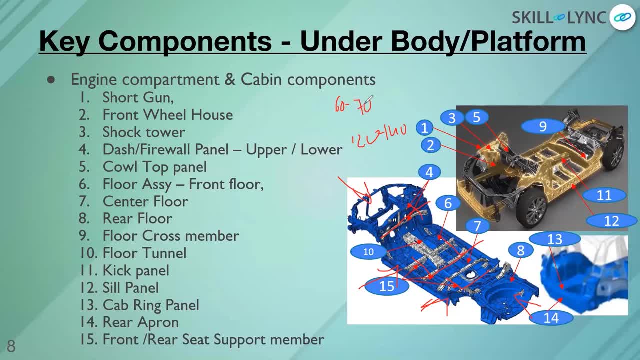 wherein others it have, and 60 to 70 component in uh uh like uh- upper body and 40 to 50 component in closer, okay, but in underbody we have 120 to 140 components okay. so there are huge components and a huge parts also. 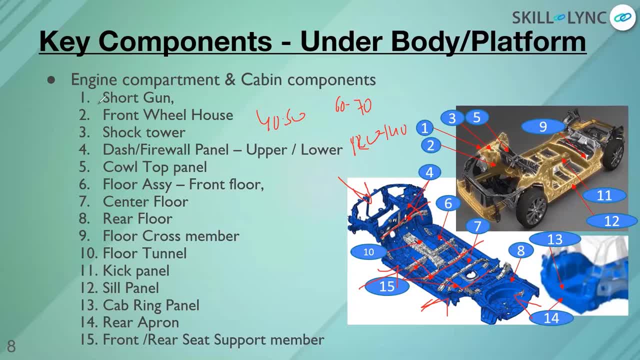 which is being used in underbody. so i have just shown, like, for what all are the 15 areas. we have shotgun, which is here, which comes from a pillar, okay. which takes the load, uh for uh. which takes the load to the side of the vehicles, okay. the uh bot, uh like uh. this area, the front, uh, this. 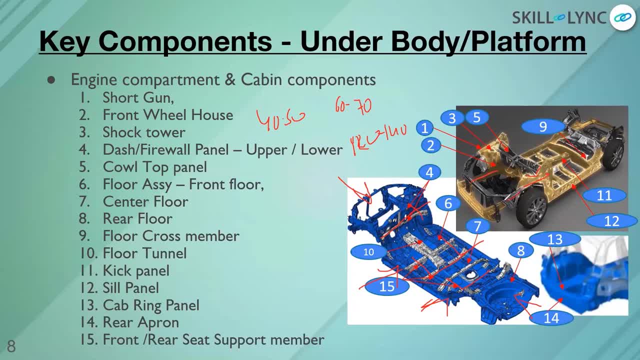 area uh, front wheel house and the bottom traverse. member. this takes a load to the bottom part of the vehicle and shotgun takes the load to the sides of the vehicle, okay. second is front wheel housing. okay, this is the front wheel housing. below this we have our wheels, okay. third is a suspension tower. 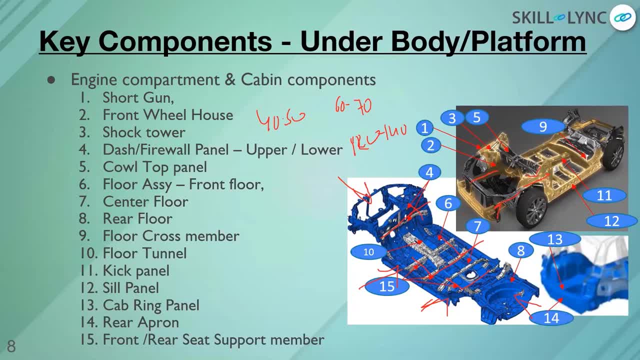 shock tower- we call it in automotive also, so that all the load will be. this is a very uh robust area because lot of loads of the suspension will be coming on this area for this dash and firewall. that is this area which you can see. so dash is a one of the biggest component in uh underbody. 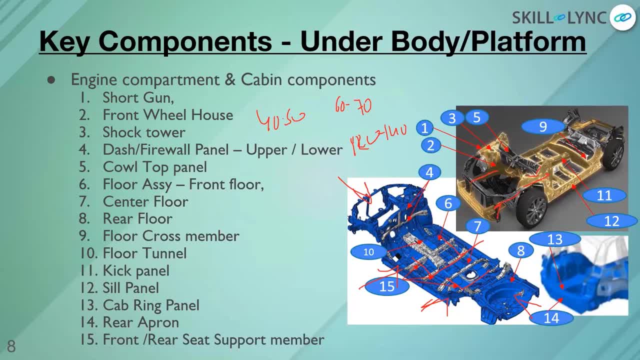 because it have lot of mounting. it have mountings for your ccb is like cross carbine, where all your dashboard, uh, your steering column, everything will be a bolted steering is been bolted to a, to a pillar and then inside in the dashboard, all your uh like brake booster, uh pedals. 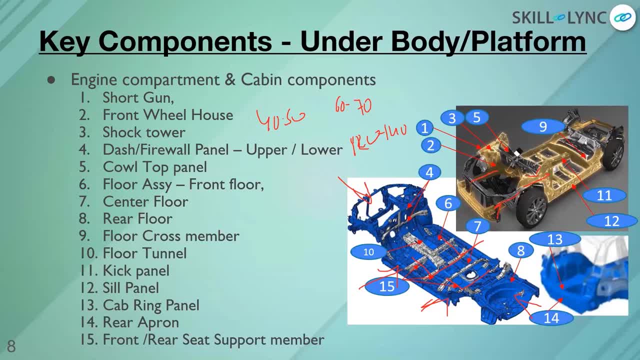 everything will be. it is mounted in uh cp, uh like ccb, and the passing is been gone through dash panel. okay, steering, uh passing is also going through dash panel. it is also a healing� chamber heat shield because it won't allow the heat coming from engine to the compartment zone. 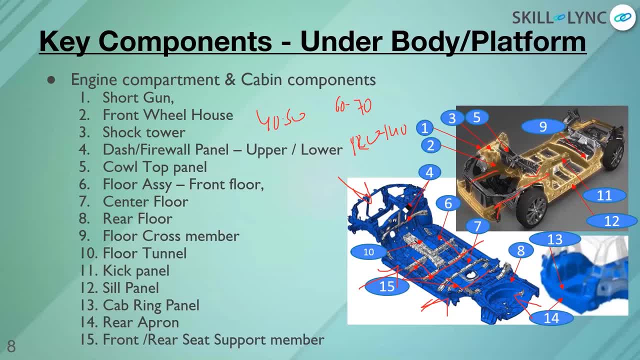 okay, it also have our refrigeration unit coming into from here and mounted in here. okay, so that is all about dash panel. call it up panel is uh here, uh, where we used to uh like. uh, the call it up panel is here, yes, because it is also the water box area. and call it up, we call it because the 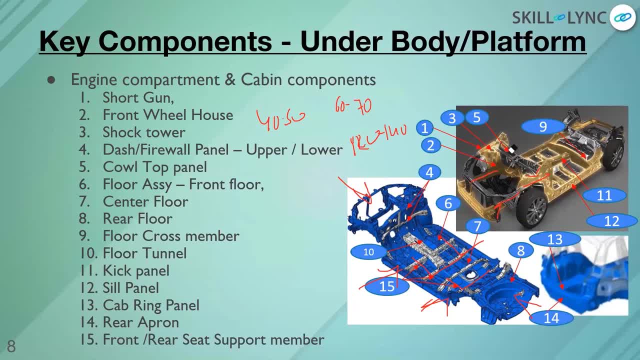 like, the windshield has been placed in this area, okay, and even the whatever, whatever water is coming from the windshield is getting collected in here and going out of the vehicle, okay, so this is all about, uh, a power top. this is how the water flows out of the vehicle. we have a hole over here. 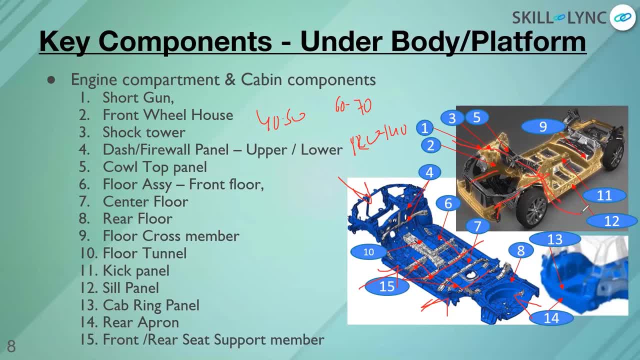 so that the water will be coming out from the bottom um outside of the car. okay, so sixth part is the floor assembly. floor assembly doesn't have any loads, so we put it in a very lesser thickness of 0.6 mm. it always only carry the load of leg and 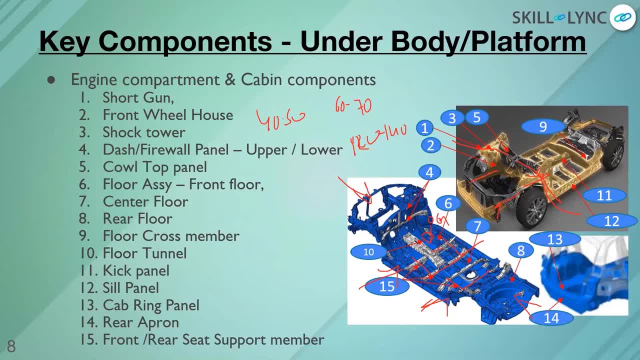 other things. otherwise all the load will be taken by this member, cross member, where the seat has been welded. okay, so this is a stiff area, this one is a stiff area and this side is a stiff area and in between, where we using our sheet panel. those are not a very much higher, stiffener, stiff train. okay, 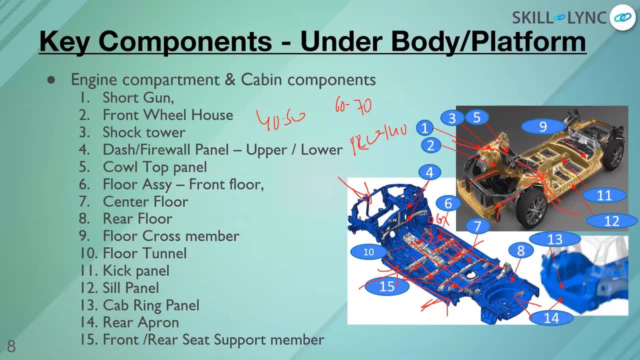 so this is about floor assembly: central floor, center floor is also here. uh, rear floor is somewhere here. okay, this one. okay here. we used to put our uh okay first. i will clear: okay, this is the central floor zone. okay, this one, this is the rear floor zone. okay, so this even protect the 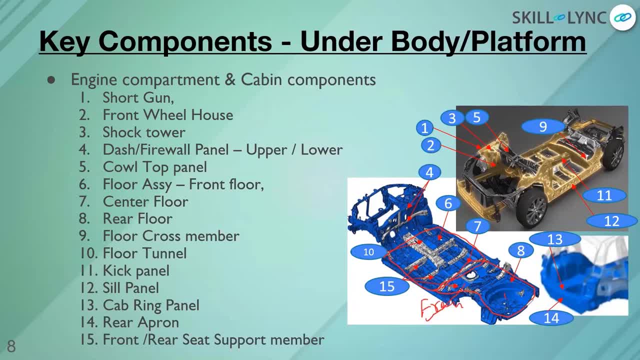 fuel tank from the top, okay, and this one have spare wheel inside the vehicle, okay. so we have both kind of provision inside the car so that whenever the the fuel should not come inside the cabin compartment zone, and this wheel and in for this wheel. there are two types of provisions. it 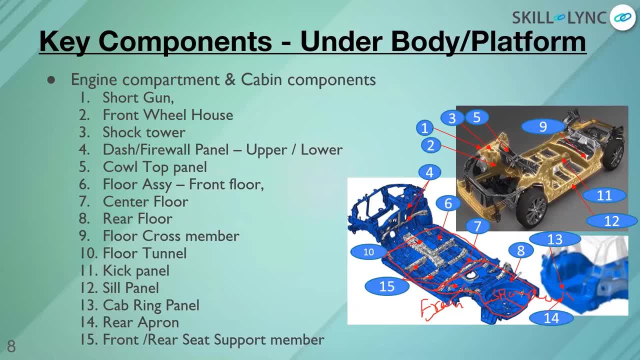 should it? sometimes it comes inside the car and sometimes it called bottom part of the car. okay, that depends if we have- uh suppose you will take examples of duster and all- we don't have it in here. we have it in the bottom part of the area. but if you will take any sedan car, we have it inside in here in hatchback cars. 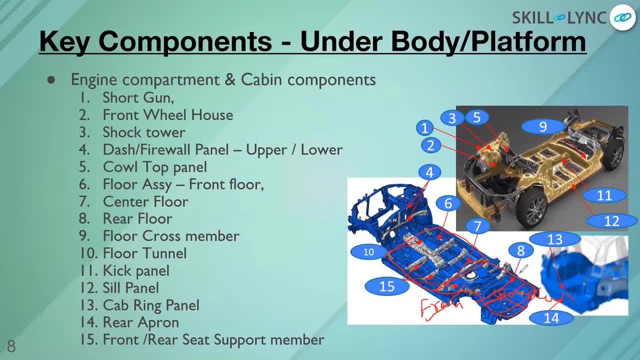 also. we have it in some time. we have it for suvs also. okay. so that is again a strategy for companies, like how they want to provide and where they want to provide the spare wheels, okay. so floor cross members: are these kind of members where our uh sheet is getting? 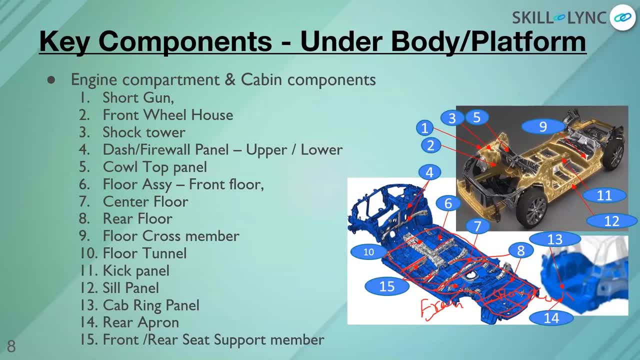 bolted, so seat is getting bolted in here. here. that is for the left uh seat. okay, here and here. that is for the right seat. and here from this zone to this zone. this is for the rear seat bench. okay, this is how the seat has been mounted. uh, we have a time constraint so i can't show you. 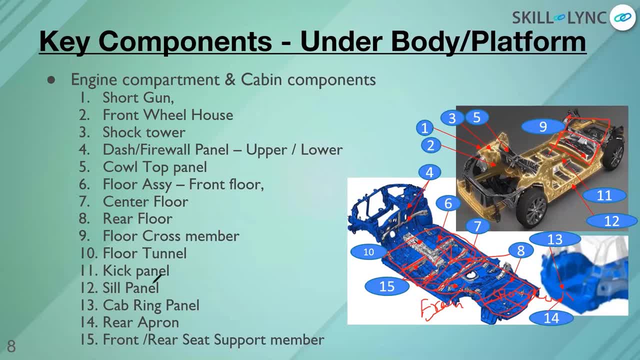 exactly where and where. so, uh, i'll show you later. okay, floor tunnel why we have a floor tunnel so that the four by four uh rod and four uh and four by two- four uh like soft drive soft- can pass it from here. at the same time, for four by two, the exhaust in four by four drives out as well as. 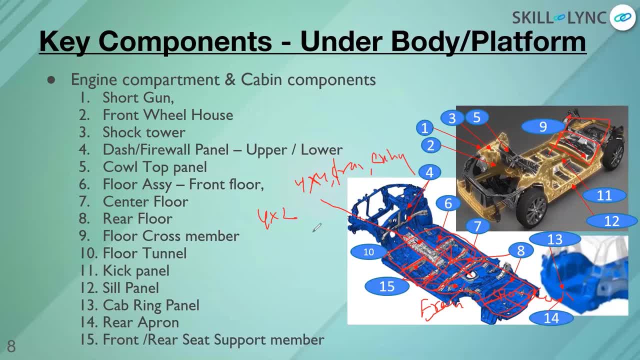 the exhaust line should pass from here and four by two, like, uh, two wheel drive, this will pass only the exhaust line, okay, so that is why we have this tunnel, uh, over here, okay, uh, then we have a kicker panel here. because why we call it a kicker panel? because below this, after this, we have a fuel tank. 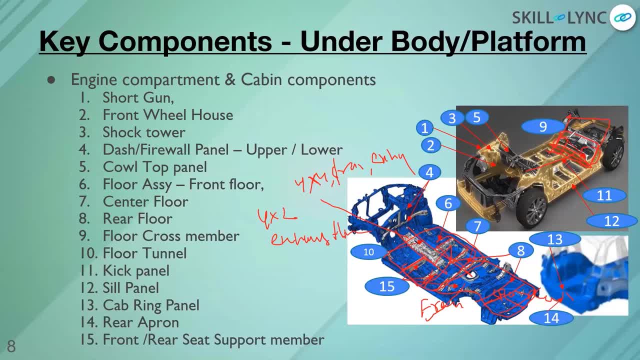 or the battery in the new generation car. we put it in here and the leg should not go below this, uh, behind this zone. okay, that's why we- uh, we keep it as we say- is a kickoff panel. okay, okay, so that the lag leg of the rear passenger should not go below this line. okay, so that is. 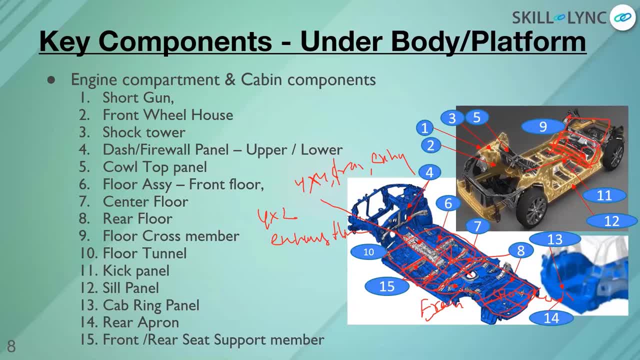 about, uh, this zone. then we have seal panel. that are the two uh stronger line of, uh stiffener going from the side component of the car, like this one, and that side also. it travels from here to up to the end of the car. okay, cab ring panel is again the same one. 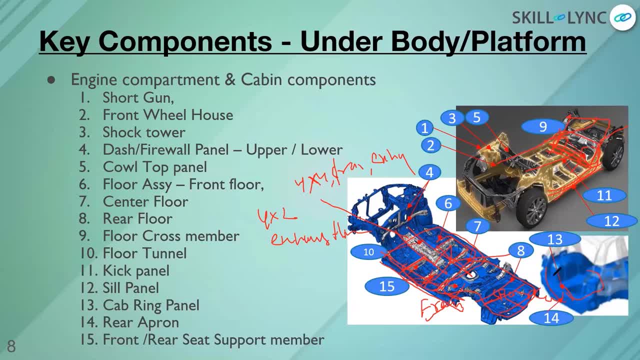 here what i have explained you. rear apron is one where the tailgate comes and get fitted okay. so we have that apron, so where, uh, the lock of the tail there has been getting engaged okay. and then front rear seat: support member. so for uh seat. we used to have the support members, so for that. 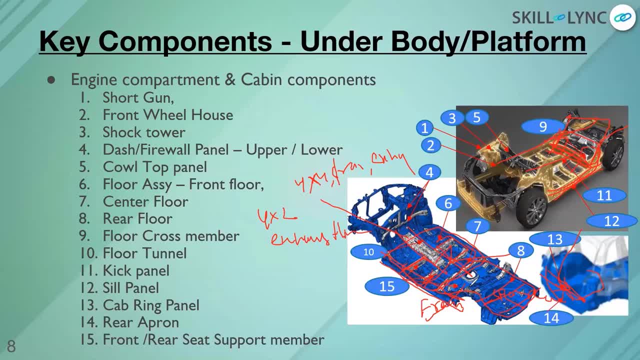 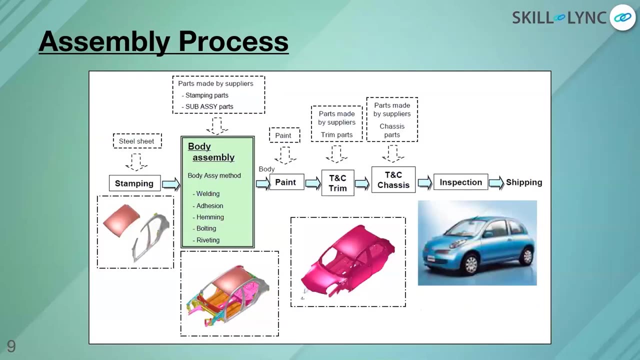 we. we have one extra brackets in those areas. okay, so that is all about uh components in biw. so till now, if you have any doubts, we i'll i'm happy to clear you and then we will go to the different zone. okay, that is how the assembly process has been done and how the 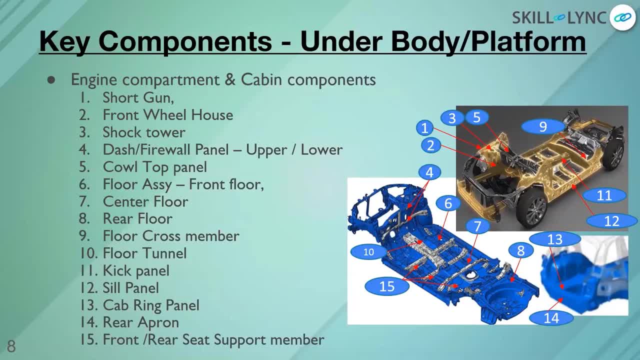 other. so till now, if you have any question, you can ask. yes, powertrain comes under underbody. do design changes according to material? yes, it does change. explain on tailgate and that is already considered. explained clear. okay, great, yes, it's a. it's a huge area. 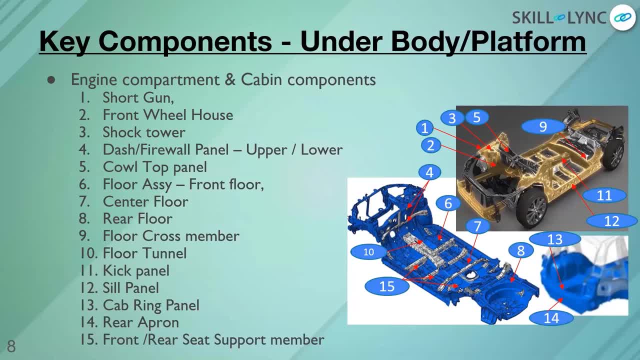 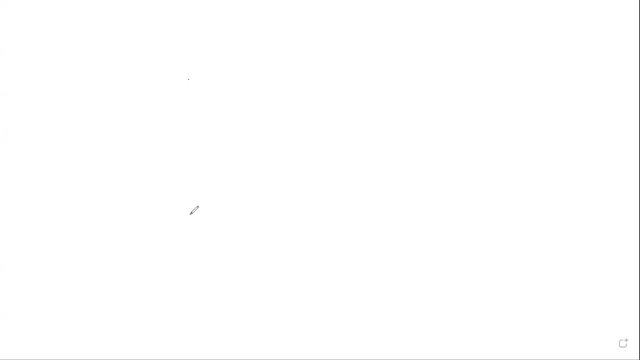 uh, so, yes, okay, somebody has asked me about shotgun. okay, define and rear another. so what is shotgun? suppose, if i will? uh, okay, you can see my white board. can somebody answer? so suppose, uh, this is the uh structure of the card. okay, so this is two cross members of the cars. okay, which is going till the rear end of the vehicle. 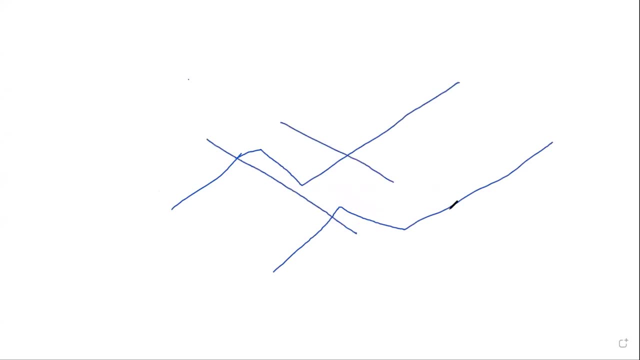 okay, so this is the center part of the vehicle. okay, suppose i am explaining in that way. okay, so this is about the, the center load. so this is the first part which takes all the load from the week. uh, the impact from the front. okay, it even have the engine mounted in these two blocks also. 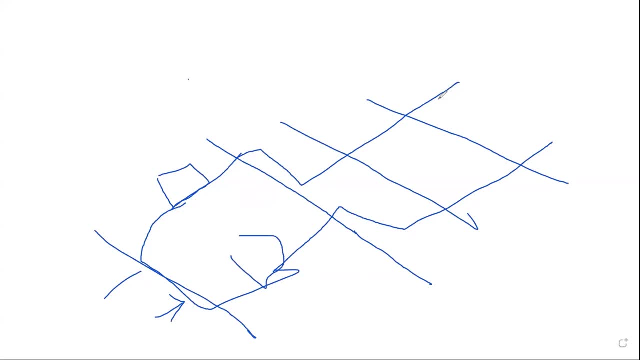 only so what? uh, the underbody is fully designed, as for the, for the crash, but upper body doesn't. uh is not been designed more into crash, so but it should also absorb the energy. so what we have done? we have used a second member, okay, which will also absorb the crash one. when, once this 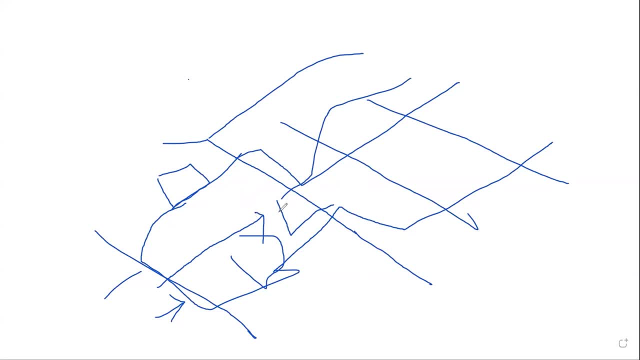 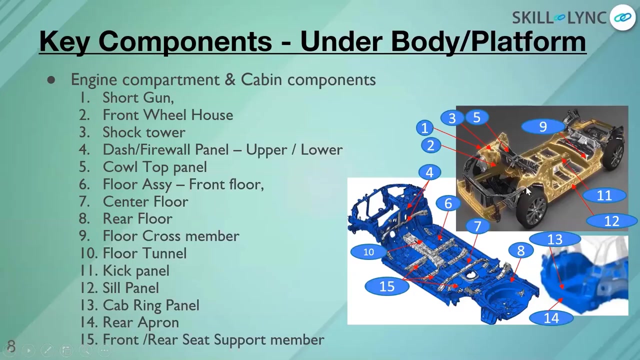 fails up to this area, okay, then only this member will start absorbing. okay, so when the second absorbing area, we call it shotgun. okay, so if i'll explain in here so you can see this golden part from where it's starting. okay, so this is from here, the second uh load impact will be absorbed. that that will be absorbed to upper body. 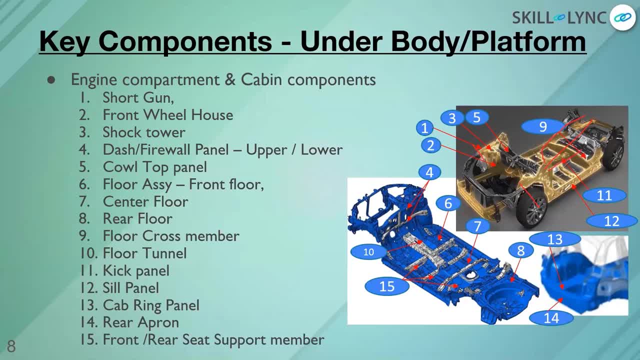 okay, uh, center area and the side of the car. but this one, these golden areas, this one, this will absorb the first load of the impact, okay, and will transfer to this till this areas in the center way. this goes from bottom till here, okay, so this shotgun is here, is to deliver the force. 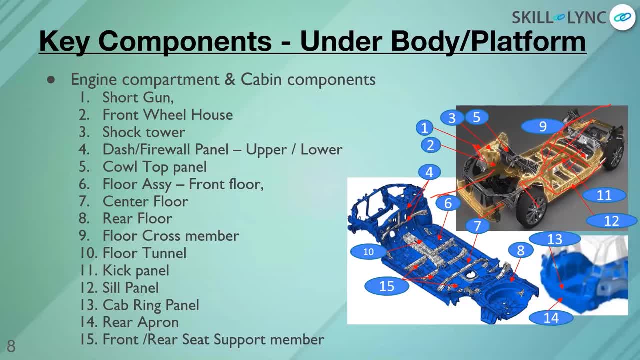 from here to the top of the car, to the bottom of the car and to the center of the car. that is why we uh this uh shotgun, okay. second is apron. what is apron is like we, it is a rear uh uh filler in this area. suppose here we don't have any apron, but in here we have an apron. okay, what will happen? 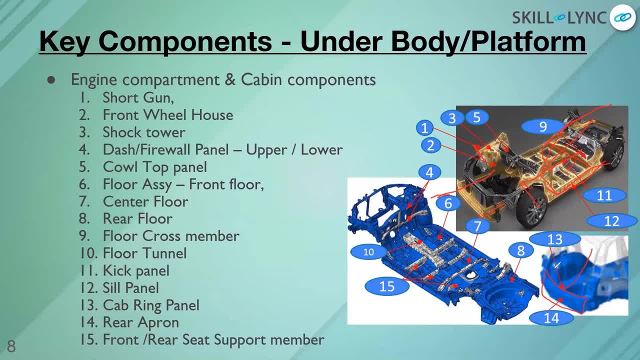 you, you, whenever you will open your tailgate, you will see one panel, okay, in which there is a gap where the latch is there- okay, which will get- and hooked- uh, which will get hooked with the tailgate, okay, so that latch should get locked, okay with this area. so for that purpose we use 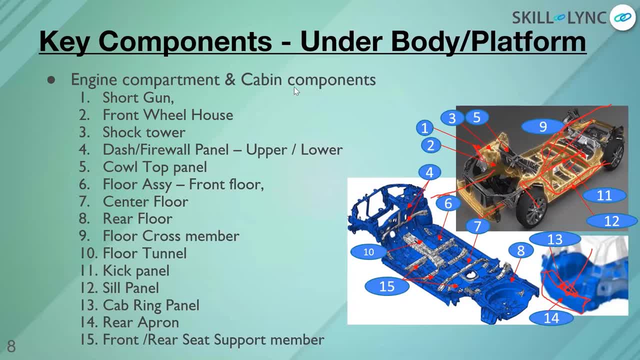 the rear apron. okay, i hope it is clear. clear, the one who have asked about shotgun. and uh, fender, oh, sorry, apron. okay, clear. so kick, kick panel. okay, so you guys are making me revise all this area. okay, okay, kick panel is the one. okay, suppose uh here, if i take a section in this area. 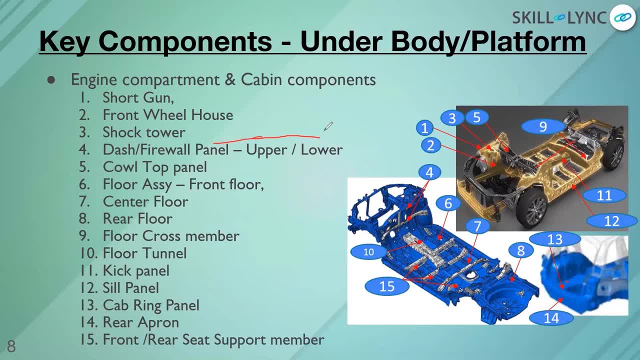 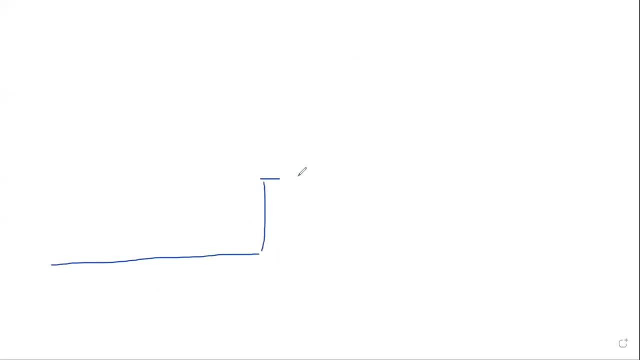 so this is the our base plate of the car and this is the kick panel. i will explain in here, okay. so suppose this is the base, okay, and this is the kick panel and this is how it goes in the vent. our seat has been placed something like this, okay, and the leg is coming here in this way, okay, so this is how. 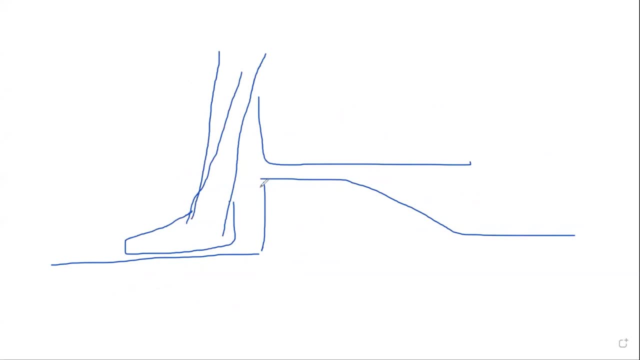 the leg legs. uh, leg has been placed okay. so if a person leg is going below this zone somewhere, suppose the kick panel is not messing with it and it will be here. so what will happen? the person leg can struck and he can fall coming out of the vehicle. so for that reason, what we do? we just have a kick. 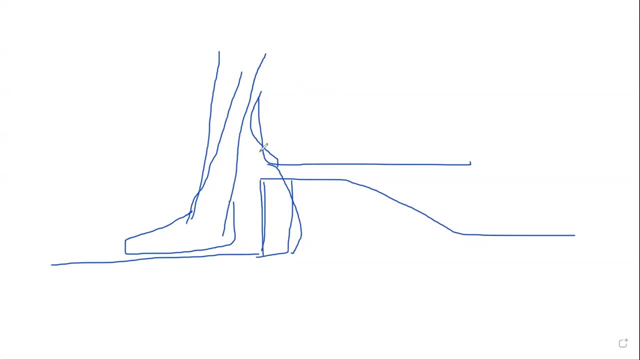 panel in here so that the person leg will not go behind this line. okay, this is the brief explanation of kick panel, so that the whenever it will kick it won't go behind this. it's a human physics we have to understand. okay, so this is a person should not fall when he is coming out of the car. this doesn't. 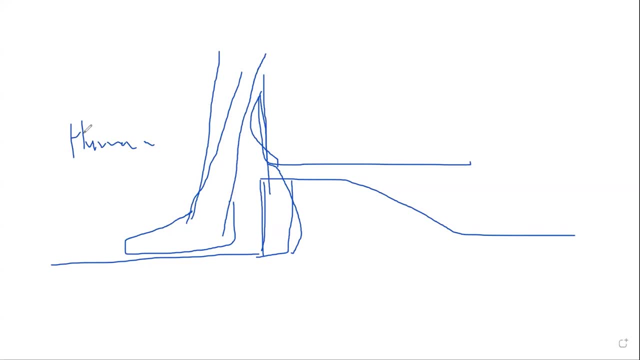 happen for the front passenger, because in front passenger we have lot of space. okay, for the rear passenger we have some space constraint. okay, for that reason, we used to provide this kind of provision. okay, that's the reason we call it kick panel. okay, somebody have asked me about dash area, right? so dash is something like this: is the dash, okay, all. 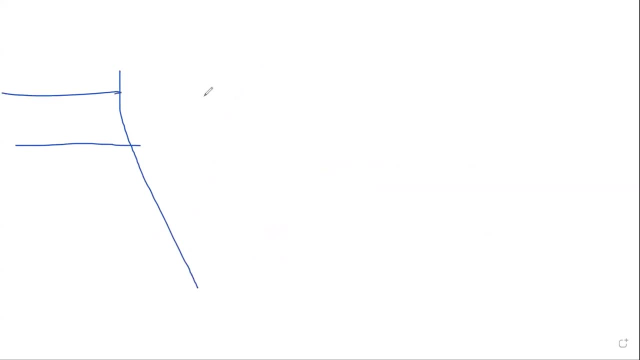 the ac. uh, suppose this are the other rod. okay, this is the steering going inside the dash. this is so all the heat panel. no heat should come inside this. even whatever the load or pointing things, it should not make this dash deform in such a way that it will damage the passenger, so dash is. that's why 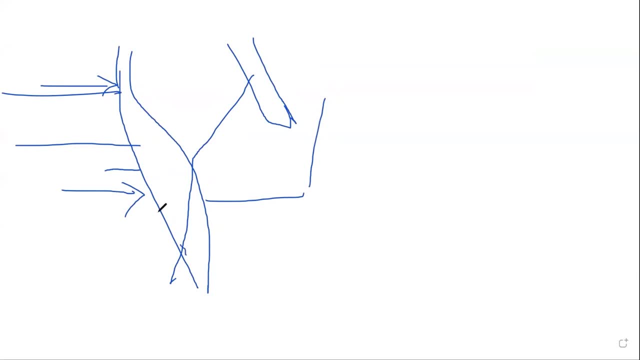 very important aspect and it is very well reinforced in all the area so that the dash inclusion- is the car- will be minimal. okay, it should not be high, it should be always minimal. okay, that is about all this area. so that's it about component of the cars. okay, i don't have 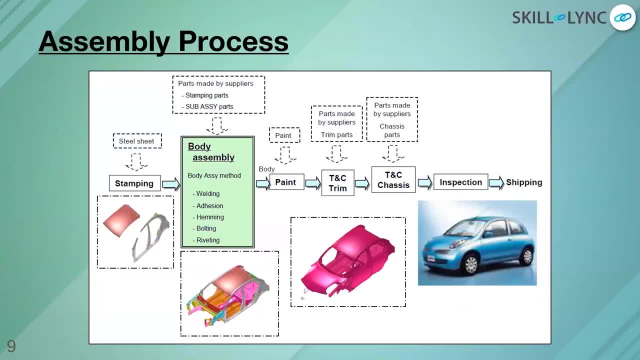 individual pictures right now. okay, so now is we have to understand how is the assembly process inside a company? okay, like how it is been done. so, uh, one is uh, one as area is our body assembly, which i will explain you how it has been done. but before body assembly, all our component is been made from out of sheet metal. okay, so this 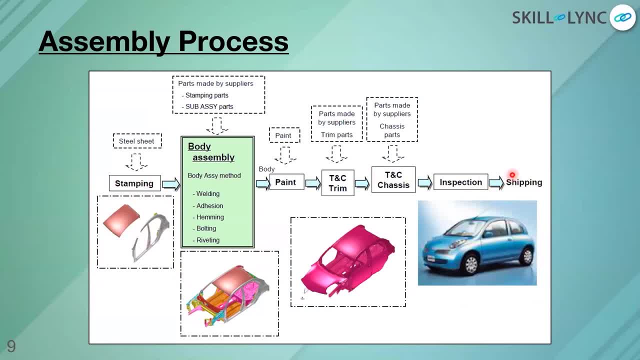 is the uh sequence how a car is been made inside the factory. first a sheet metal will be coming okay, and it will be getting stamped inside the uh uh in in the uh press shop. then that components have been gone is going to body assembly shop, where where we used to weld it all together so to make an assembly okay, then this will call as a body in. 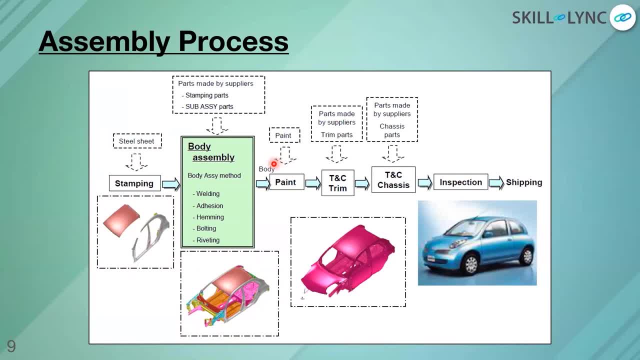 white components. then it will go to paint department. okay, where it will get painted. then trims and chassis area will be coming. okay, where all the plastic trims will be fitted into the vehicle. plastic trims, seat and all things are are been fitted into the vehicles. okay then tnc chassis, where the the bottom chassis parts, uh, the the axles and all. 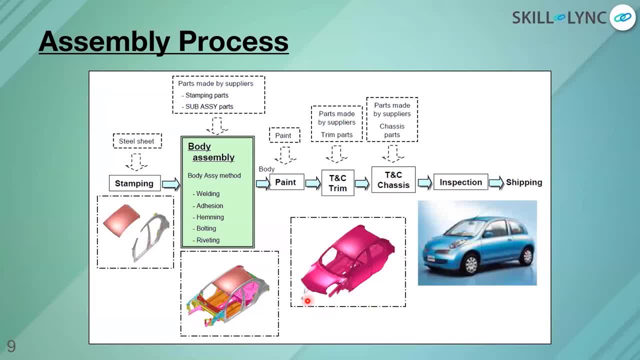 parts have been, uh, bolted together, joined together, and it is also being tested in this zone how the suspension testing, the rolling testing, those kind of tests, not for all the vehicle, for all the vehicle. we will be having that test and we have separate in one stock. we will take out some of 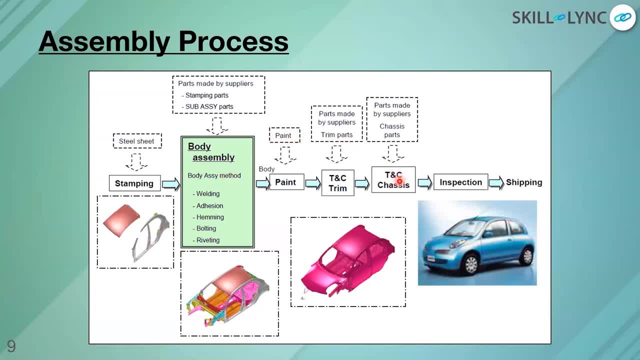 the vehicle and we have a rig test also. okay, we have a small test rig where we will test the vehicle the first go. then we have a inspection area where we inspect, you know, with a lot of quality inspectors which will see all the smaller, smaller defects. if there is any paint defect, 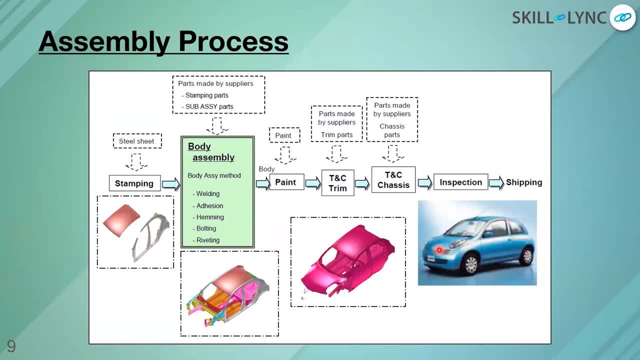 so or any dent on any other panel, the car will get rejected. it will not be getting sim okay. so it should clear all this zone to get sim okay. so this is how the car has been made: first tamping, then the body assembly where all the components 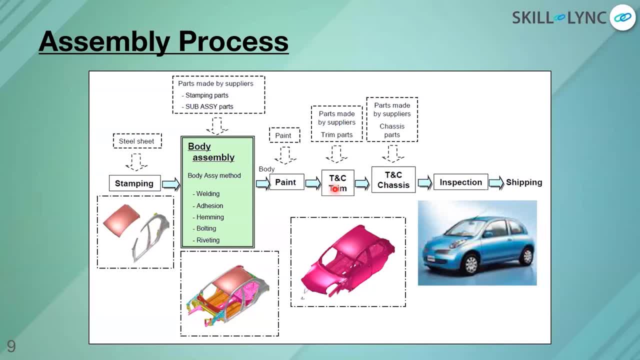 will be bolted and welded, then paint after the paint, all the uh supplied parts like glass, okay, the windows fitments and all uh, the chair seats, all the plastic component mats, roof mats, everything will be fitted. okay then tnc, where the chassis, uh, the engine parts have been fitted, then the 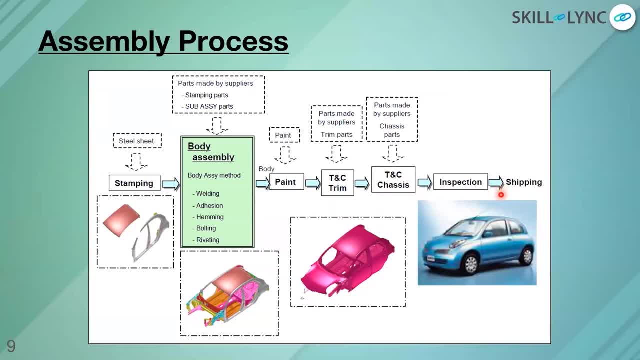 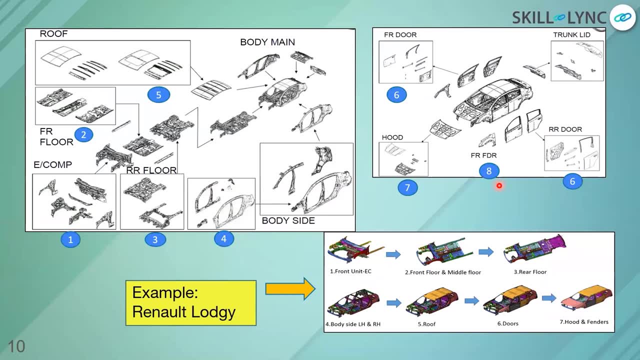 inspection and then the car car is gone for shipping. okay, this is the sequence for, uh, the car to be manufactured, but in the varied shop, how it has been divided. as i have already told you, the component of the car has been divided into three areas: one is underbody, second is closer and third is upper body. okay, so in. 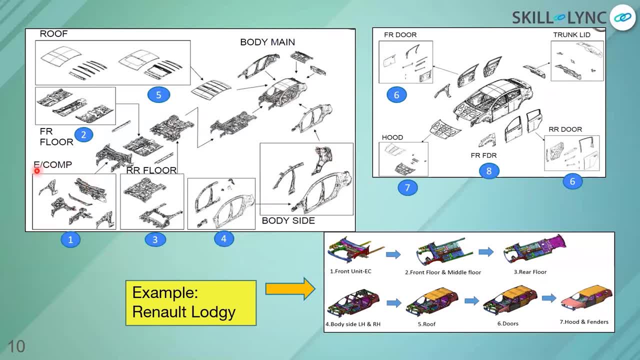 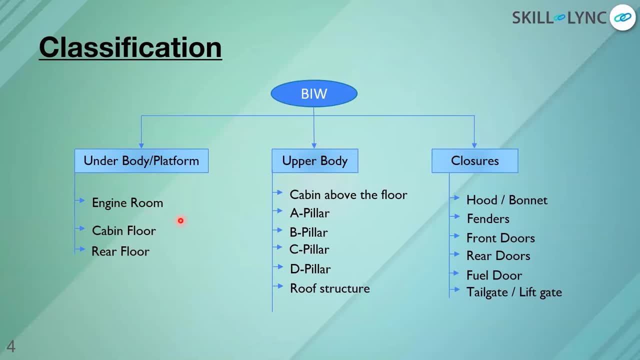 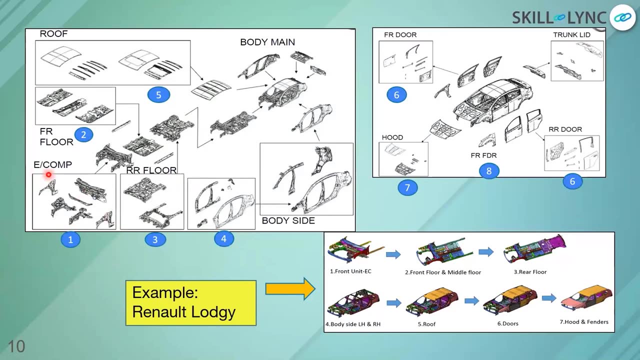 underbody. we have three areas, as i've told you: front area, engine compartment area. if you remember, i've explained in hue in here: engine room, cabin floor and the rear floor. okay, so this is how the assembly looks. okay, so this is the engine area. so this is the complete assembly and these are the 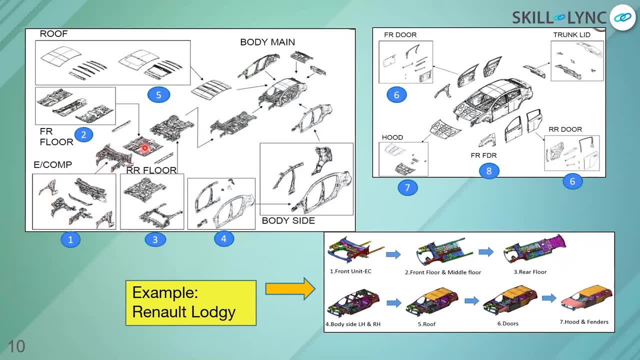 sub assembly which will get welded together to make this. this is the cabin area for the front. this is how it is all together and welded to make this. then this is the rear floor, how it has been welded: skeleton and the surface all together. So this all together, 1,, 2, 3 combine to make a complete underbody. okay. 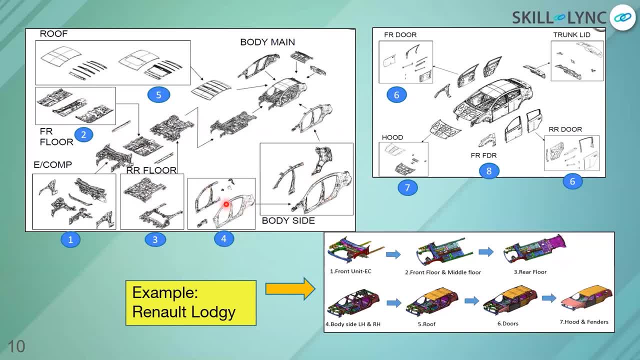 Then we have body side. okay, that is with body side outer, body side inner panel, then quadracore panel. all together when we assemble we make a body side outer assembly. for the side and for the right side is different Roof all together will make an assembly okay, and then the tail all together will make one. 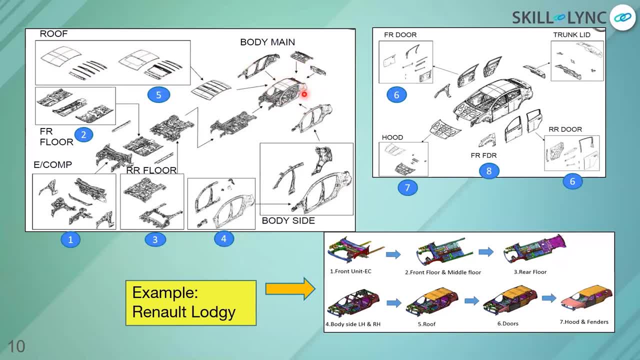 assembly. okay, So all when will fit. it is coming up to this skeleton zone. okay, till this skeleton zone. First is front unit. this is the example of Renault Logi in which I have worked. this is how the front unit will come, then the front and middle, then the rear floor, then 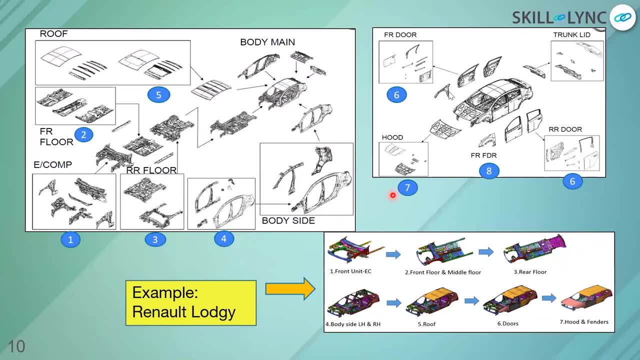 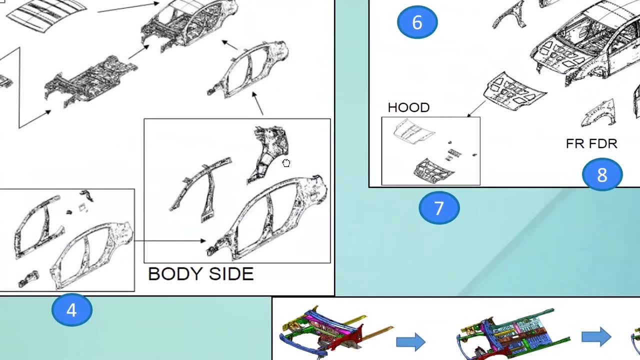 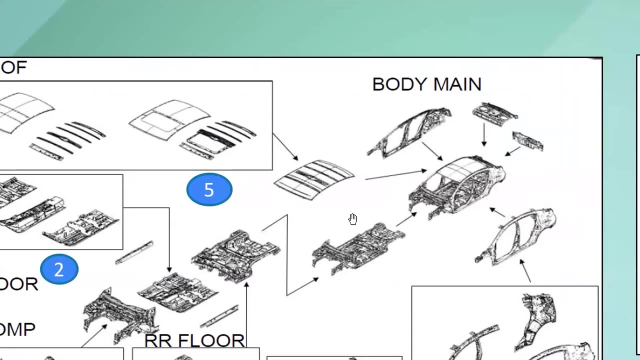 with the side panel if you want, I can, sorry, zoom this area. then the sides, how it is been used. this area is been welded in here and this reinforcement, So it is been welded. okay, all together. then the roof is been bolted or welded whatever. 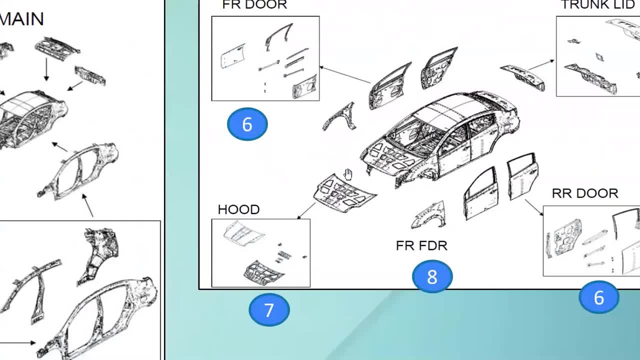 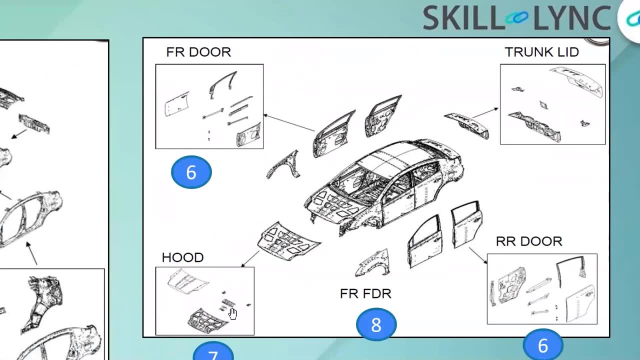 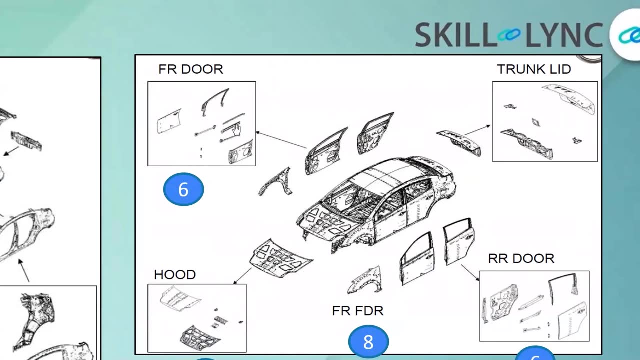 it is okay, and then all the closures coming. So in hood also we have small, small component: hood outer, hood inner and the reinforcements for the latch and the hinges. okay, For door, if you will see front door, we have anti-inclusion beam skirts, front beam outer. 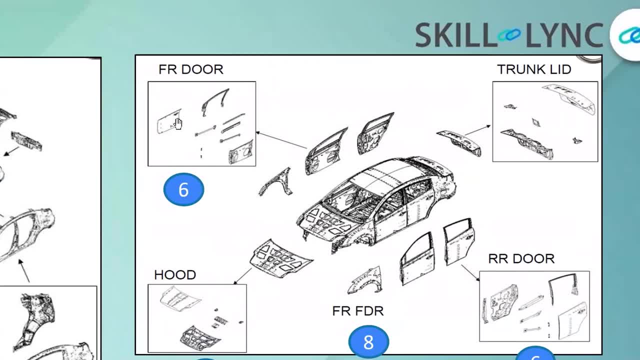 panel, sash type panel, inner panel. all together We make a Body door outer okay. similarly we do the trunk lead with the outer panel and the inner panel reinforcer, with all the hinge reinforcement and the latch reinforcement. So all together when we complete our BIW from here it goes up to here the assembly. 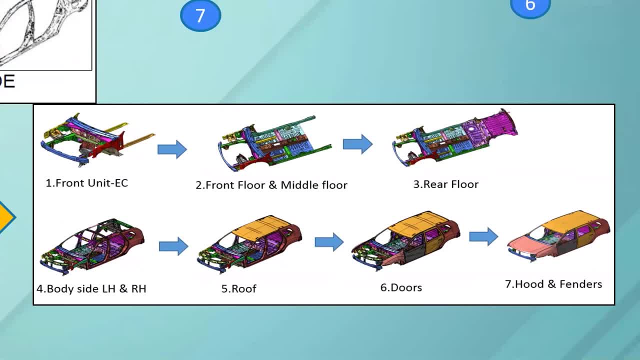 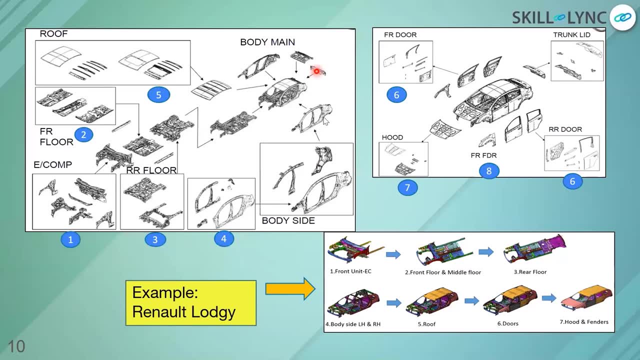 occurs in this progress. So any doubt in this two assembly sequence anyone. I will explain you about the welding process in upcoming slides, maybe tomorrow, not today. yes, I will explain you about hemming also. Anyone have any question related to this two assembly area? clear, all clear, okay, great. 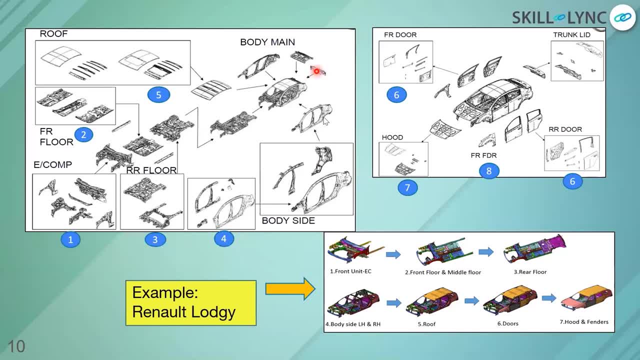 great. So chassis fitted in TNC chassis- okay, chassis you mean the engine and complete engine suspension axle all together will be fitted in TNC. yes, first one is engine Fuel tank comes in this zone, okay, in the rear floor. as I have explained in the this: 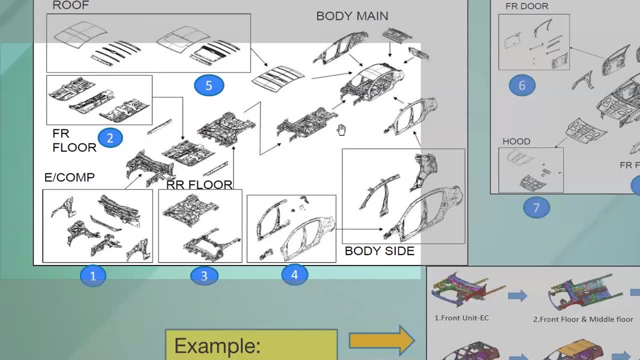 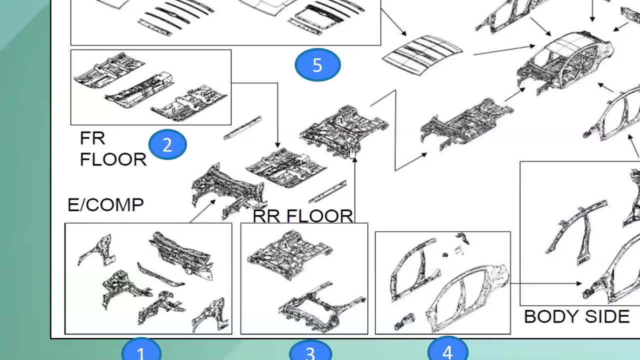 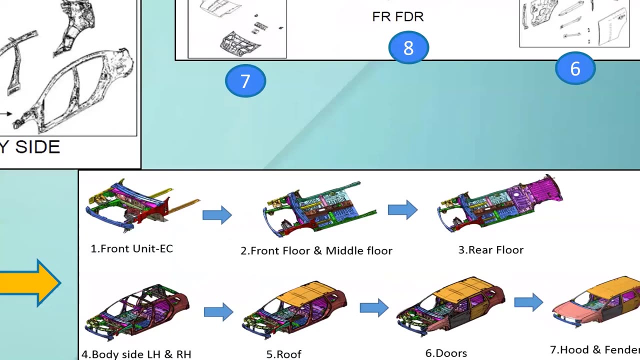 this zone of the vehicle is where the fuel tank has been bolted. okay, here under, under the front of this area. okay, I can explain in here also, in this zone. okay, this outlet which you see a small hole in here, that is for the fuel pump. okay, so that you can. 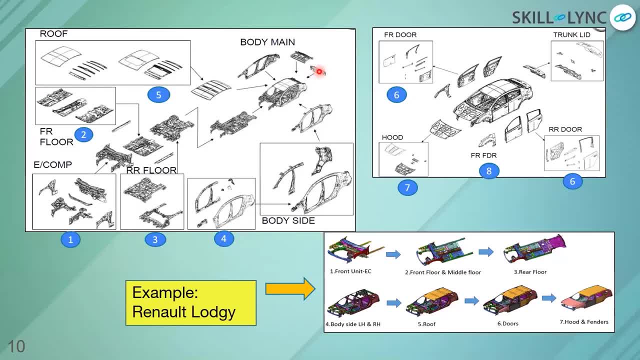 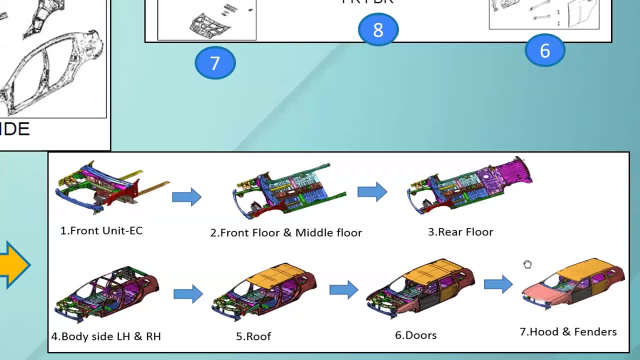 like service your fuel pump, if there is any issue. no, BIW contains all the seat metal parts. before painting This, this is all BIW, Okay. Okay, That is BIW components till here, okay, and this has been like painted and then sometimes. 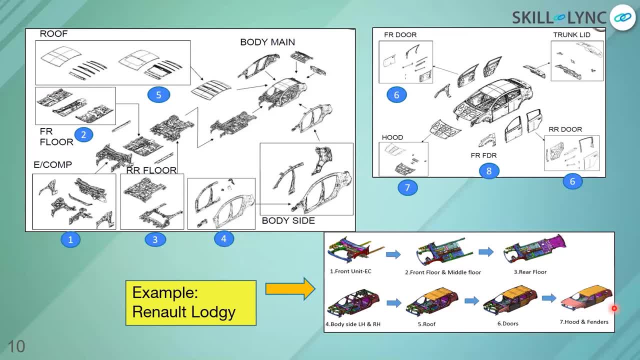 it. it is getting dismantled. all the doors will be getting dismantled and they have to fit a lot of things inside the door. so after they paint and dismantle it and then TNC, they will assemble it again. okay, software, we use a lot of software. Enex like depends. 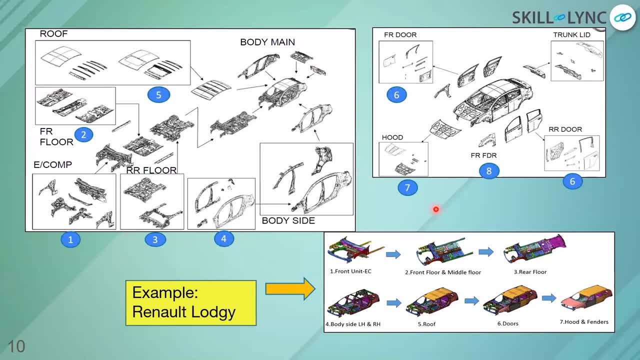 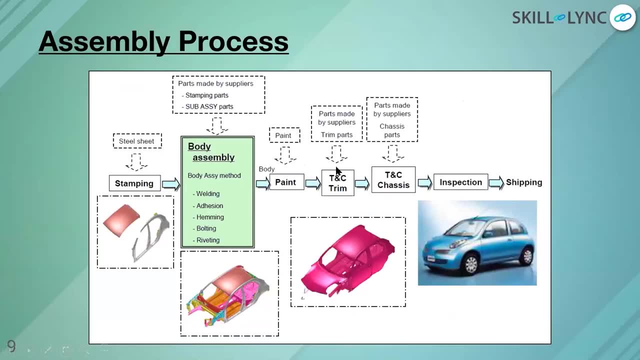 on company. what company is using? some company use Enex, some company- you know how they company- use Katia. some company use solid work. so it depends on company. so this is all about all about assembly process. so I will show you some of the videos related to part and manufacturing. 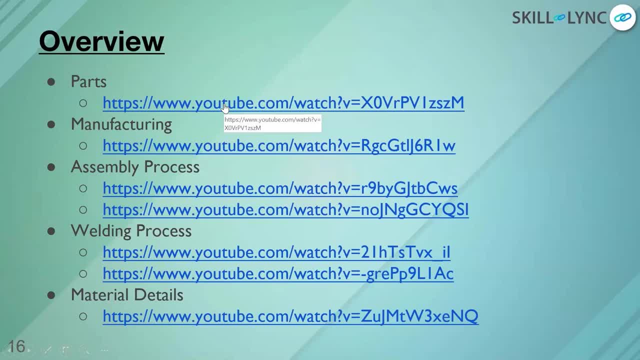 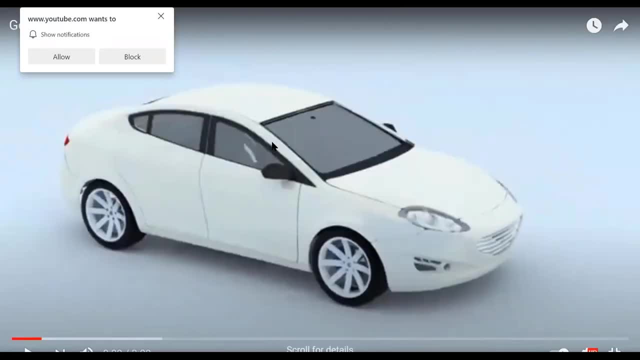 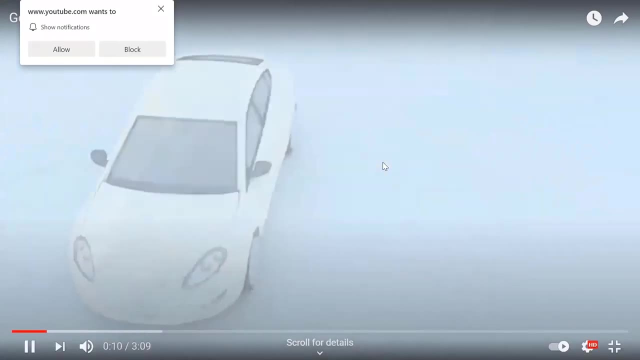 and assembly process and then rest of the things we will be discussing on tomorrow. maybe, okay, you can see my screen, guys, can someone confirm? okay, you can see the video running YouTube? okay, great, so, uh, so, if you can see, this is a complete car, as I have explained you. these are all the classes. 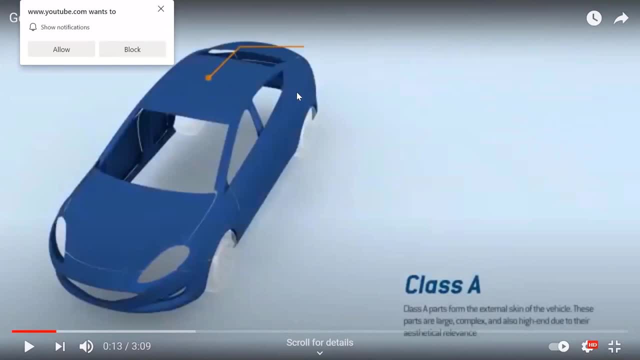 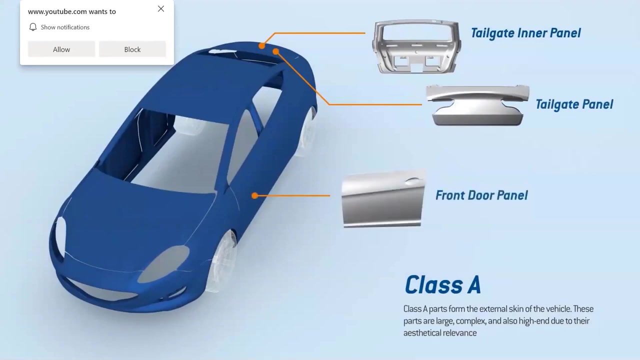 surfaces. uh, in the area which is been given by a styling team to us from which we extract the complete car: okay, roof panel, body side panel, fender panel, food panel, food inner panel and the other areas: okay, tailgate, tailgate panel. front door panel: okay, front door inner panel is also. 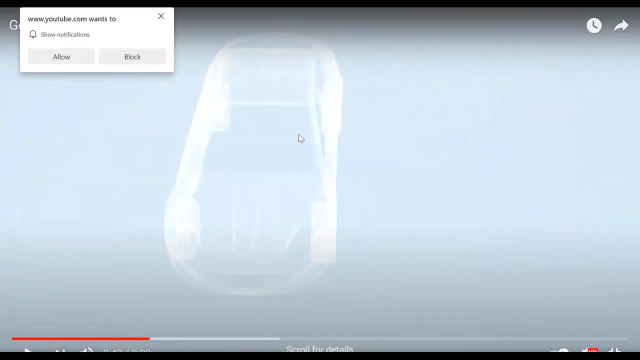 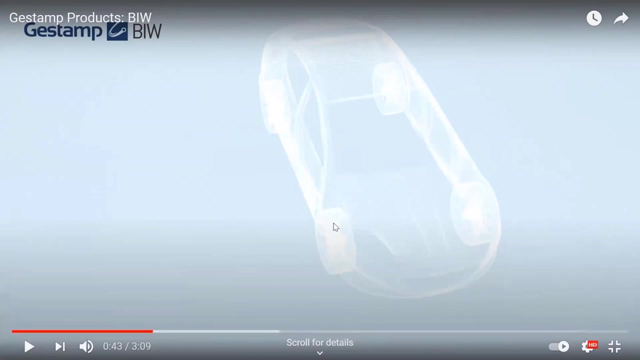 there. okay, can you hear any music? no right, hello. I, I think I don't have access to music. I, I can't play the music. how, how can I help? I, I don't know, but uh, when I'm playing before it have a sound, but now I can't uh get the sound. I don't. 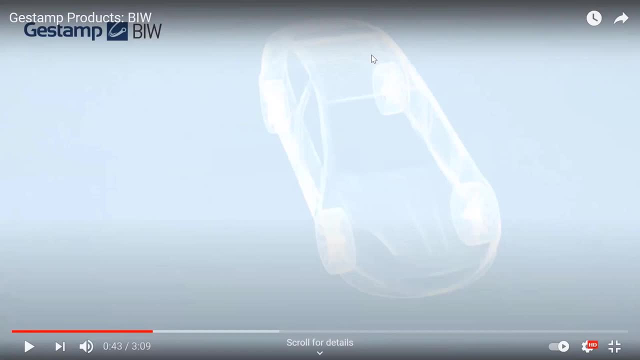 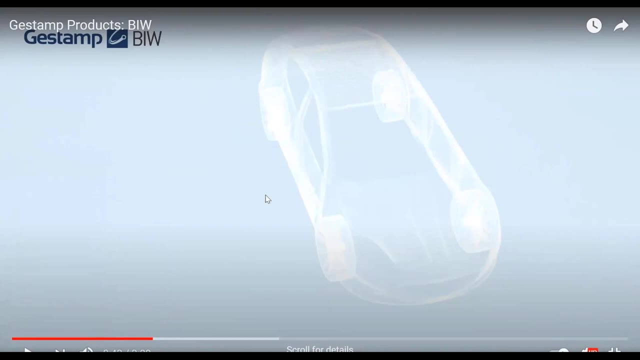 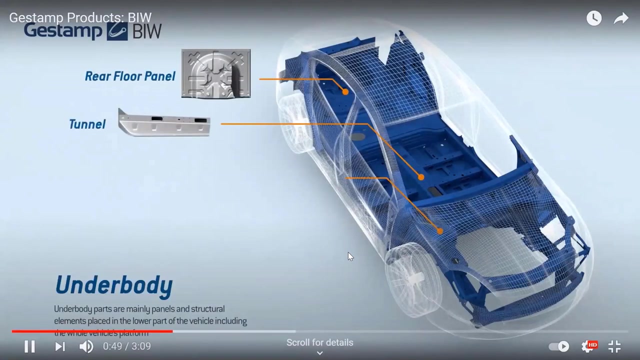 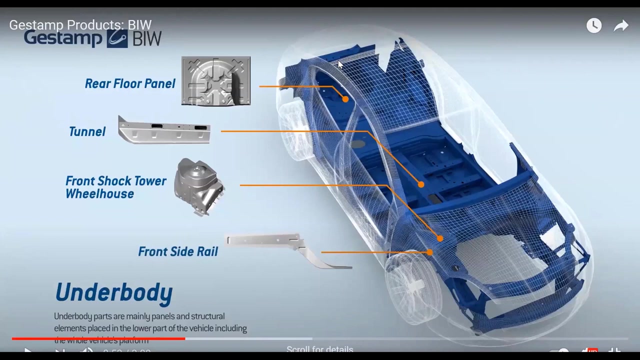 think you can share uh sound from your screen onto my not sharing. oh, okay, okay, yes, yes, share sound option is there. yeah, thank you, thank you, sure, now people. uh, okay, leave it then. uh, I think there are some audio issue. I have to deal with my uh mics and 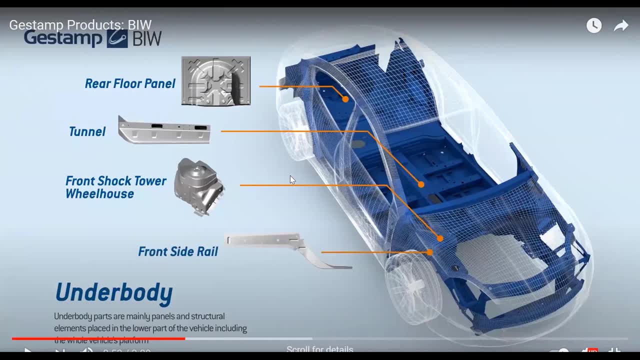 all, okay, there is no such Informatics sound in here, it's just a music to entertain you guys, okay, so again. so, these are the areas, like, as I have explained you, so you can go through with this video also, which will say: uh, this is again where the spire will be, will be there. these are the Shock Tower, uh, front. 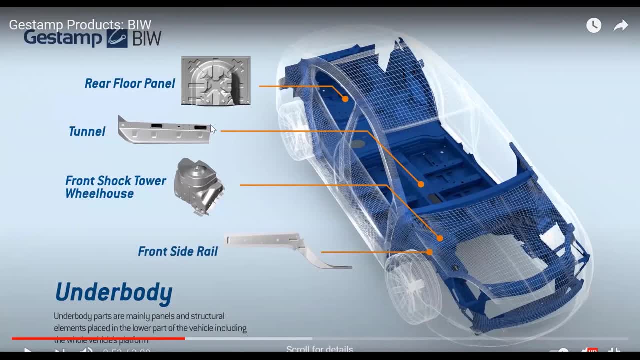 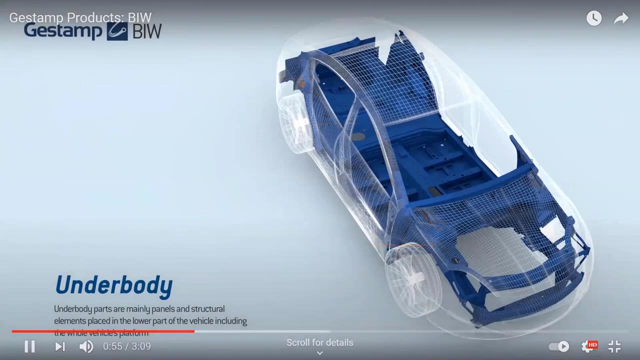 side rails, okay, which absorb all the load and transfer it to back outside of the vehicle Tunnel, which allows uh, which takes the load from the uh, and the same time, it have an envelope for our exhaust passing and the drive sub passing. okay, so this is all the components. uh, it's a. 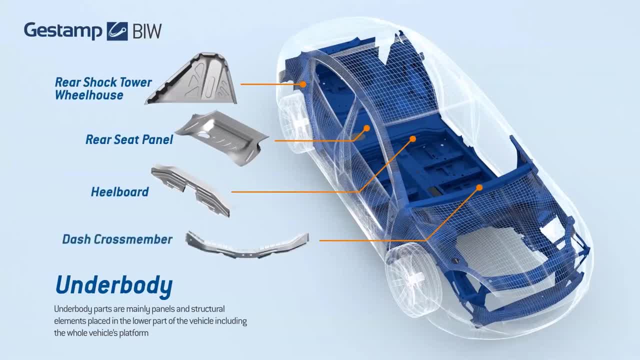 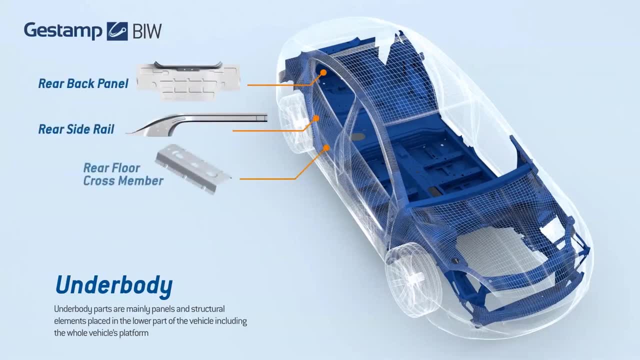 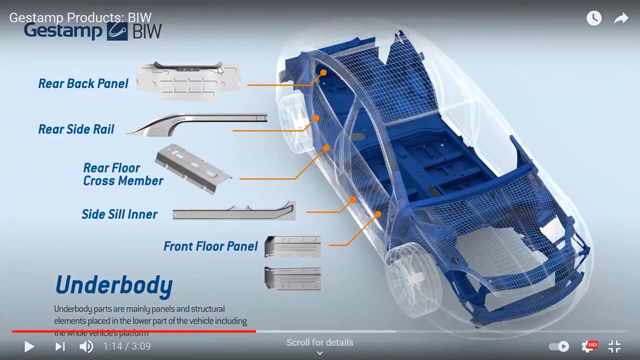 rear Shock Tower, rear Sheep panel: okay, heel board or the kickoff wall wall. what we have explained. dash crossmember is for the dash reinforcement, okay. rear back panel is for the sedan cars. most of the time we have it. we don't have it for our hatchback and this one, okay. so 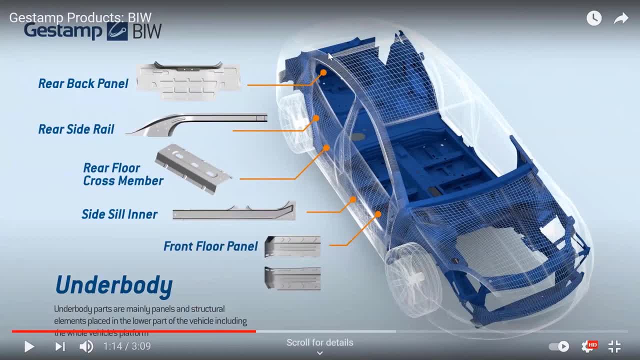 this rear back panel. we have it for apron also. okay, and in the sedan car, if you behind the seat, we have one panel area also that is also be said as rear back panel. okay, so this is all about the components you you can see inside the car. okay, this is upper body. okay, b pillar, b pillar inner. 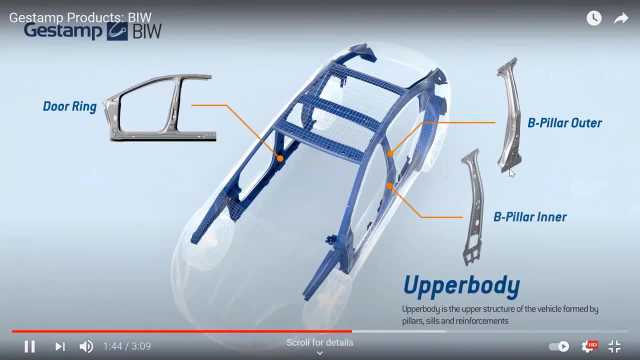 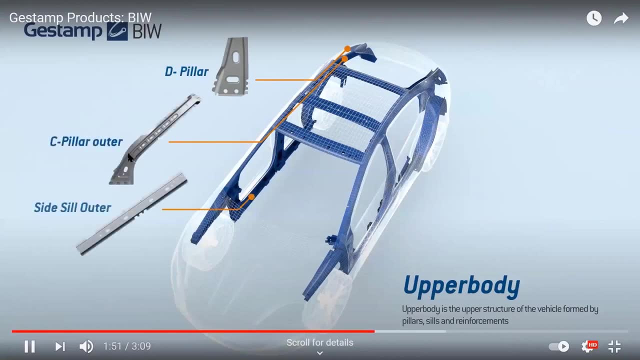 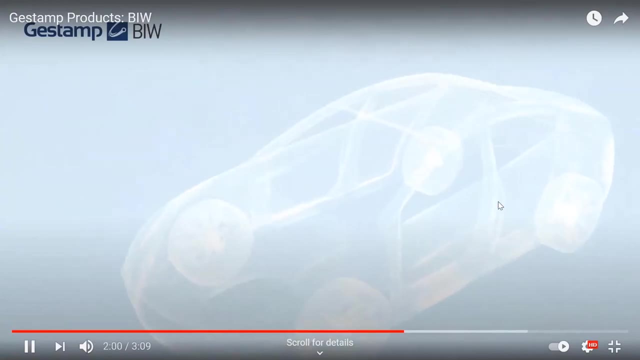 b pillar is again i have, as i have explained you it has been also used. we cut the part and we use in for two variants: d pillar, how it has been used. c pillar, outer side sin, that is for the side crash things and all okay closers. these are the complete range for inside enforcement is a window frame at the same. 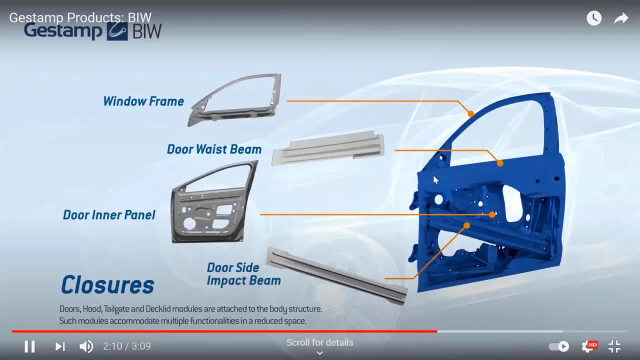 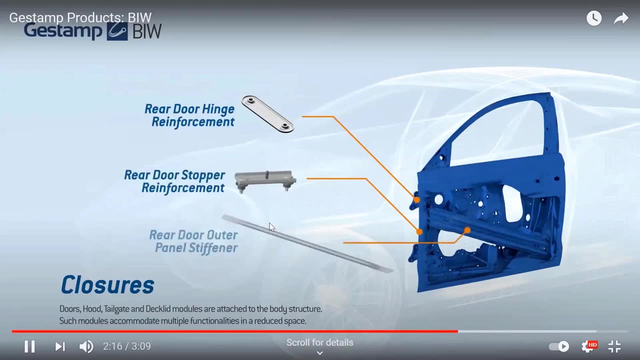 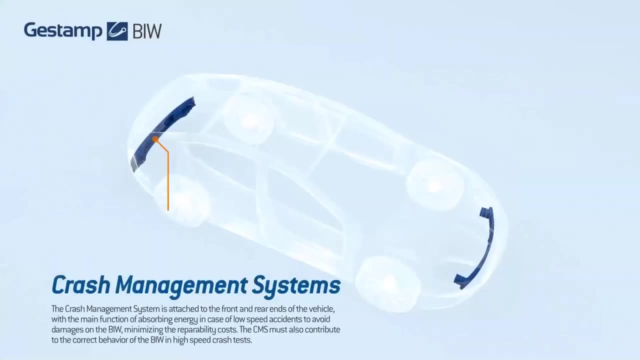 time sash frame. also, door waste beam is used to send the energy from here to at the back. also okay. anti-infusion: uh, it's for the side crash. we use this part. okay, crash management system: uh, this rear bumper and front beeper have been used for some heavy. 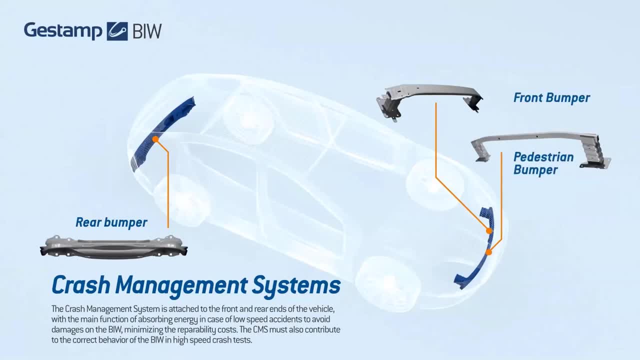 related: crash, okay, or pedestrian bumper: uh. some country have some strict regulation, suppose? uh, europe and us uh have a r-car related uh concerns. so for our car, if the car is hitting with the speed of 10 km ph, none of the areas should be affected, unlike only this part should get affected. okay, for that we use this uh bumpers in the front and the. 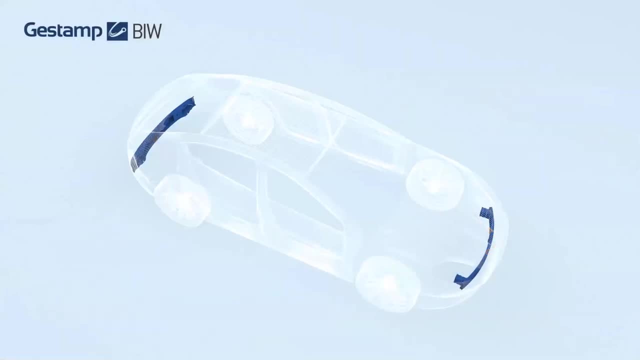 rear. these are the steel bumpers which comes the after the plastic bumper, and that's what is 퉵یم dej me hmmzin rea cuzそう días в porsche. in the front and the rear. these are the steel bumpers which comes be after the plastic bumper, and part, except for main vehicles, okay, for that we use these bumpers in the front and the rea this after the hoffe ng bumper, and that's why your fool will fuck, получить null without having ani. 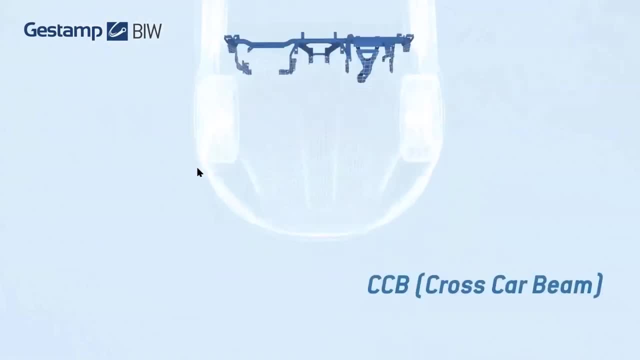 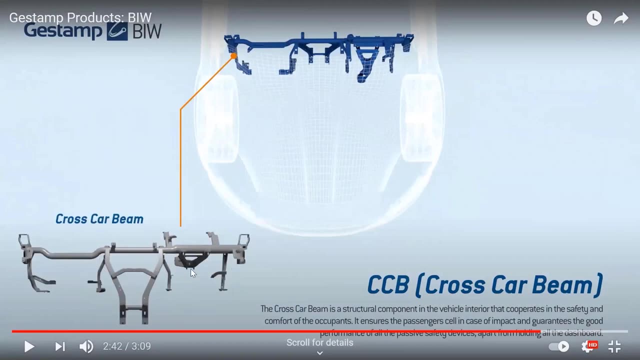 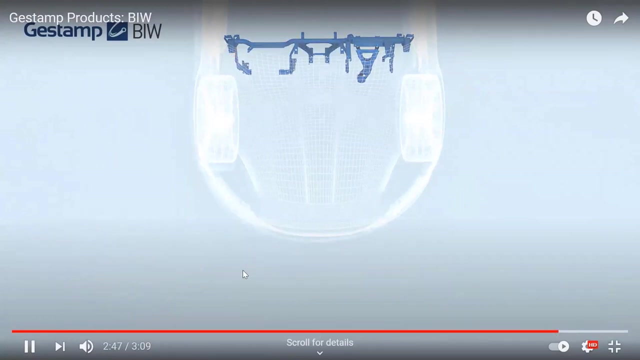 the absorbers inside the car. this is the cross car beam, which holds everything, like the steering, the pedals, ac, air conditioning areas, everything of the car is been like in the dashboard. everything, whatever you see, is been assembled in this cross car beam. okay, but that is not a battery boxes. 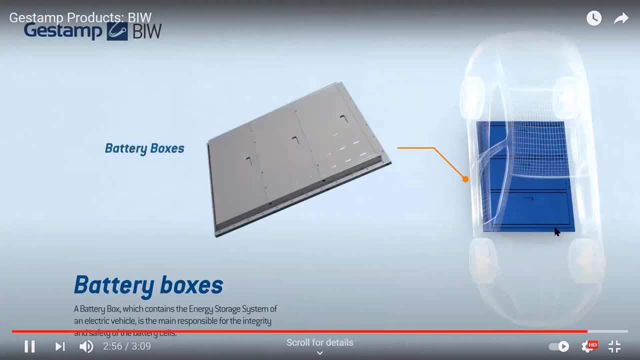 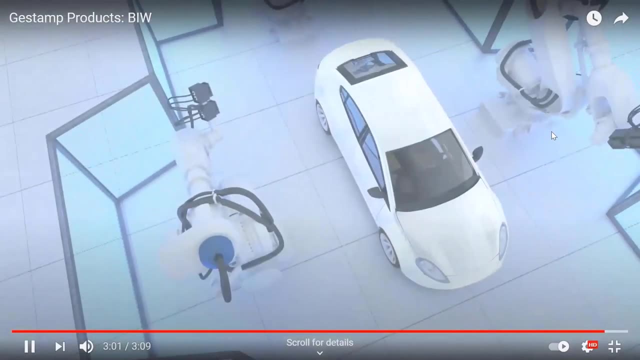 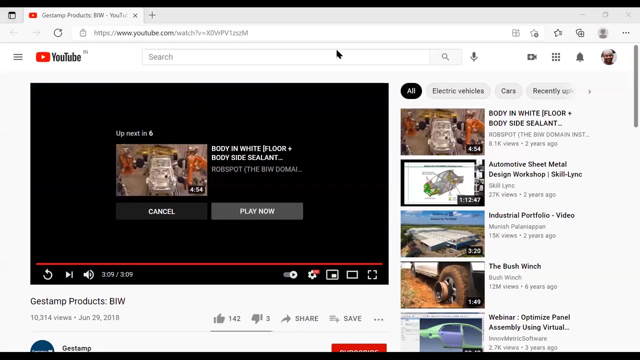 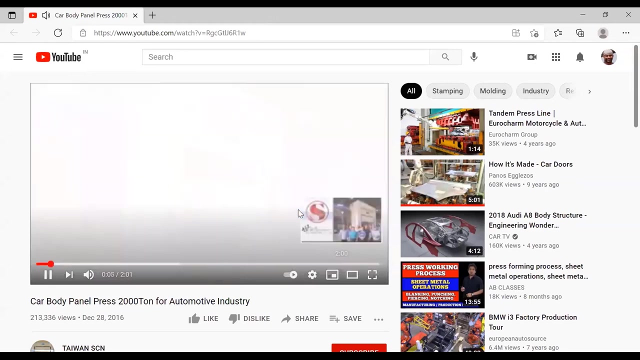 is in this underbody central area, below the car unit, below the underbody unit, the sheet unit. okay, so we used to produce. this is how the printing process is been done. okay, this is all about the parts. okay, the manufacturing process is this: inside the car for the part components. okay, 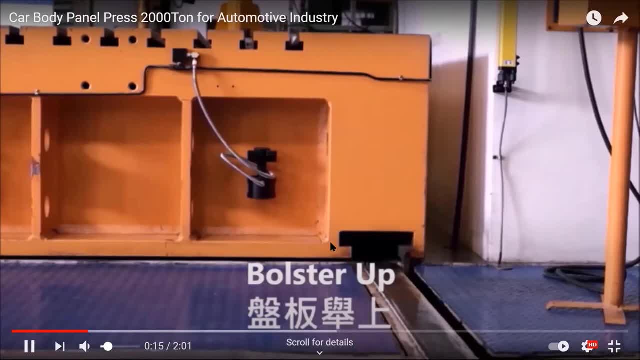 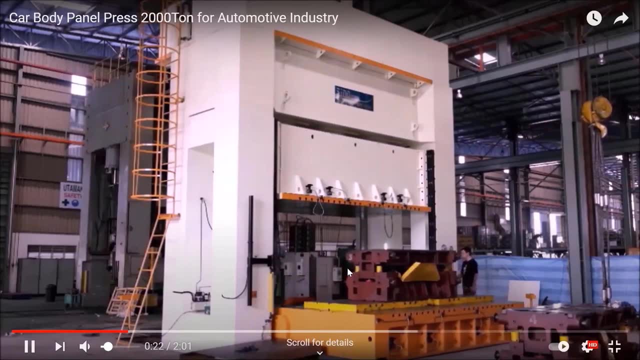 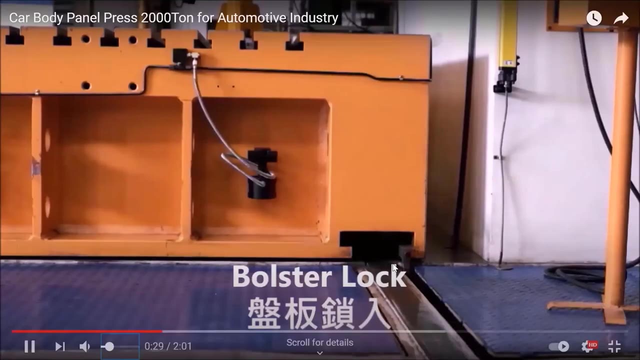 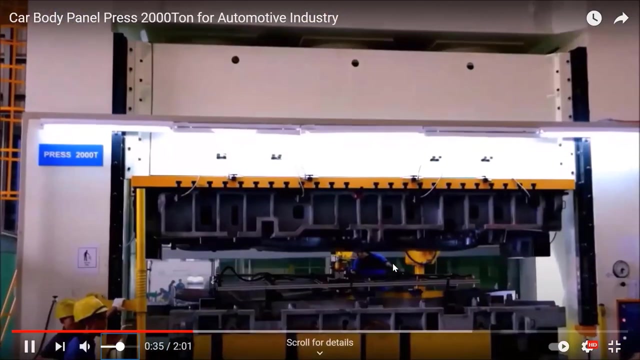 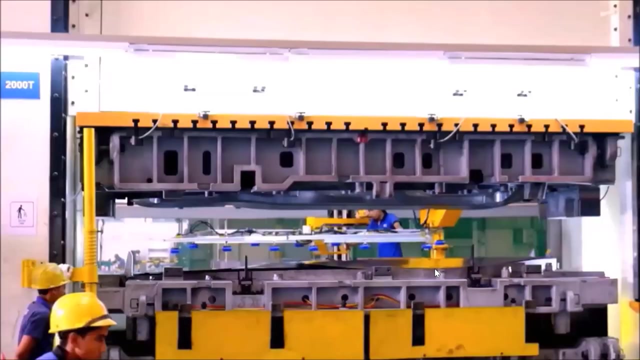 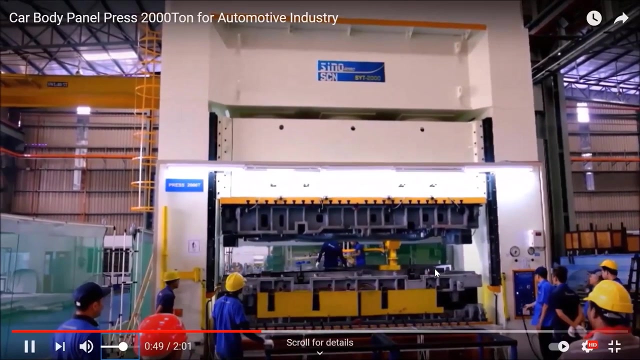 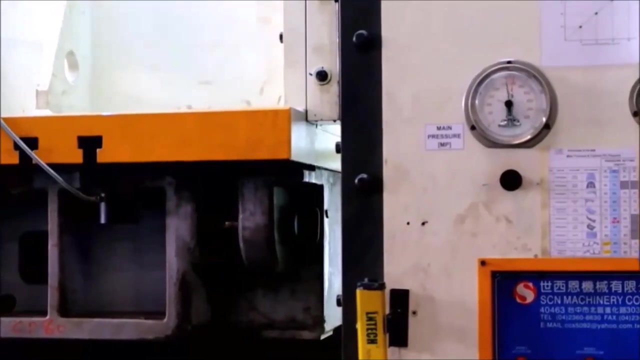 so this is the tool, the punch and die, which we use in the industry. okay, to make a component. inside this we'll put a small, small uh sheets and we'll get our form component. okay, they have loaded the sheet metal inside this sheet. okay, the die is pretend to cheddar. 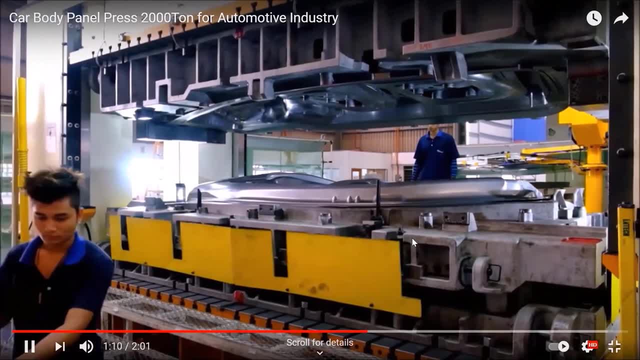 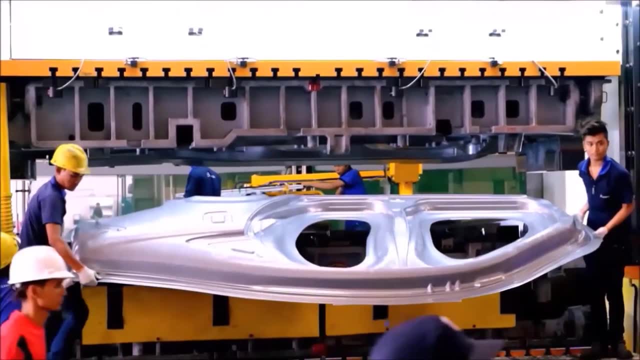 okay, loads were acting as they build on the component. the first strike because my PSOisses also the car and this died okay, but this is the die how it is been working. The load is acting on the component. that is what i was telling you兩 time. the Title of the car and i was telling you guys about this yak of the PSO. this đang ska song to tell you how its looking. okay, every timeYou should see how the PSO looks. so the first strike has the car back and then feels t the spoiler. its going to flood the entire car. so mobile car needs to come in the back of the car to start the PSO6 and auto start the car. so there is a Ek. 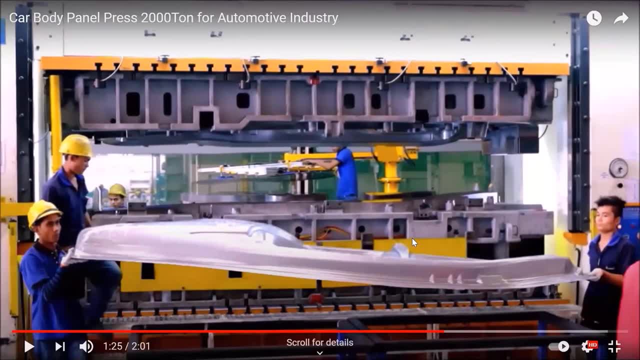 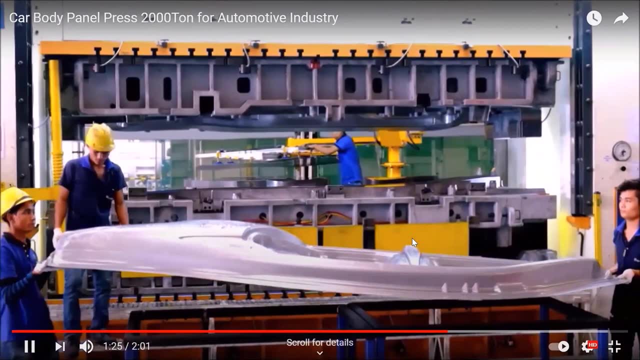 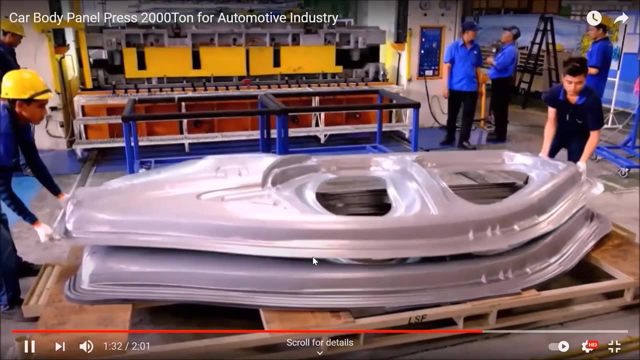 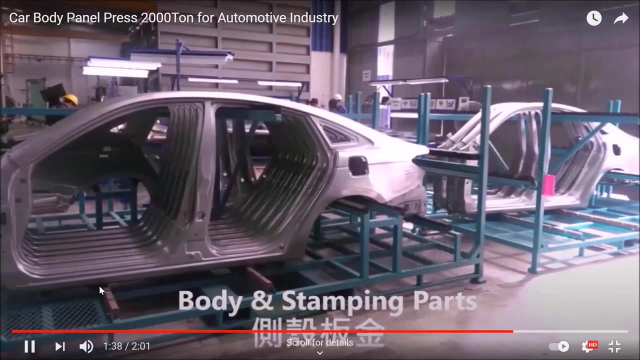 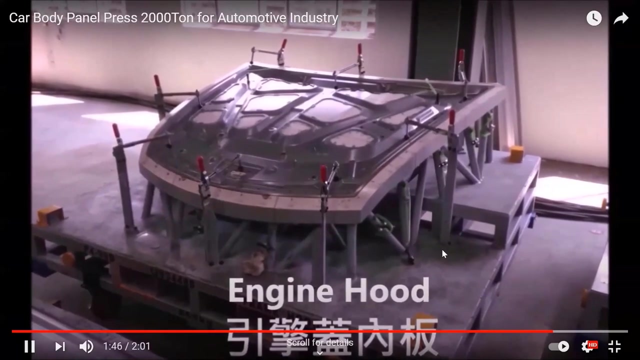 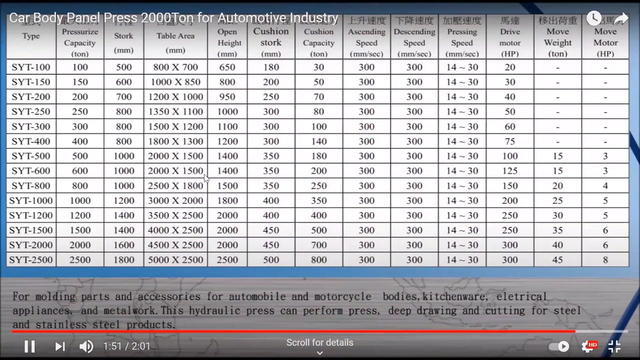 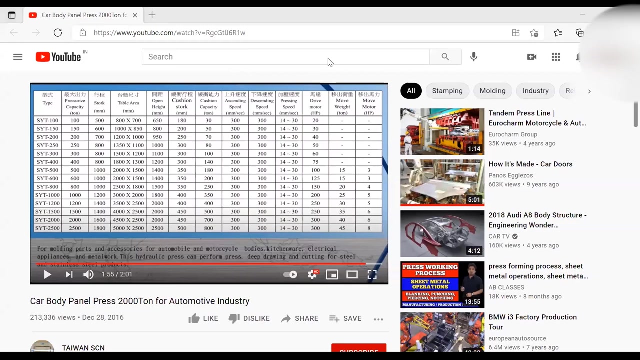 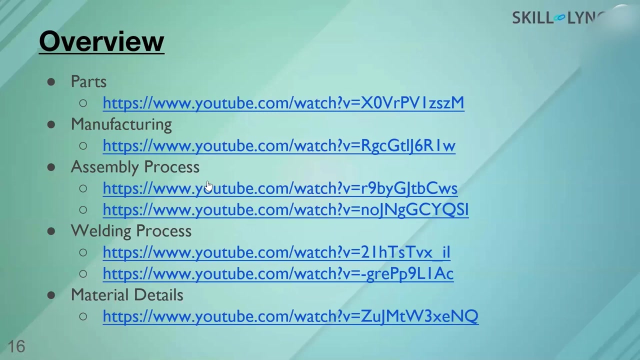 bso we generally have two strikes once: first strike, one the second strike, and then we have piercing operation, then we have trimming. so this is all related to the manufacturing, how it has been done in automotive and this is the assembly process. video. good grammar and spelling are important, but if you want to write essays that inspire, 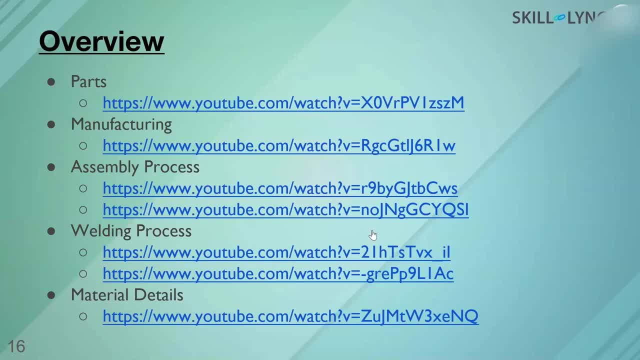 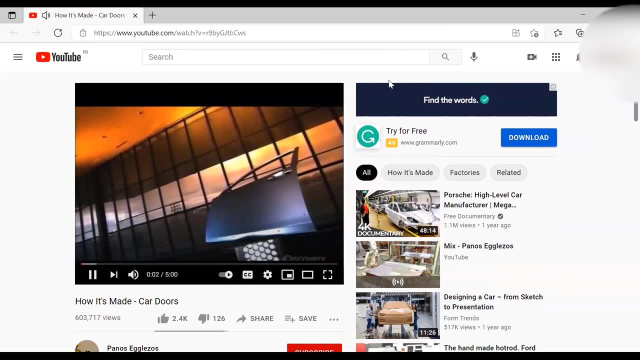 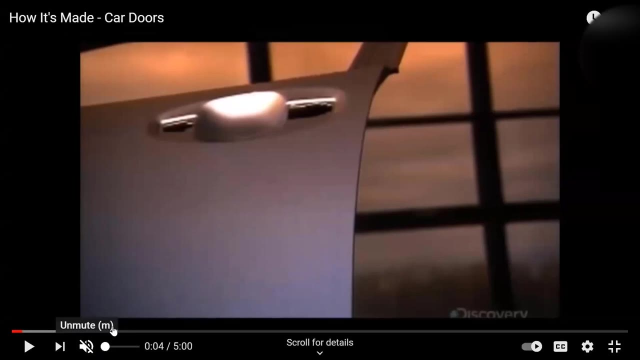 messages that forge brighter connections. car doors have come a long way over the last century. so you guys can see this car door video, uh, how the manufacturing has been done. i'll mute the video, okay, i will mute the video okay. so, guys, can you see my video of the car door how it's made? cardo. 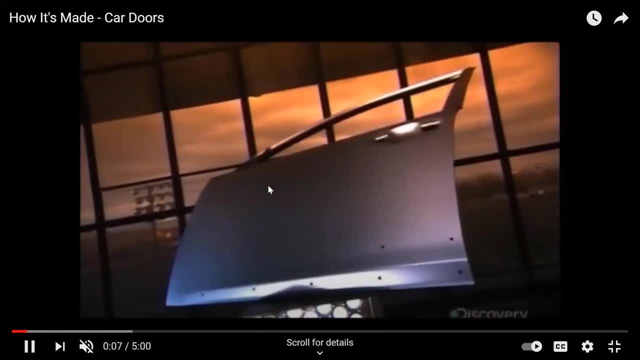 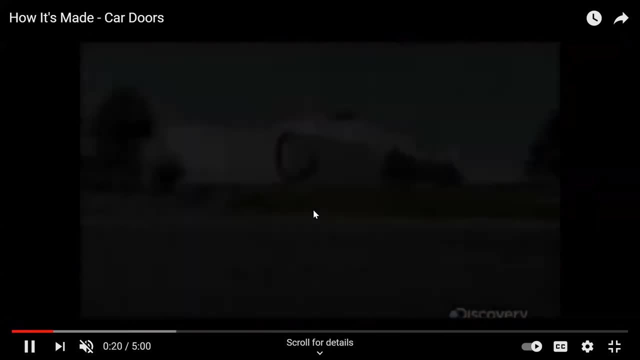 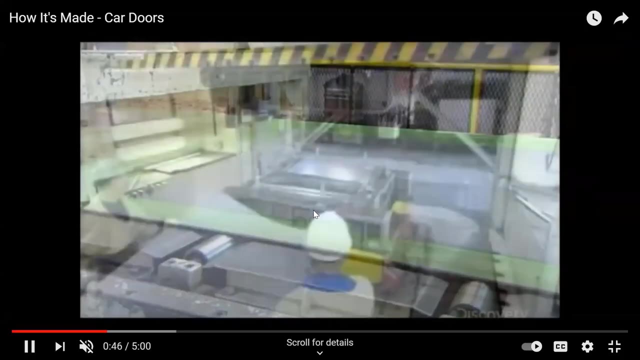 okay, great, okay, so you can see this. uh, i have just kept one ppt, uh, one video for this, how it has been made. okay, the car door. so, uh, it's from the rolled sheet, it is, it is it has been cut and as a component, and see how it has been kept inside the tool. and this is the car door. 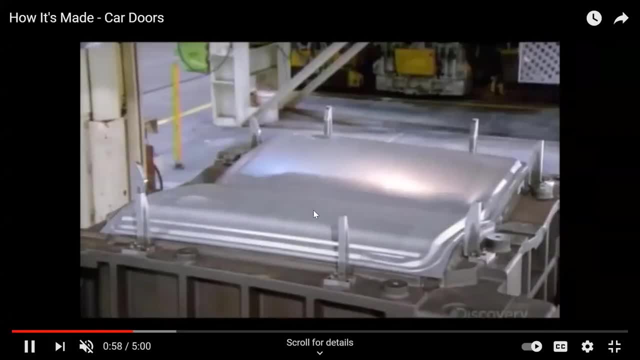 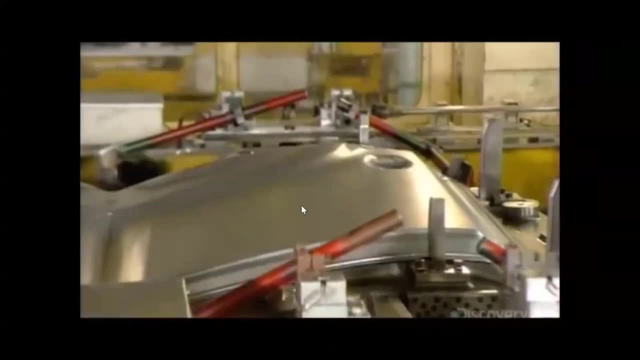 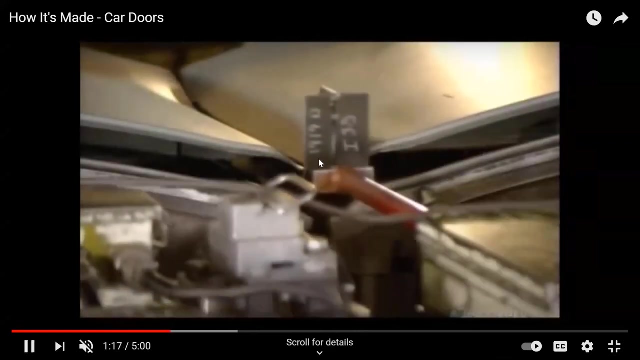 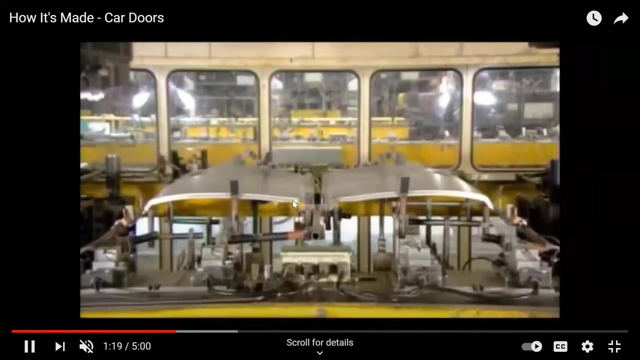 is how it will be formed. okay, so this is the first draw. it has been made. okay, you can see. okay, now two, two lh and rh has been divided into and it's been cut. uh, they have separated it with the trim operation and now they have all the forming, uh piercing operation. they will be 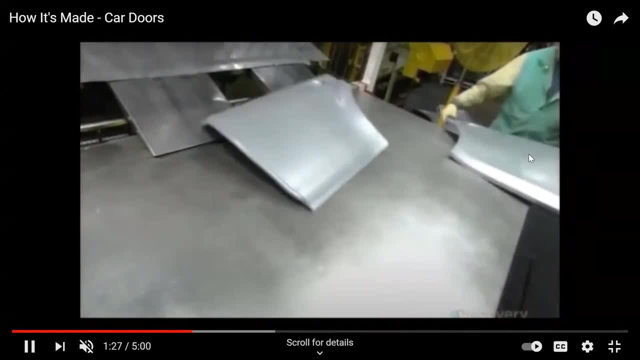 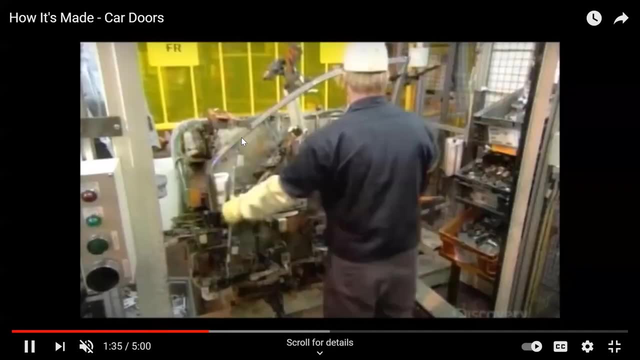 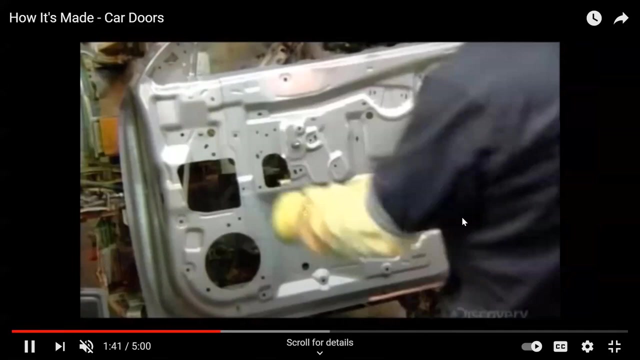 performing in this. okay, so we have now both doors- lh and rh doors. so the quality inspector is inspecting all the roughness and all they will say. so this is how they will do. this is the window frame, the top frame. this is the front reinforcement where the hinge in all will be fitted. this is the rear- uh, in a panel of the door assembly. 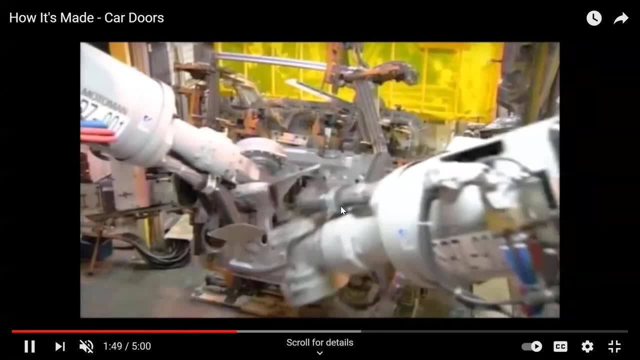 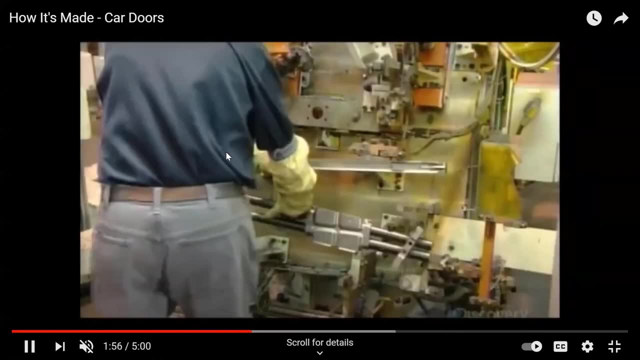 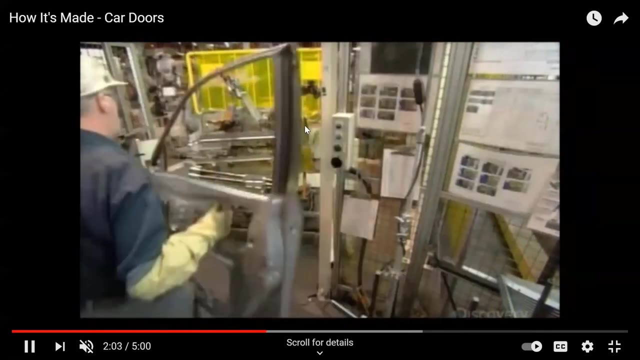 okay, and this is how they are building it. this is a spot robotic welding process. we had, uh, we even have a, like uh, manual process of welding. also, this is an anti-intuition beam and this is the upper west. okay, that is used to transfer the load from front to the end of the car. 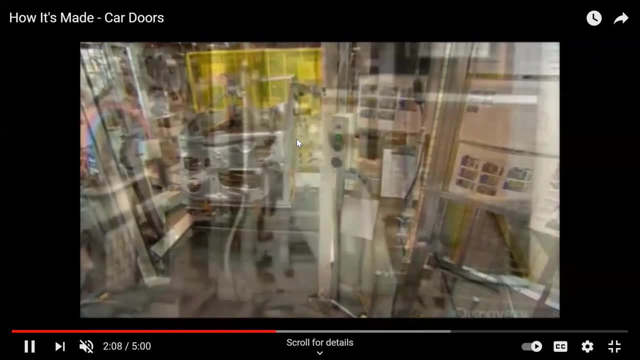 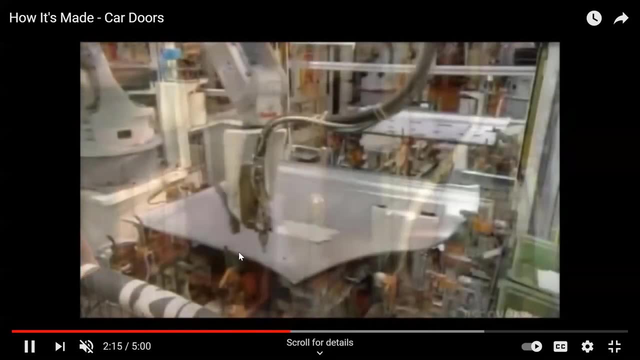 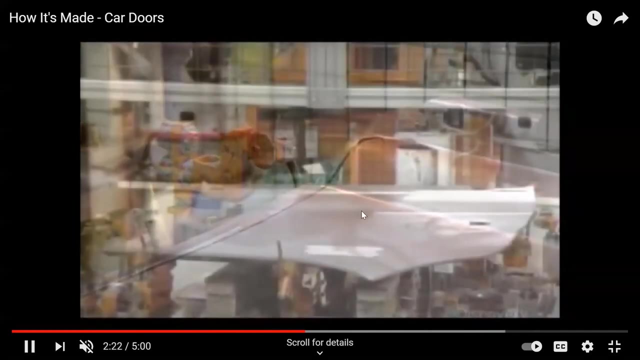 okay, and then they will put this again. it's a robotic welding. this is how the uh arc, this spot welding, they are doing for the components. okay, this is the mastic provision, adhesive provision, how they are providing. okay, for hemming operation. now the outer panel of the door. 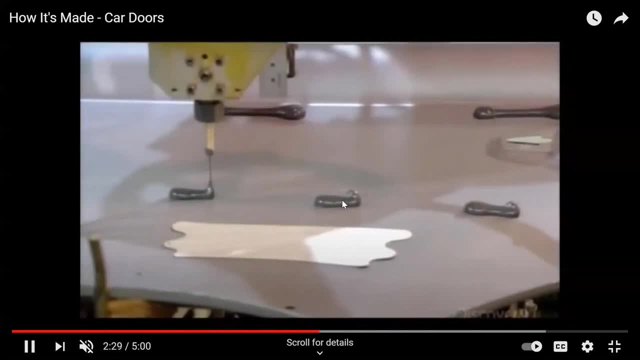 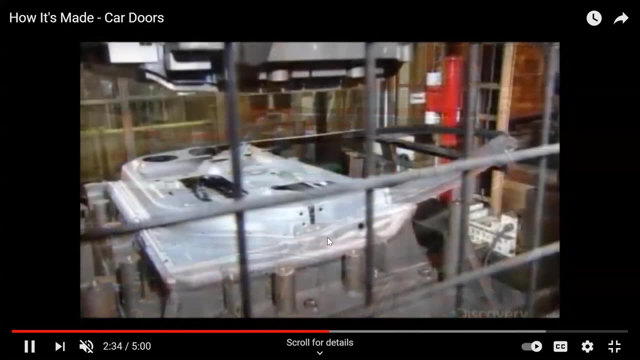 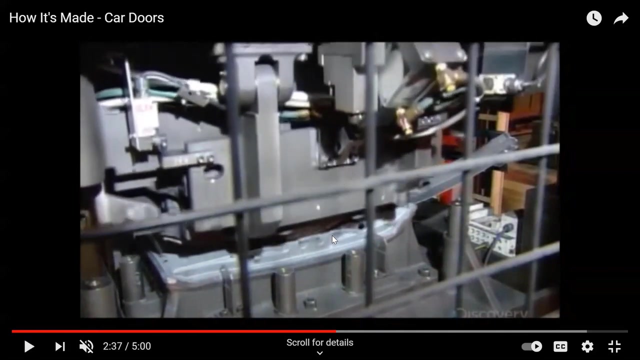 and the inner panel of the door. it is not been getting welded. it has been attached together adhesive. why it is not getting welded? because after the weld it always leaves a mark, okay, which is not acceptable by customer. uh by visible. they should not see any welding marks on this kind of a surfaces. so that that's the only reason we used to uh do adhesive. 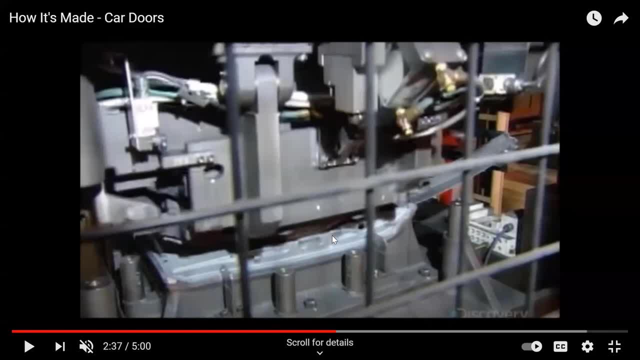 uh, we used to provide adhesive okay in this areas because, uh, and even though adhesive is an expensive process, but even though adhesive is an expensive process, but even though adhesive is an expensive process, but all because it have a visionary impact, uh, in the car, uh, and the customer directly can see it. 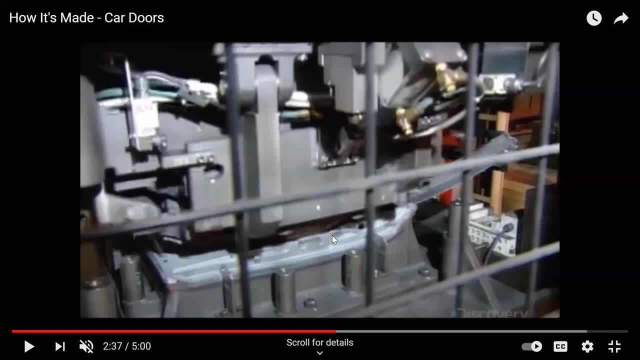 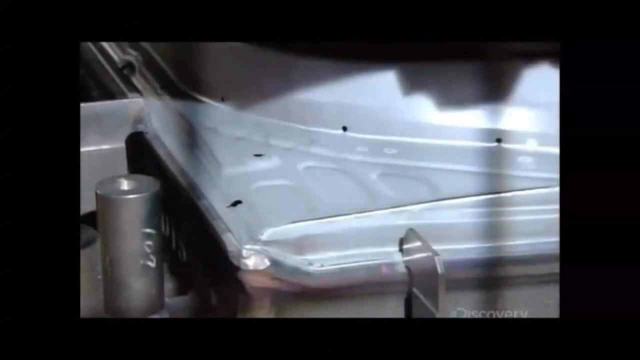 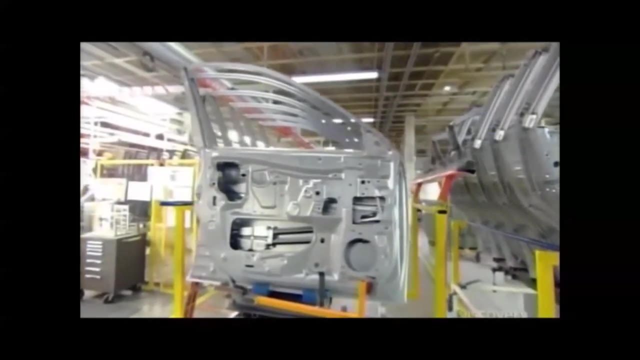 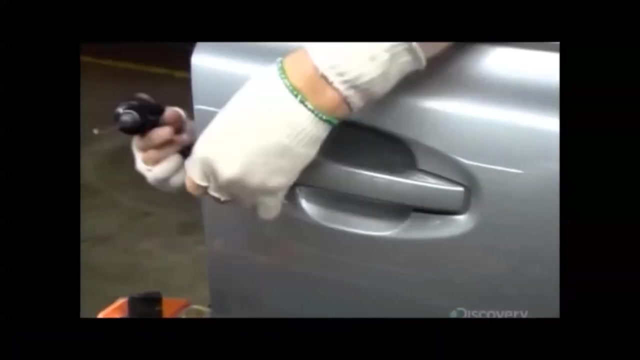 okay, we used to uh provide, uh, this kind of adhesives in the car, okay, okay, so you can see, this is how the assembly for all the biw component is is been done in the door, uh, door panel. and this is how the tsa in tnc of doors, how everything has been fitted. okay, so this is how the handlebar has been fitted. 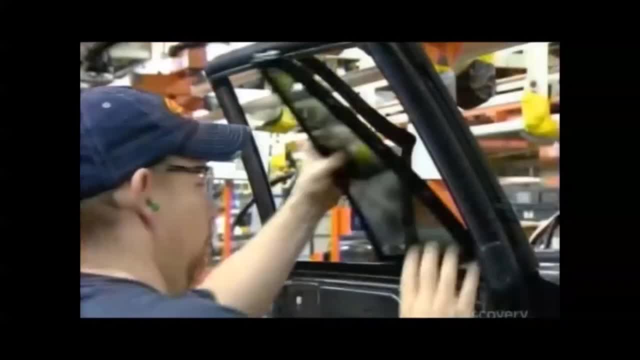 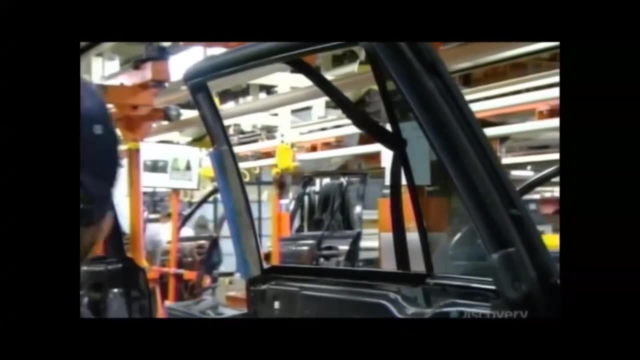 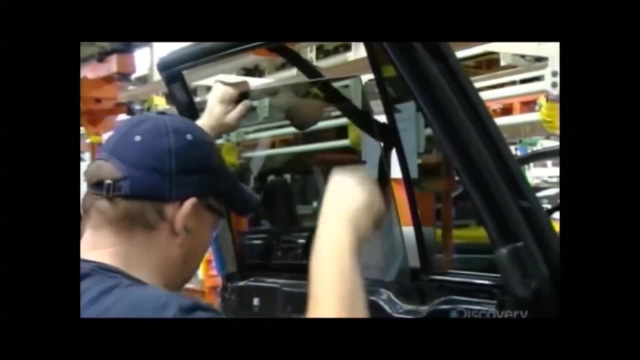 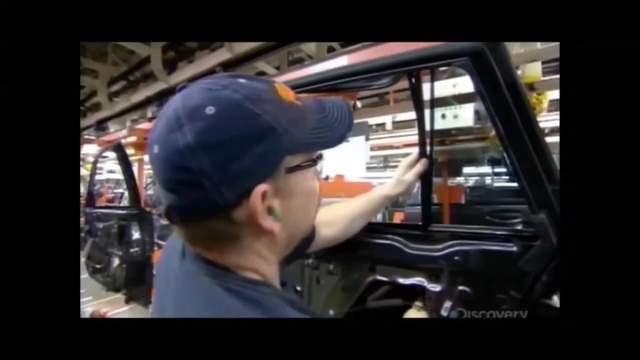 this is the chrome uh fittings. uh, at the top, this is how the windows are being fitted. okay, so you will see on the inner plastic- ip and all other things- glasses- how it is all been fitted together. you can see it in this video. okay, this is the rail: uh rail for the windows to move. uh, this will be moving in this way only. 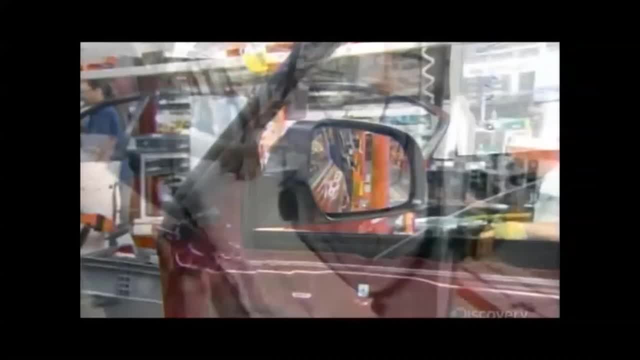 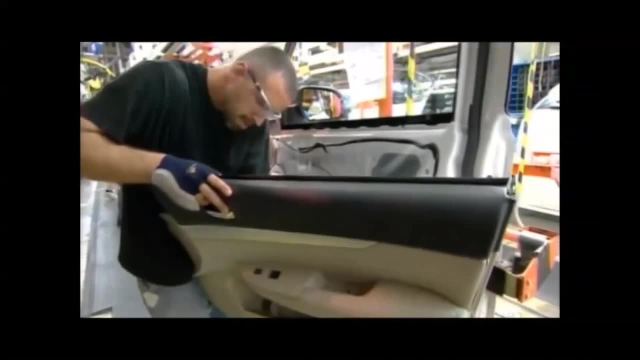 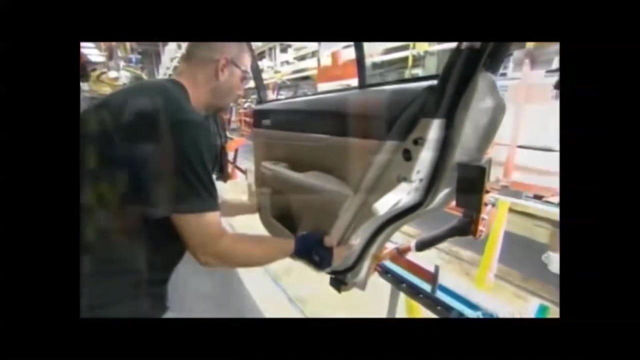 this is a side mirror. a side mirror sometimes be fitted in the body. okay, this is the complete ip mixed with the soft and hard plastic. again, it's a different area and how they are testing the functionality of the windows and all. and this is how the door smd has been completed. okay, 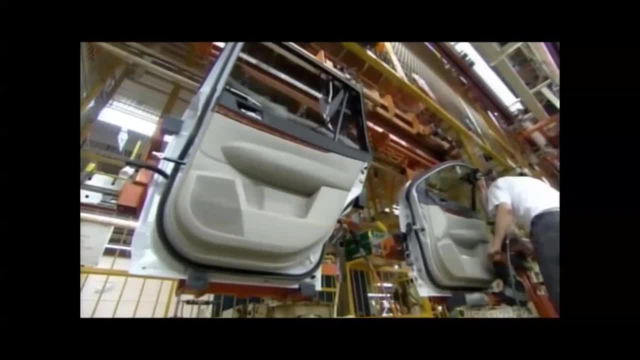 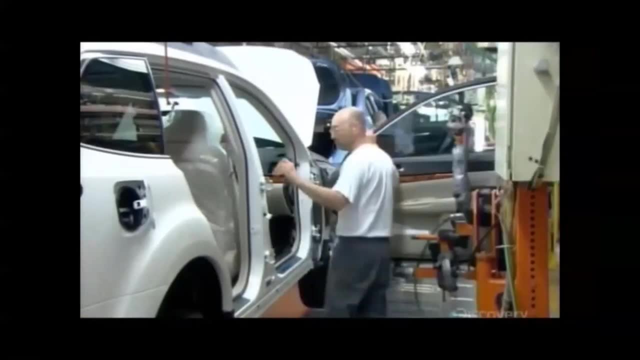 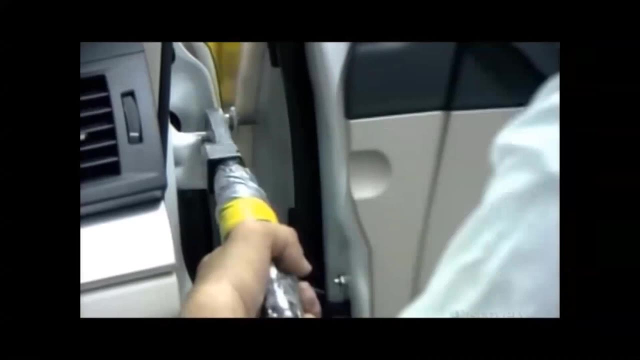 and the door assembly is also getting uh fitted in tnc uh of the car. okay, after the pin, the door assembly comes out of the car and after this all the seat and all the dashboards, everything has been fitted. they assemble these doors in the car clear. 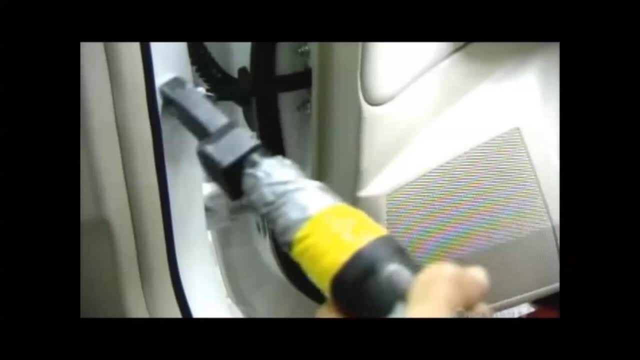 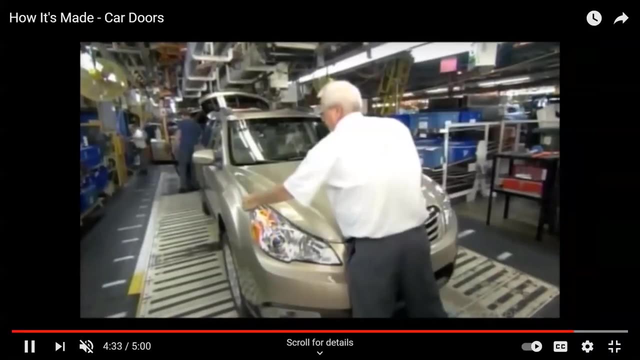 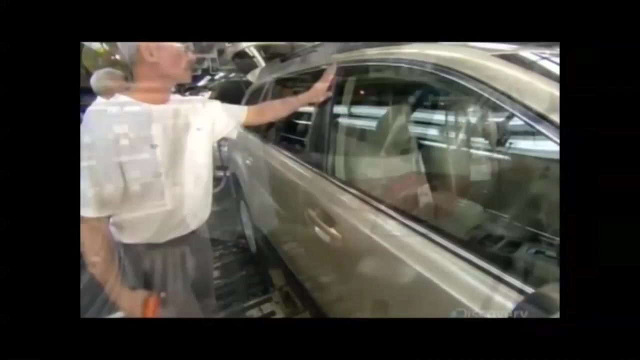 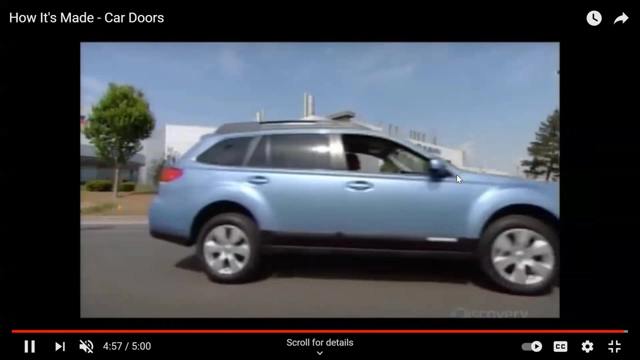 so this is how they do hood and this is their. what they are checking is the gap and flush, so the gap and flush should be all equal. okay, they are checking this. uh, it should not have any impact. okay, so this is the complete tour of how it has been made. okay. 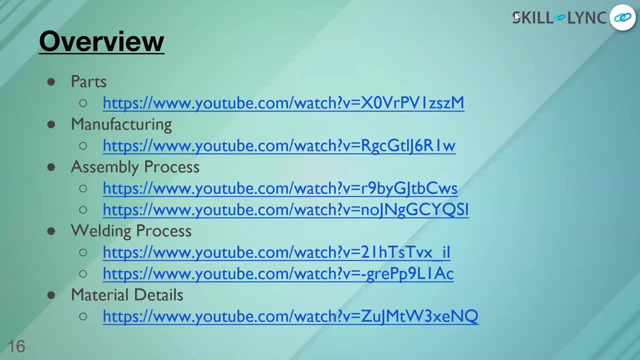 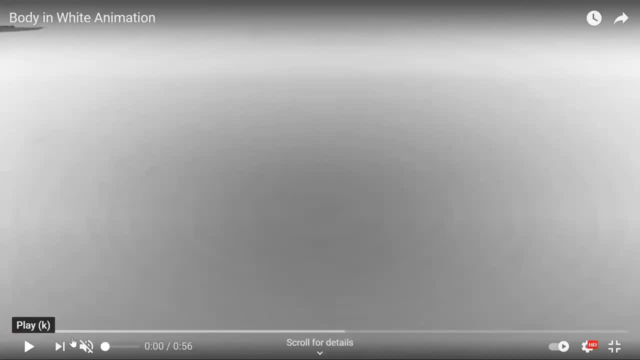 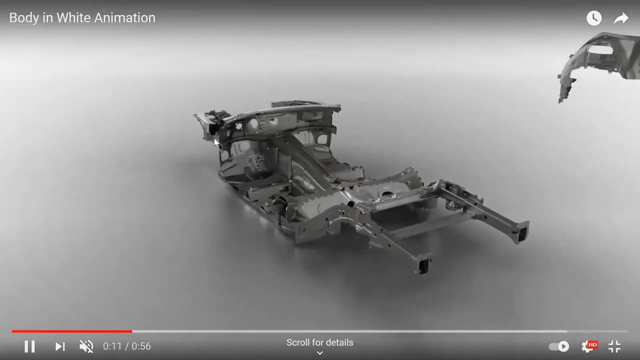 so, uh, one last video i will be playing for today is like animation of body and white smd how it is been done. okay, uh, you can see my screen. uh, okay, yes, okay, so this is how all the component is being assembled. okay, this is only the rear area. this is the front area. this member is only the member which. 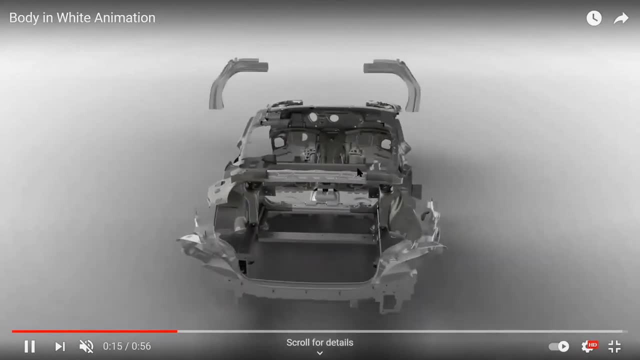 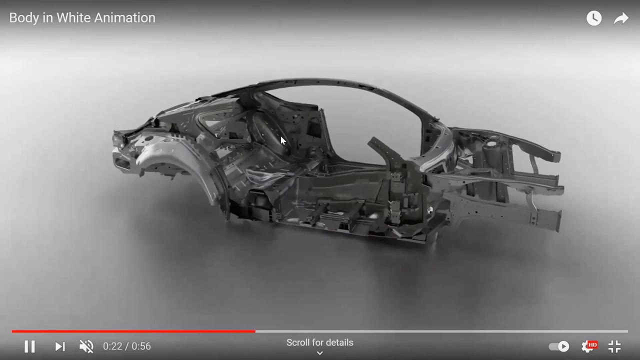 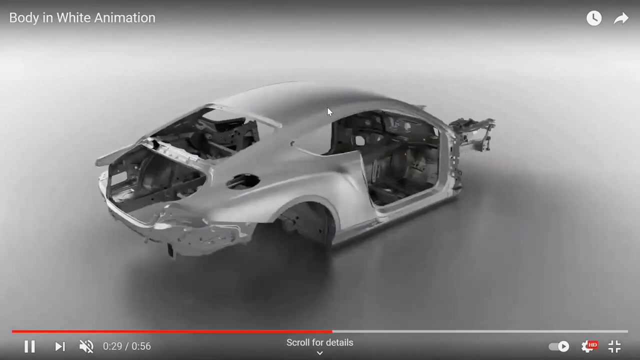 is transferring all the loads. it's for the sedan car. looks like a sedan car. yes, because they have a separate member in here. okay, that is only been used in the sedan car. this is all the components been used in biw, bso, roof members and all. it's a bottom tray kind of things where we 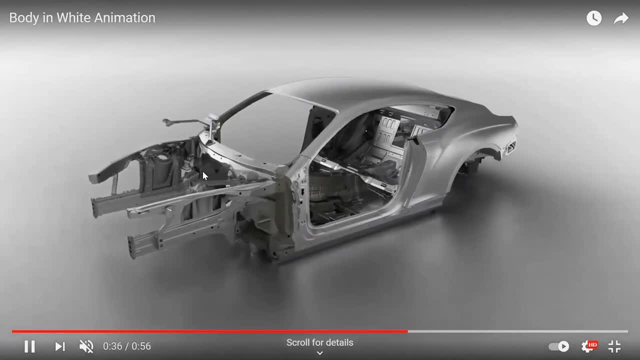 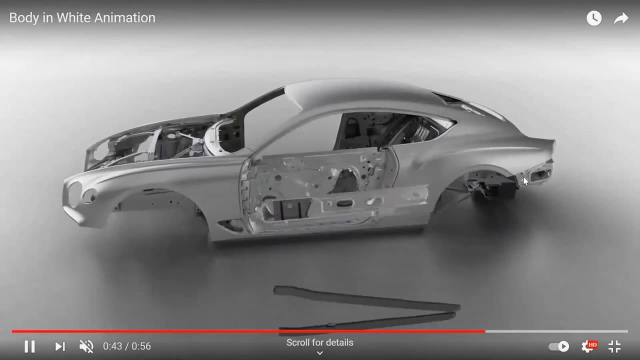 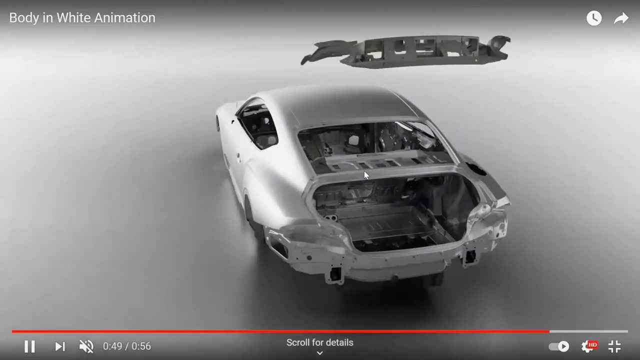 use to keep our spare components and all. so this is a very expensive unit of the car, expensive car. okay, it's something like bentley alpine, so they are using for different, different kind of more members. it's aston martin, sorry. so they are using different, different members. 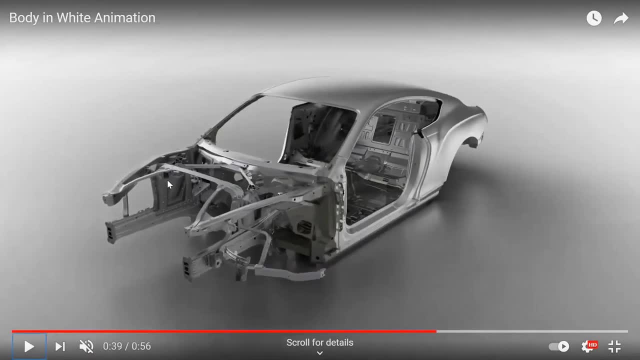 inside the car okay, which is not been used, like some here. okay, this is not. this enhances more torsional stiffness because the vehicle have more dynamics and the higher speed okay, so it should not get deteriorated. that's why they have more stiffener agent in this area. 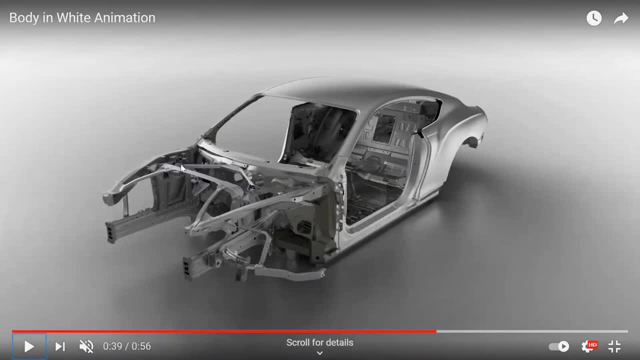 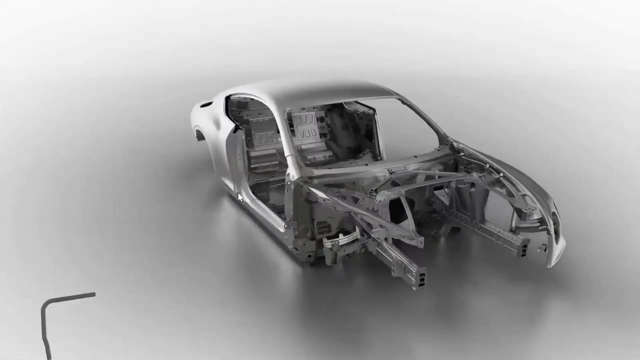 sometimes they use different materials. in these zones they use more yield component, like. sometimes they use magnesium, sometimes they use aluminium, with alloyed casted aluminium also. okay, so all together, they used to make this kind of zones. so that's it for today.